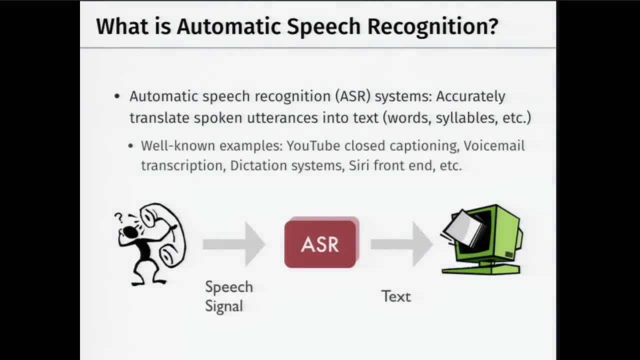 So the voicemail transcription is also an ASR engine which is running Dictation systems were actually one of the older prototypes of ASR ASR systems and I think now it's obviously gotten much better. But I remember Windows used to come pre-packaged with 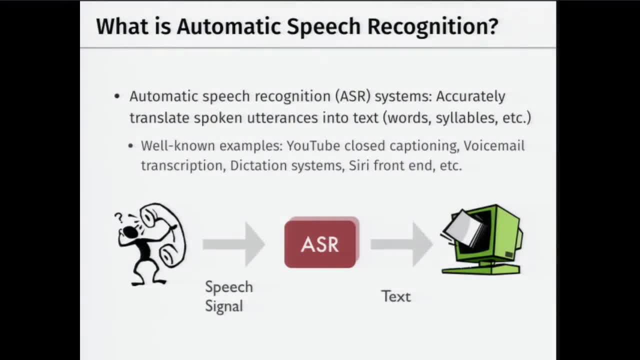 the dictation system, and that used to be pretty good. So, dictation systems, of course you're speaking out and then you automatically get the transcript, the corresponding transcript. So Siri, Cortana, Google Voice Search- all of their front ends are ASR engines and so on. 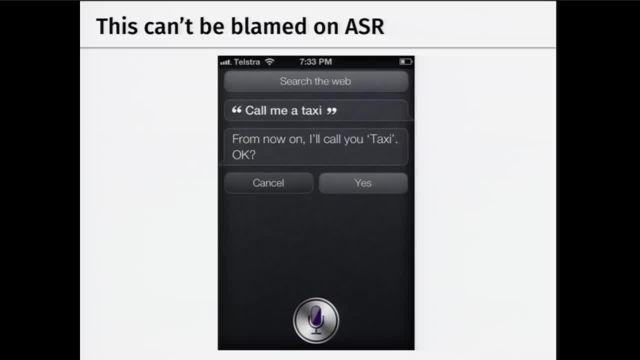 So this is ASR, but if so, I didn't get a picture for Cortana. I apologize, This is Siri, But if you were to say call me a taxi and Siri responded, from now on I'll call you taxi, okay. 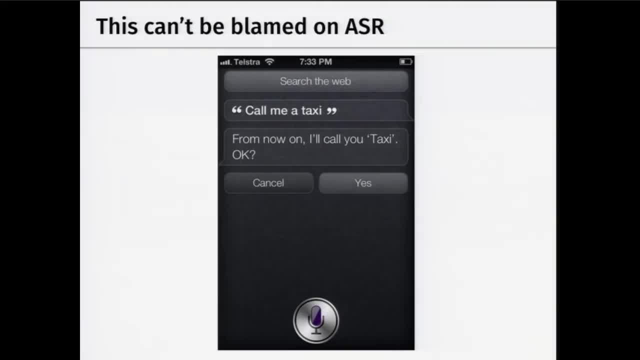 This is not the fault of an ASR system, So the ASR system did its job, but there's also a spoken language understanding module to which the ASR will feed into, And so that didn't do its job very well, and so it got the semantics wrong. 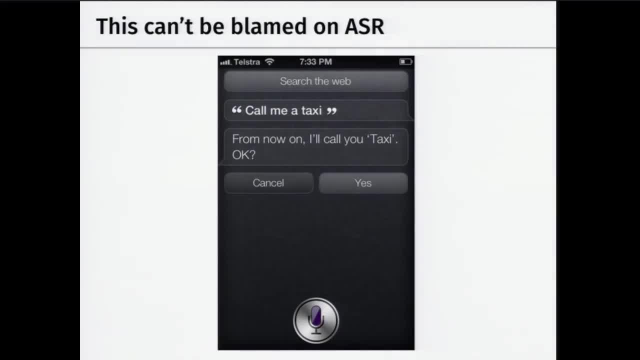 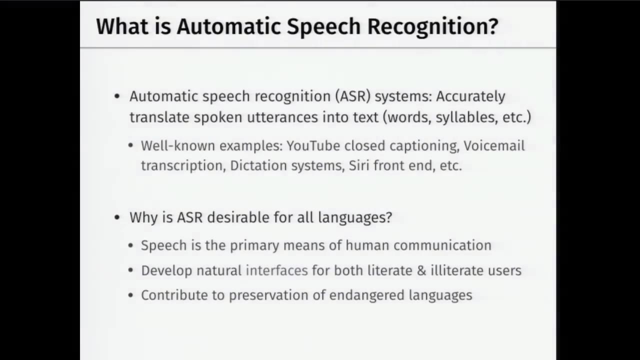 So people typically tend to collate the understanding and the transcription part as ASR. but ASR is strictly just translating the spoken language, The spoken utterances into text. So why is ASR desirable and why would you want to build ASR systems for maybe all languages? 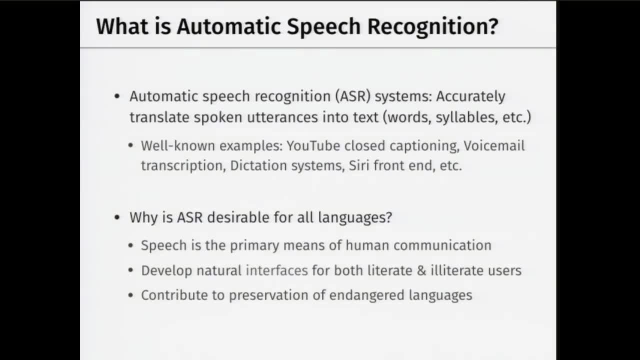 So obviously speech is the most natural form of communication. So rather than typing, which is much more cumbersome, you can speak to your devices, And if ASR systems were good, then that kind of solves lots of issues And it also keeps your hands free, which is not always a good thing. 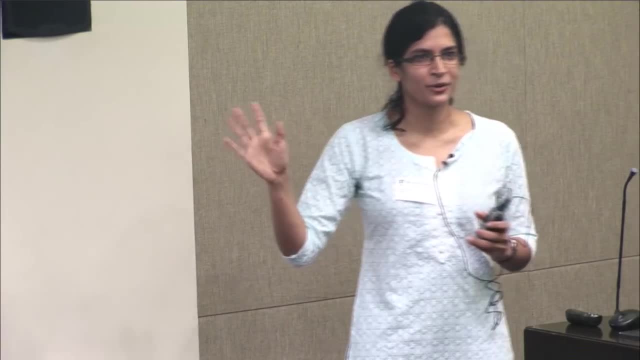 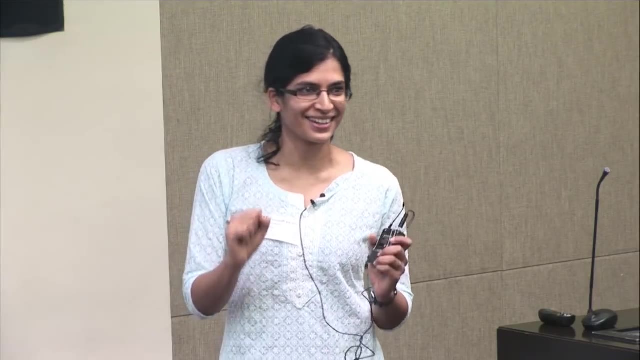 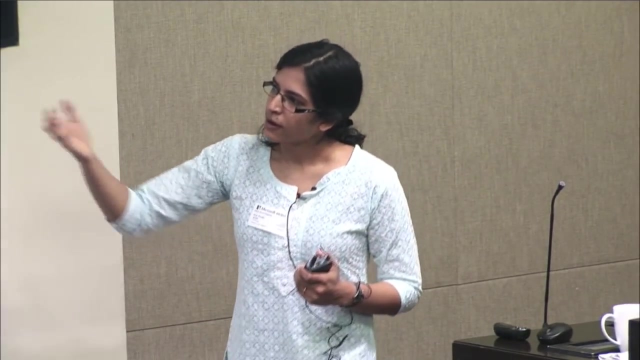 So many car companies like Toyota and Honda are investing quite a bit to build good speech recognition systems Because they want you to be able to drive and talk. I don't know if I entirely recommend it, but so clearly it leaves other modalities open to do other things. 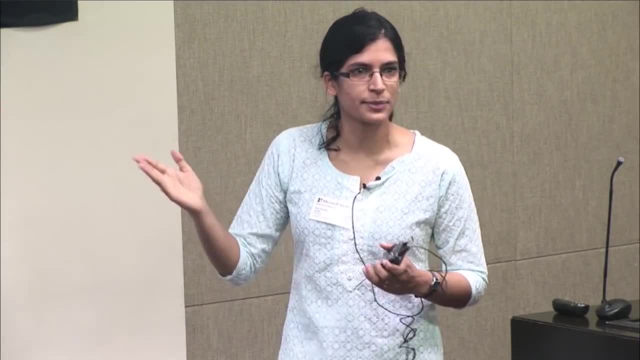 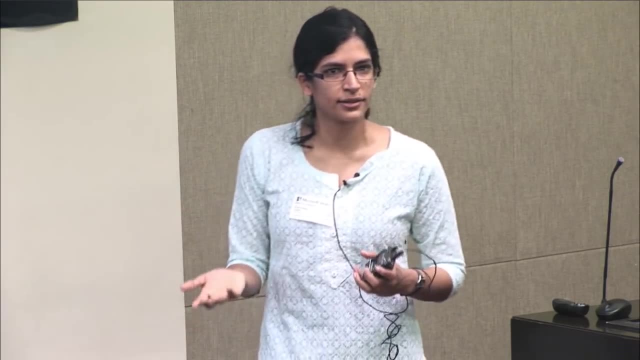 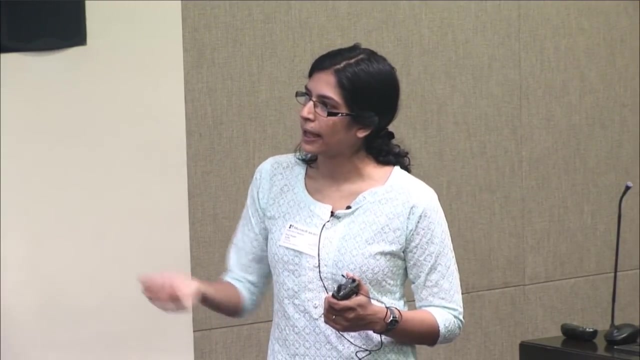 Also, another very kind of socially desirable aspect of building ASR systems is that now you have interfaces for technology which can be used by both literate and illiterate users, so even users who cannot read or write in a particular language can interact with technology if it is voice driven. 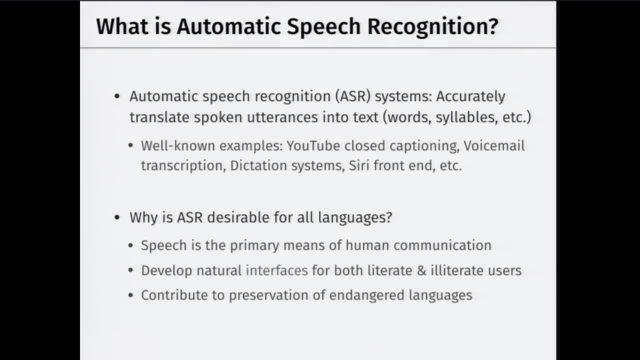 And this was endangered languages, which was a point which Monojit brought up- That lots of languages are currently close to extinction and all they've been given this endangered status. So if you have technologies which are built for such languages, it can contribute towards the preservation of such languages. 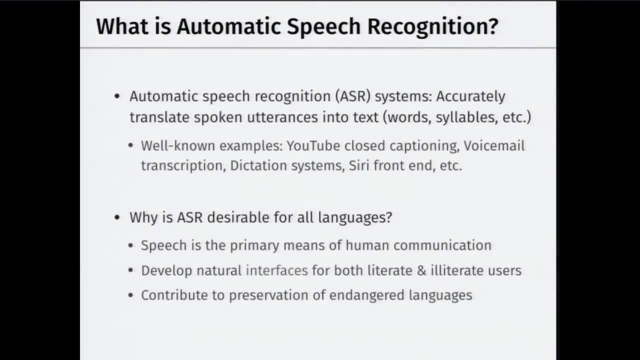 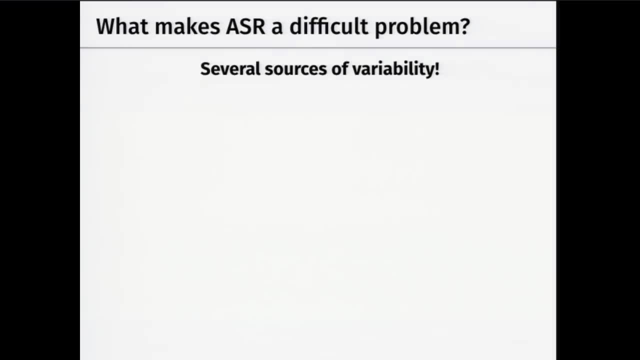 So that's just one kind of nice point of why you would want to invest in building ASR systems. So why is ASR a difficult problem? So the origins of ASR actually go way back. It's a long standing problem in AI back in the 50s. 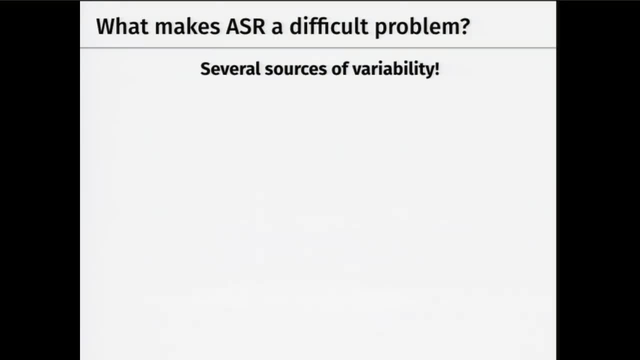 So why is it such a difficult problem? And clearly it's not very difficult for humans to do speech recognition, especially if you're familiar with the language. It's difficult because there are several sources of variability, So one is just your style of speech. 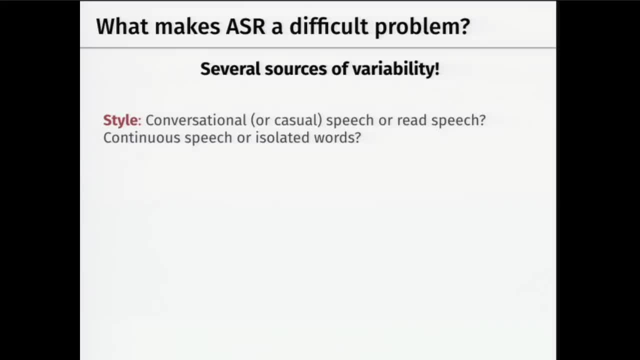 So currently the way I'm speaking it's kind of semi-spontaneous, but I more or less know what I'm going to say or how I'm going to say it by the points on the slides, And it's certainly continuous speech. 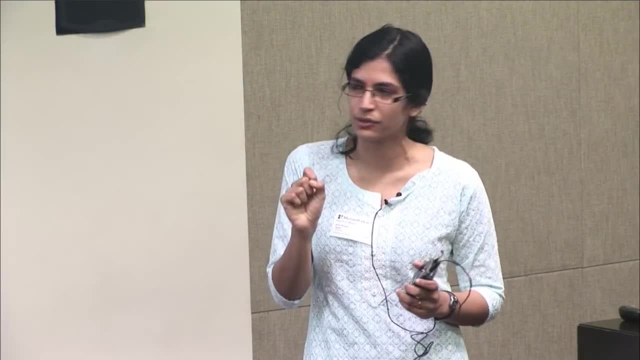 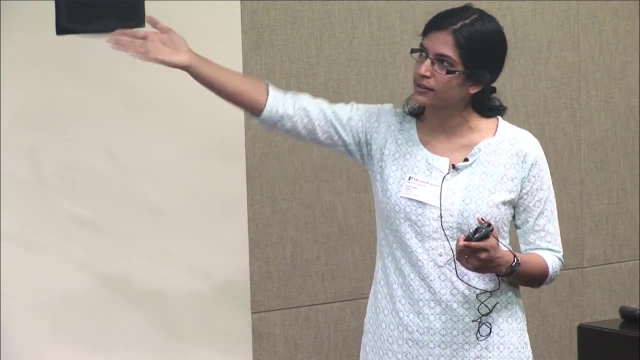 So I'm not speaking in any kind of staccato manner or I'm not saying isolated words. So just the style of speech can have a lot to do with how ASR systems will perform And, intuitively, isolated words are much more easier for. 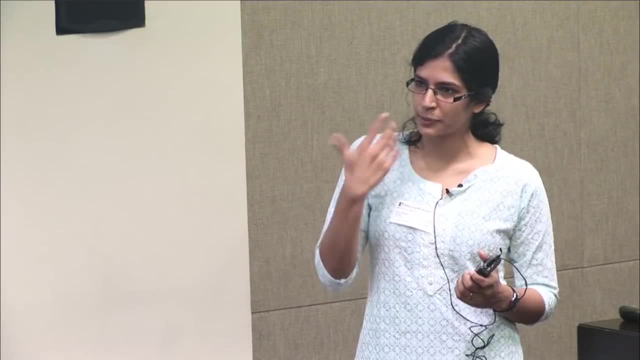 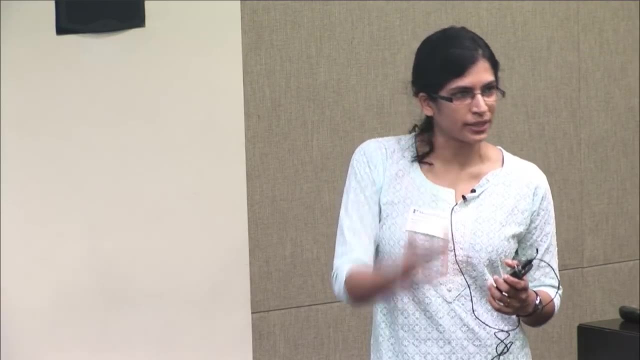 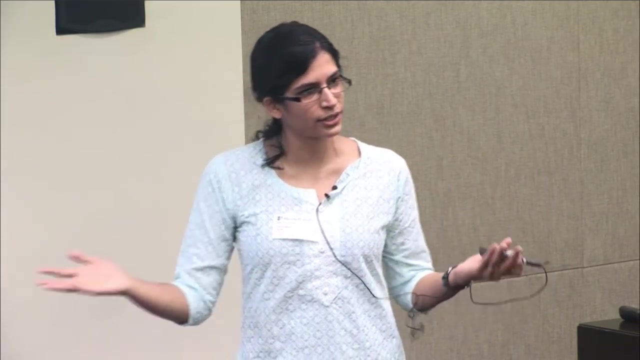 ASR systems than continuous speech, And that's because when you're speaking spontaneously, words are flowing freely into one another And there are lots of variations which come in due to variations, and there's this phenomenon of what's known as co-articulation. so it's just that words 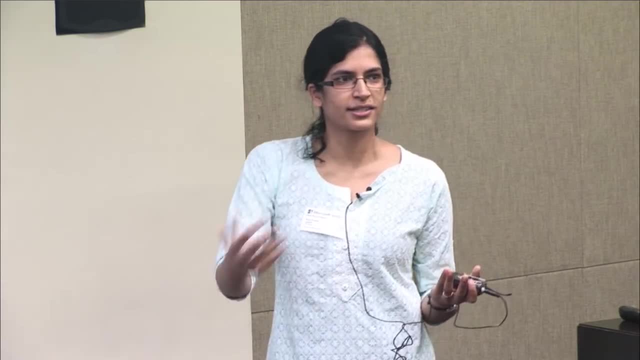 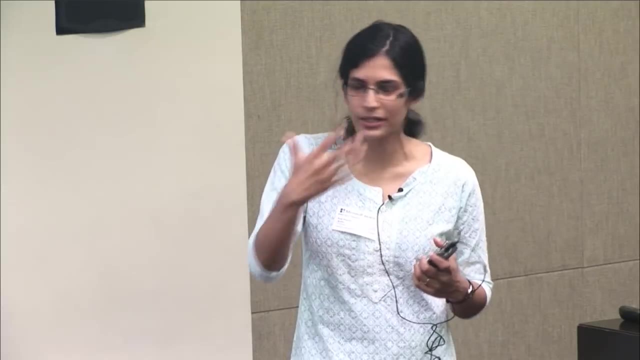 your preceding word affects the word which is coming, and so on, And so because of this kind of smooth characteristic of continuous speech that actually creates quite a lot of it's quite challenging for ASR systems to handle it. Of course, nowadays if you have lots and lots of data, 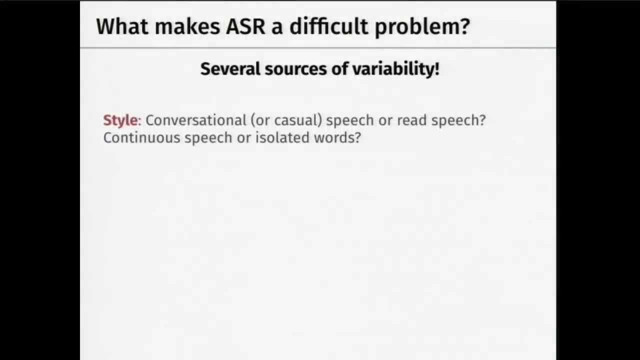 this is not really a problem. But this is one prominent source of variability. Another, of course, is environment. So if you're speaking in very noisy conditions or if your room acoustics are very challenging, for example, it's very reverberant, so you have a lot of echo. 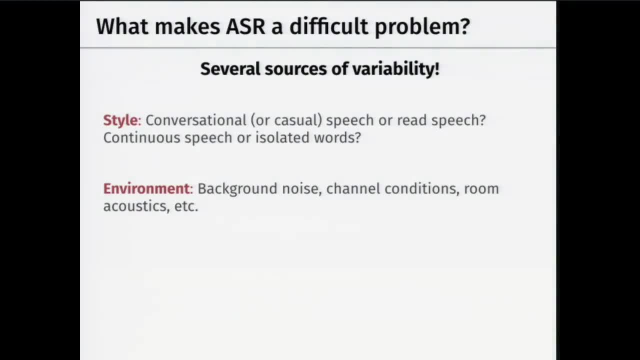 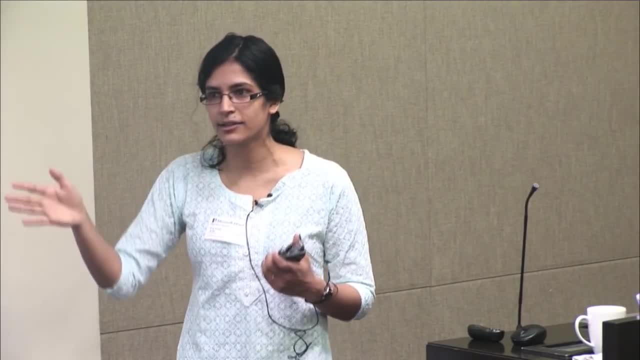 Or you're speaking in the presence of interfering speakers, so that's actually a real killer. So if you are talking and there's background noise, but the background noise is not like vehicle noise or something which can be easily isolated, but it's actually 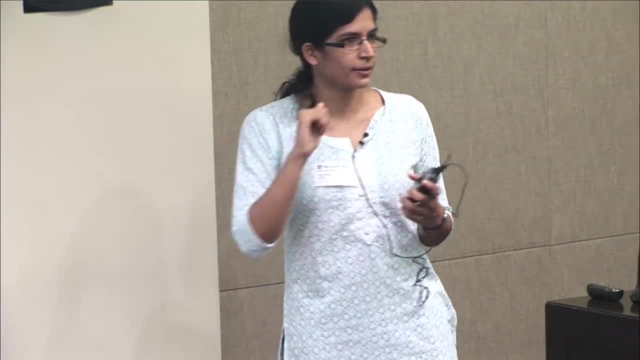 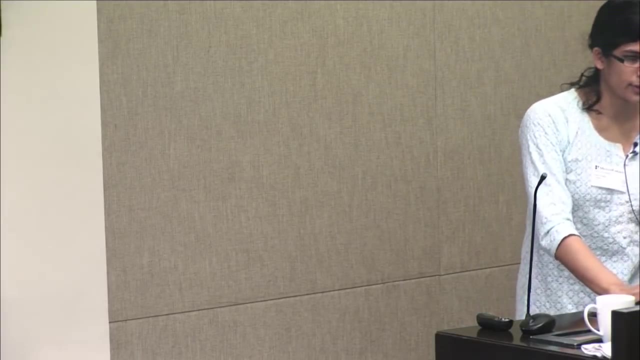 people talking in the background. That's really hard for ASR systems to kind of pick out the voice in the foreground and work on it. So environment is another important source of variability and something which people are very actively working on now to build what are known as robust ASR systems. 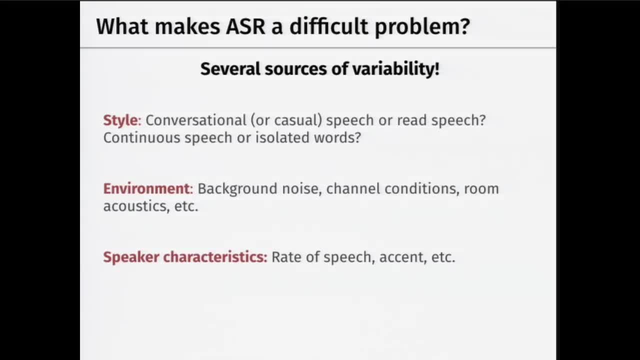 which are robust to noise. Then of course, speaker characteristics, So all of us have different ways of speaking. So of course accent comes into play, Just your rate of speech. some people speak faster, some people enunciate faster. 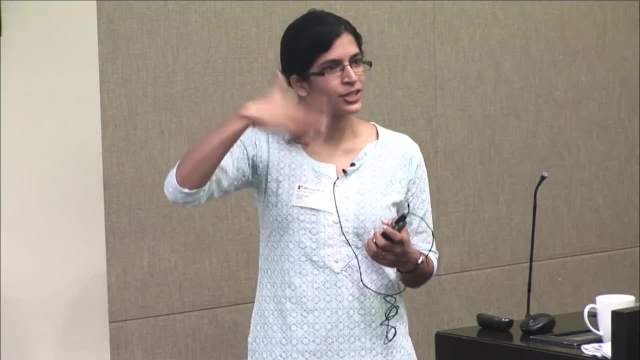 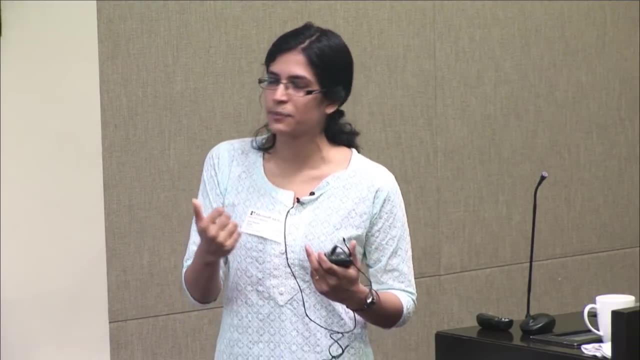 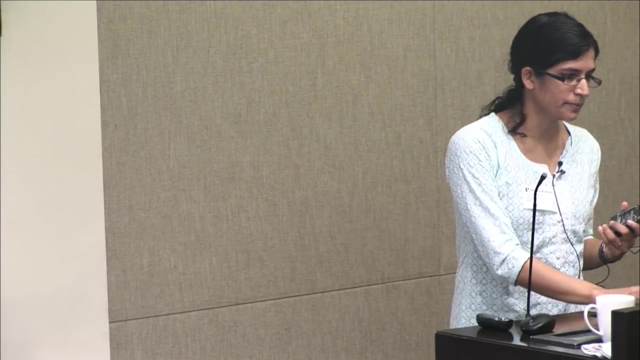 Some people enunciate more. Of course your age also changes the way your characteristic of your speech. so the child's speech is going to be very different from adult speech. So various characteristics of speakers also, which contribute to making ASR a challenging problem. 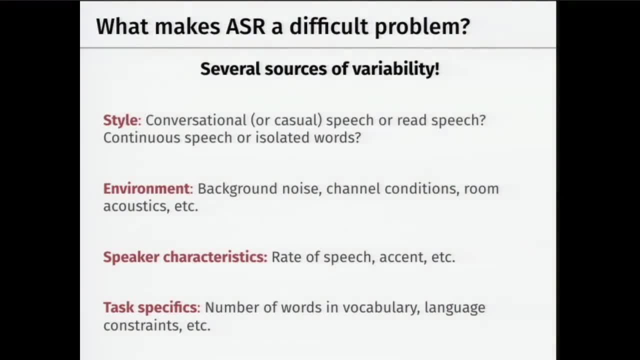 And of course there are lots of task specific constraints, So, for example, the number of words in your vocabulary which you're trying to recognize. So if you're looking at, say, voice search applications, they're looking at a million word vocabularies. 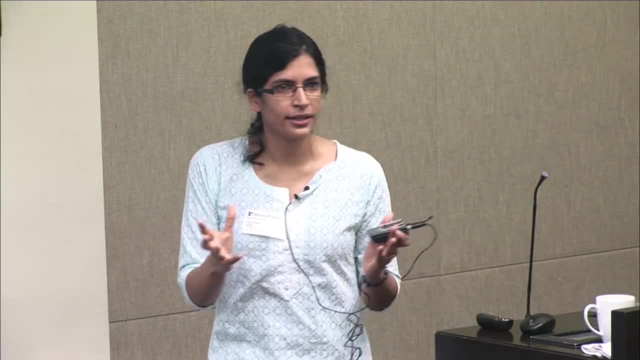 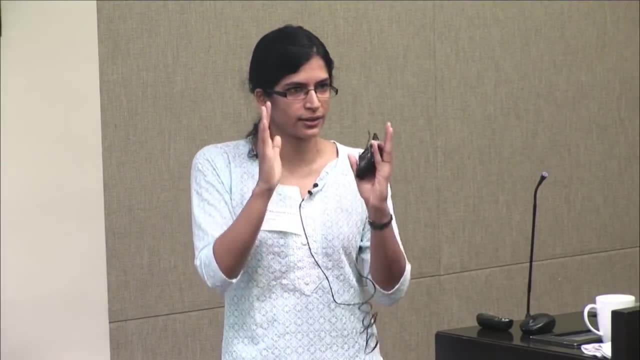 But if you're looking at a command and control task, where you're only trying to move something or your grammar is very, very constrained there, your vocabulary is much smaller, so that task is simpler And you might also have language constraints. 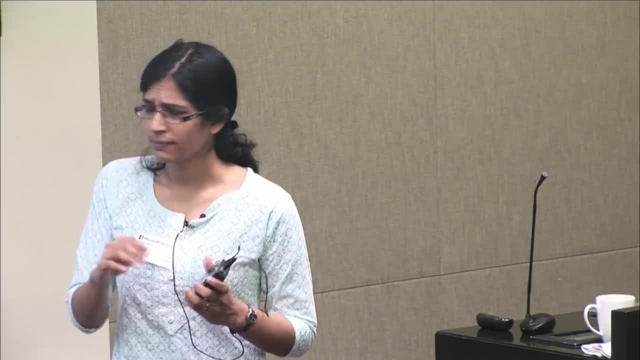 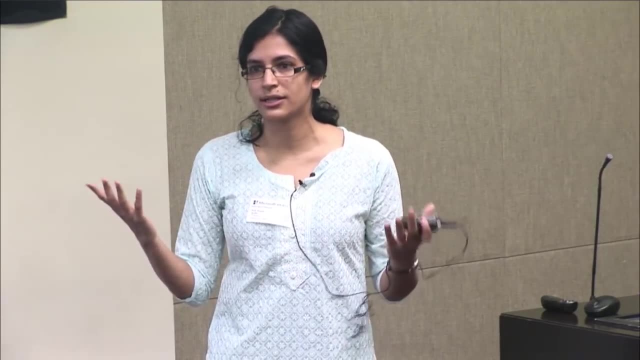 So maybe you're trying to recognize speech in a language which doesn't have a written form, so it doesn't have transcripts at all. then what do you do? Or you're working with a language which is very morphologically rich, or it has words which have 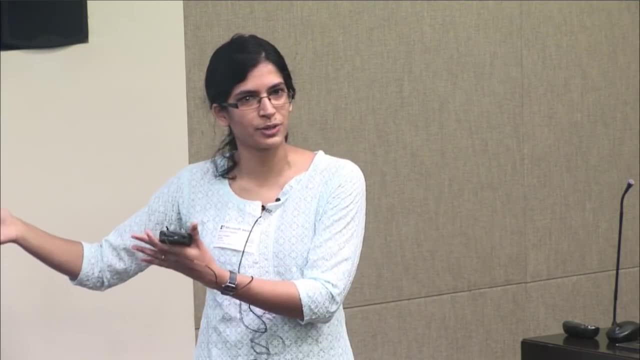 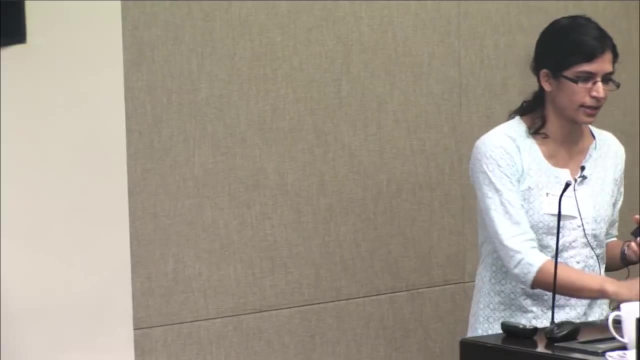 agglutinative properties. So then, what do you do with your language models? Maybe n-grams are not good enough. So lots of task specific constraints also, which contribute to making this a challenging problem. Okay, so hopefully I've convinced you that ASR is. 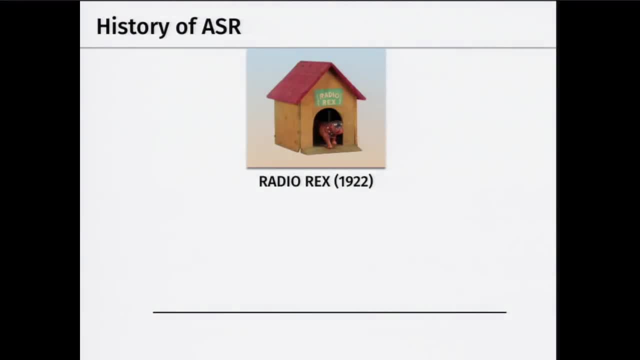 quite a challenging problem to work on. So let's kind of just go through the history of ASR- and this is just a sampling. I'm not going to cover most of it, but I'm going to cover most of the important systems. 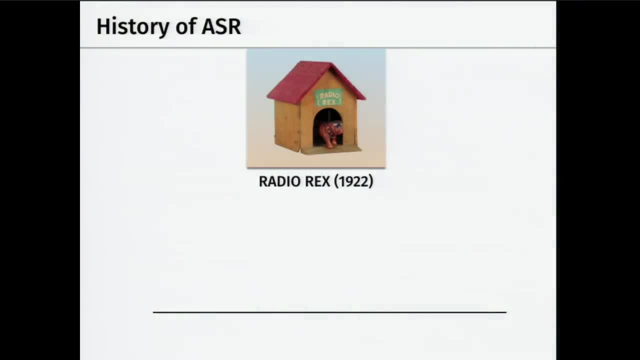 There's been a lot of work since the 50s. This is actually the 20s, but I'll talk a little about what this is. So the very first kind of ASR- and I'm air coating because it really isn't doing any recognition of any sort. 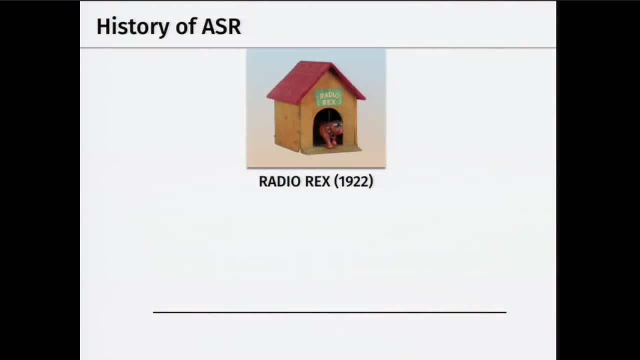 But it's this charming prototype called Radio Rex. So it's this tiny dog which is sitting inside its kennel and is controlled by a spring, which in turn, is controlled by an electromagnet, And the electromagnet is sensitive to energies at frequencies around 500 hertz. 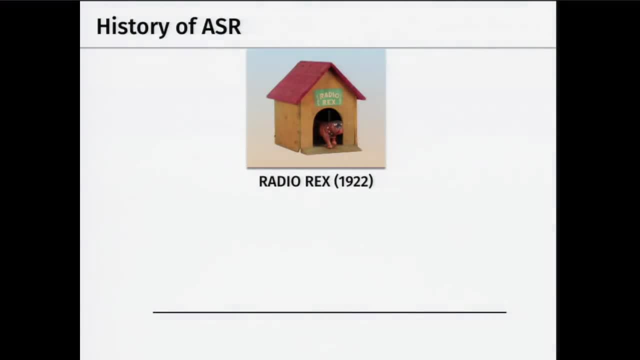 And 500 hertz happens to be the frequency of the bubble sound. eh in Rex. So when someone says Rex, the dog will jump out of the kennel. So this is purely a frequency detector, so it's not doing any recognition. 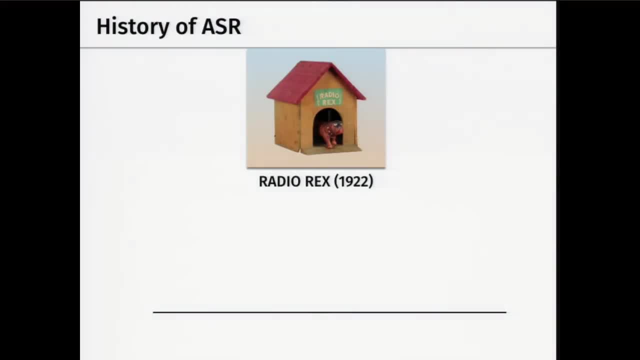 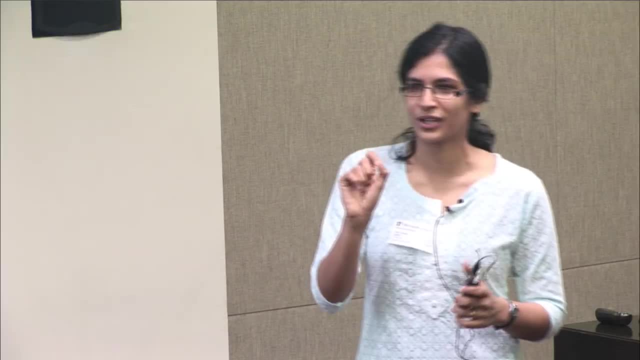 But it's a very charming prototype. But clearly I mean, can anyone kind of there's so many issues with this right, But with this kind of a system and your hard coding, okay, it needs to fire at this. It needs to fire at this 500 hertz. 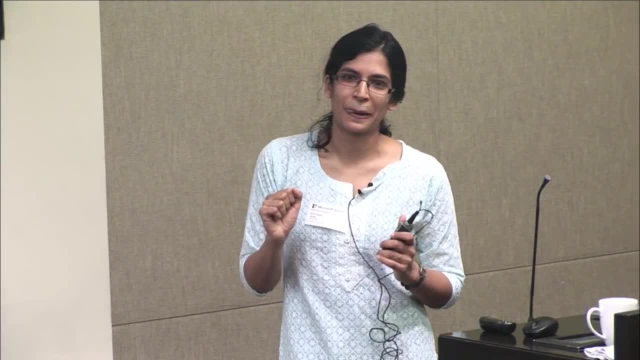 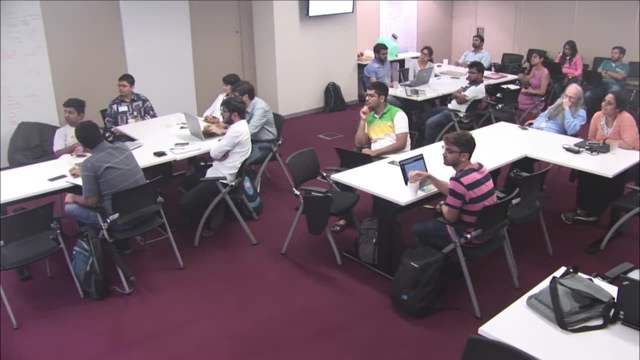 What is an obvious problem with such a prototype? Noise? Noise, yeah, of course, Different people it might not- Yeah, exactly. So this only works for adult men, So it's sexist and it's ageist. It doesn't work on children's speech. 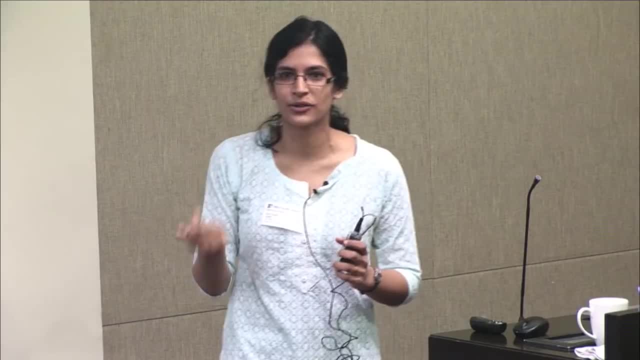 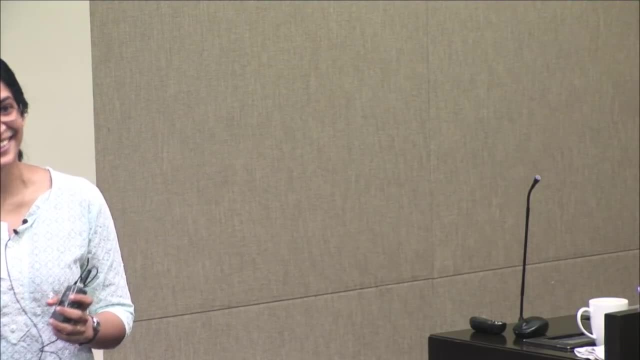 It doesn't work on female speech. So, yeah, that's obviously an issue when you hard code something, But this is so. this is actually. I recently discovered this is on eBay And you can- Can I just-. Yeah, I wanted one of these. 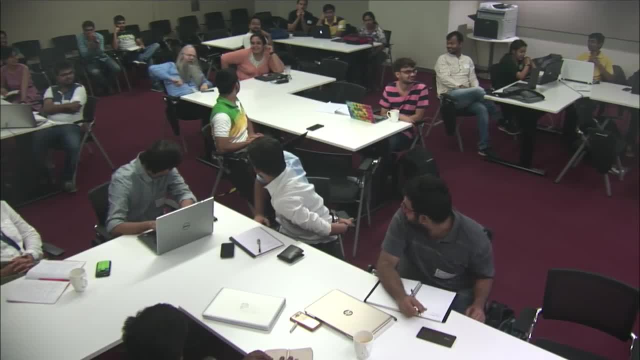 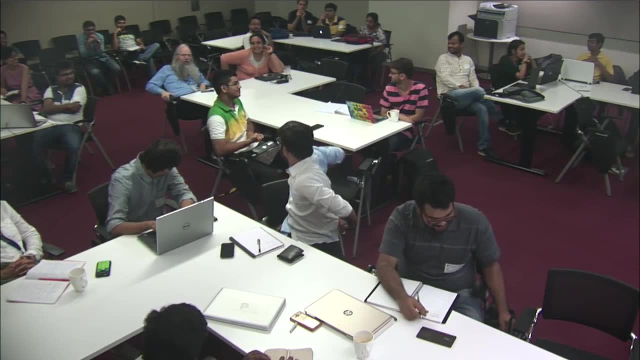 Oh, really, Okay, yeah, yeah. yeah, There was one on sale for- Yes, And so I started bidding, actually created my account to bid for this thing, And then I noticed the person who kept bidding on top of me. 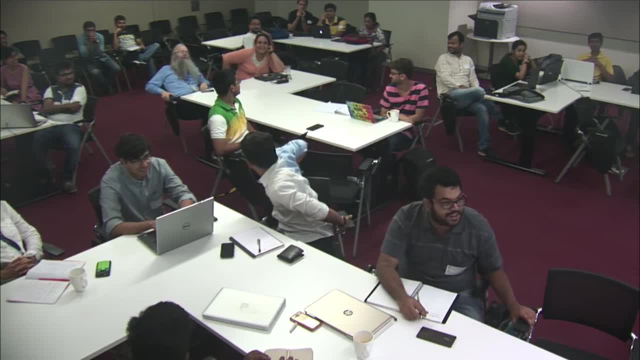 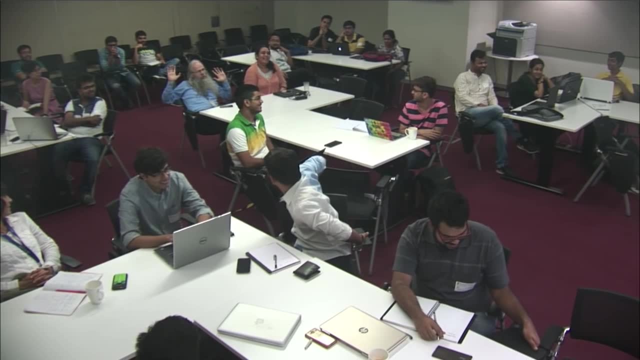 was someone who's called Henrik Hermanski, Oh no, Who's a professor at JSU, because he wanted one as well. Oh okay, so he-. So I stopped bidding and asked him for the video. if he gets it. 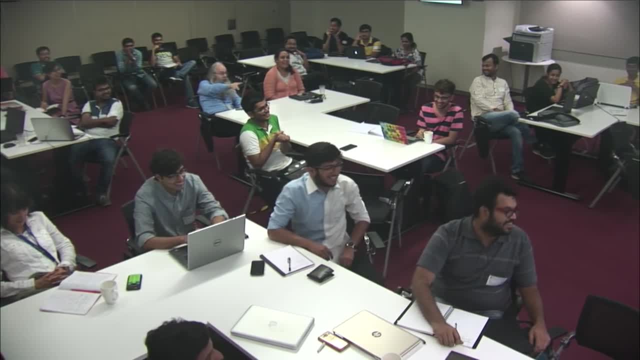 So he didn't buy it. He doesn't give me the video. He doesn't give me the video, but he did buy it. Wow, okay, Okay, so I can add that to my slide. Yes, That Henrik has this now. 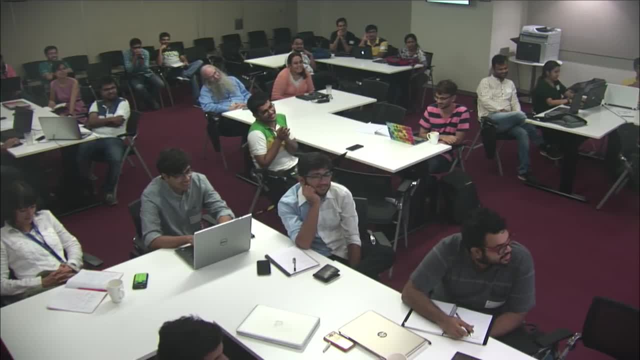 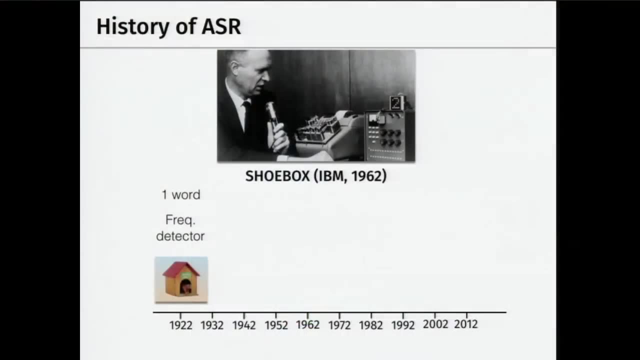 Yeah, Henrik has it. yeah, Okay, so that's the very initial prototype. But that's single word and it's a frequency detector, So this is not really doing recognition. So the next kind of major system was Shoebox, which was in 1962, and it was by IBM. 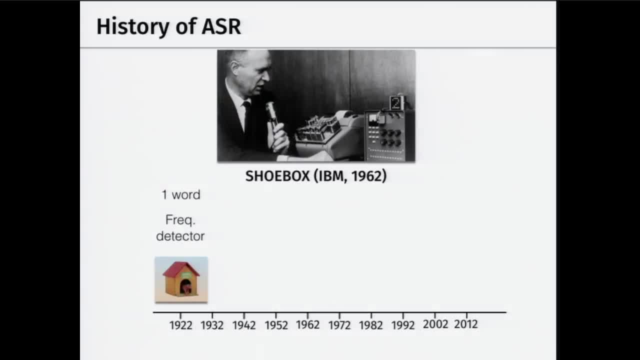 And they actually demoed the system and it did pretty well. But what it was recognizing was just connected strings of five digits, So it's just purely a digit recognizer and a few arithmetic operations. So it could do basic arithmetic. You could say six plus five is, and so on. 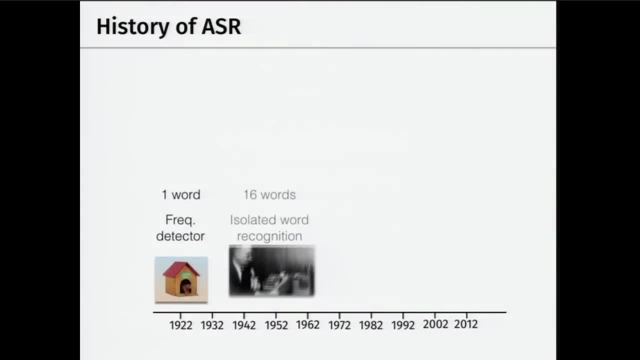 So it would perform really well, But of course this is also very limited, So it's just a total of 16 words, so 10 digits and six operations, And it's doing isolated word recognition. So actually, sorry, this is not connected speech. 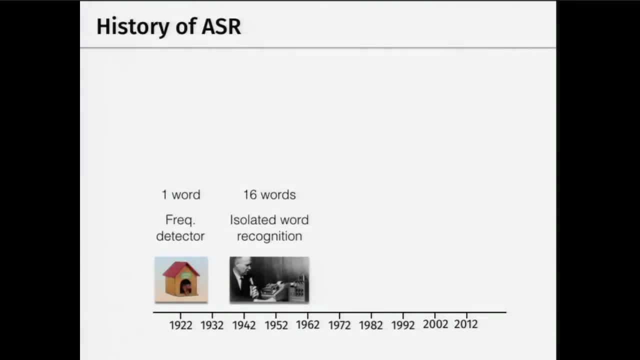 You would have to say it with a lot of pause in between each of the individual words, So this was just doing isolated word recognition. And then in the 70s there was a lot of interest in developing speech recognition systems and AI-based systems. 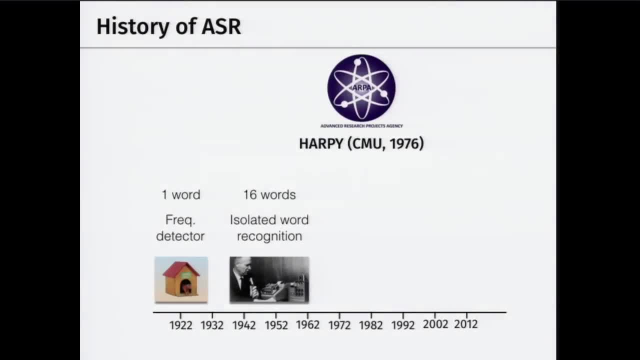 And ARPA, which is this big agency in the US, funded this $3 million project in 1975. And three teams worked on this particular project And the goal was to build a fairly advanced speech recognition system which is not just doing some isolated word recognition. 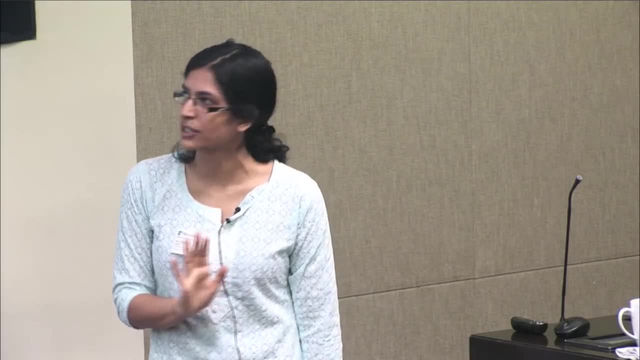 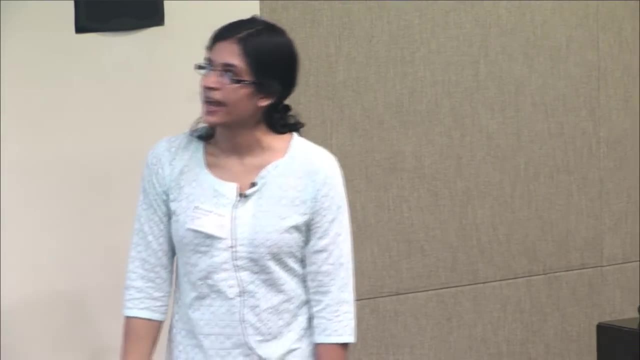 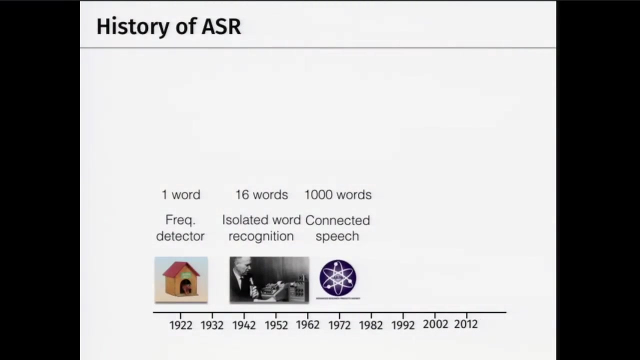 It would actually evaluate continuous speech, And so the winning system from this particular project was Harpy out of CMU, And Harpy actually was recognizing connected speech from a thousand word vocabulary. So we are slowly making progress, But it still didn't use statistical models. 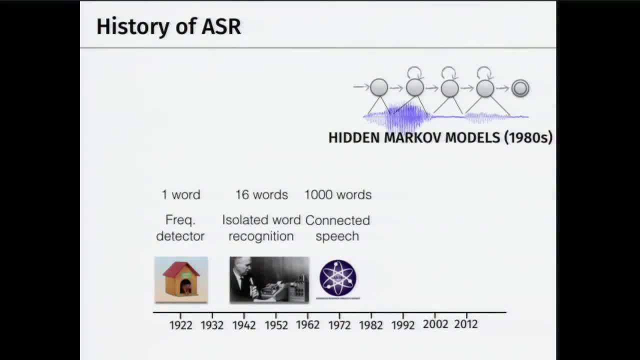 which is kind of the current setting, And this was in the 1980s, kind of pioneered by Fred at IBM and others. around the same time, Statistical models became very, very popular to be used in speech recognition And the entire problem was formulated as a noisy channel. 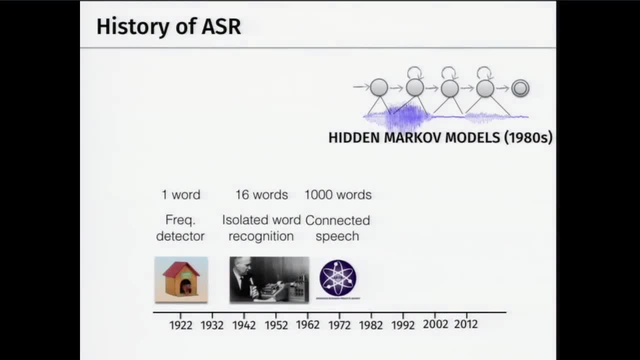 And one of the main machine learning paradigms which was used for this particular problem were hidden Markov models. So I'll come to this not too much in detail, But at least at a high level. I'll refer to this in coming slides. 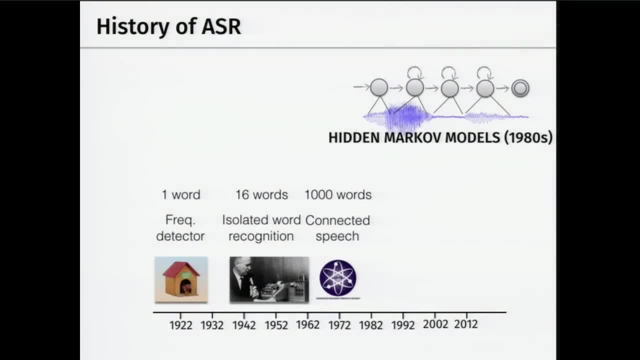 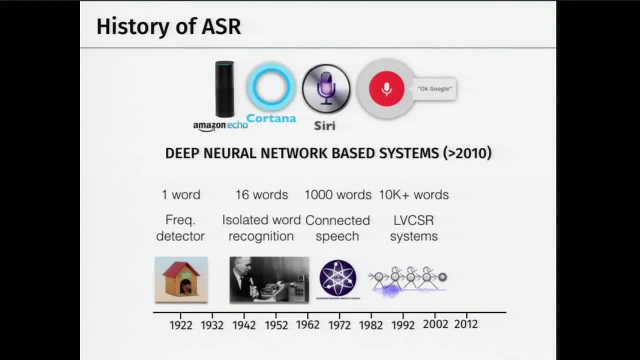 So these statistical models were able to generalize much better than the previous models, Because the previous models were all kind of rule based And now we are moving into 10K vocabulary sizes. So the vocabulary size is getting larger And these are now kind of falling in what are known as large. 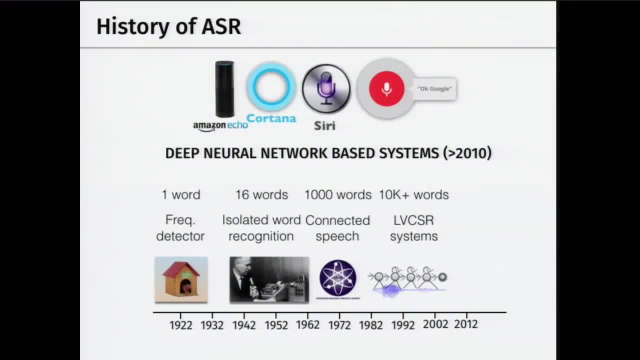 vocabulary, continuous speech recognition systems- Although of course now large vocabulary is much larger than 10K. But that was in the 80s And we were in this plateau phase for a long time. And in 2006, deep neural networks kind of came to. 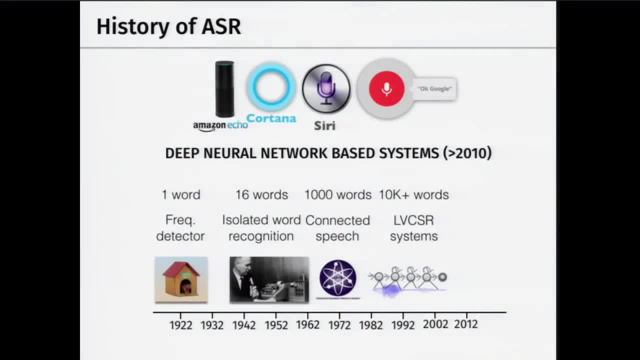 the forefront, And now all the state of the art ASR systems are powered by deep neural networks. So any of these systems you might have used- Cortana, Siri, Voice Search- they're all at the back end. they're powered by deep neural network based models. 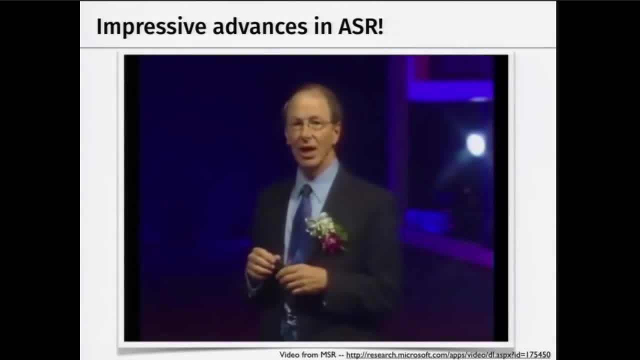 So this is just a video which was actually quite impressive- And this happens to be by the CFO of Microsoft, Rick Rashid, And this was a really impressive video. So this came out in 2012, when Microsoft had completely shifted to deep neural network based models in the back end. 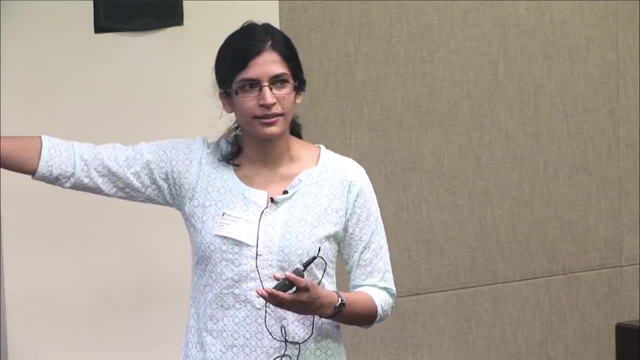 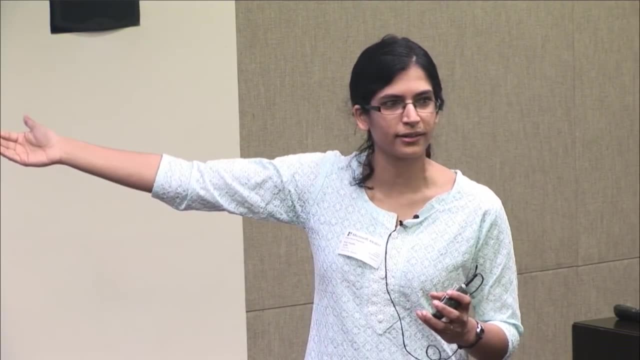 I mean even in their production models And this actually. so he's speaking And in real time. the speech recognition system is working and giving transcripts And you will see that the quality of the transcriptions is really good. And while the transcriptions were being displayed on, 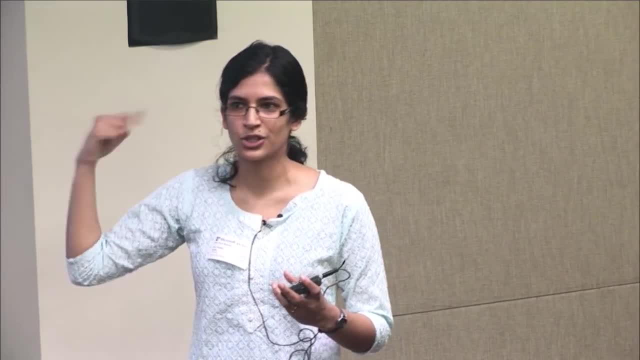 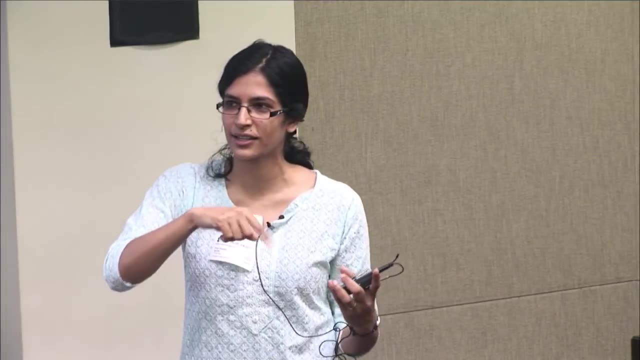 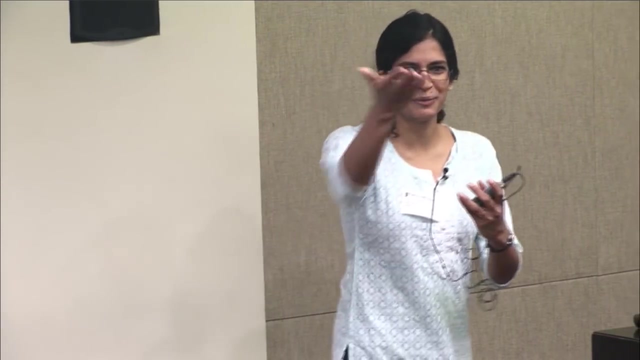 the screen they were also doing translation into Chinese, And so there was another screen where their MT system, their machine translation system, was working and producing real time Mandarin transcripts. So it was a very impressive demo And I'm told it was not. 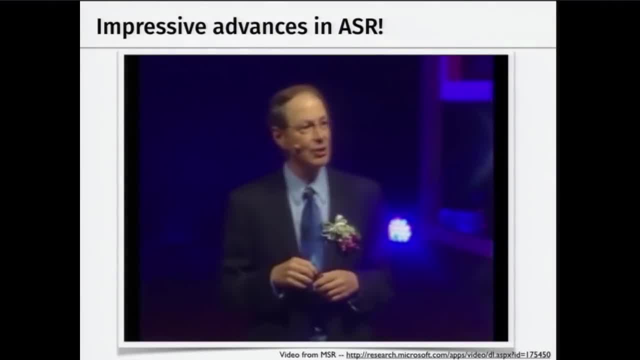 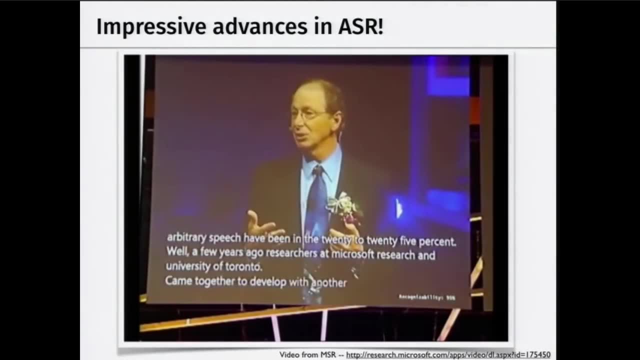 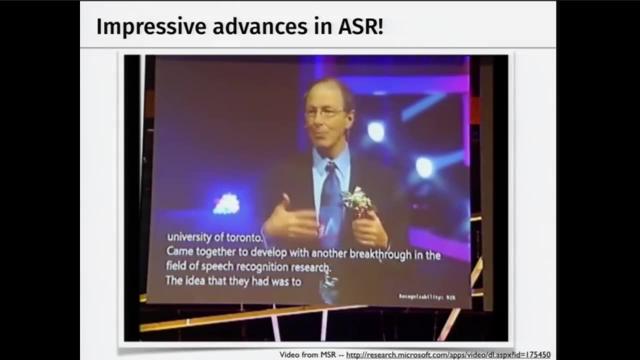 but Sunaina knows more about the demo itself. University of Toronto came together to develop another breakthrough in the field of speech recognition research. The idea that they had was to use a technology in a way patterned after the way the human brain works. 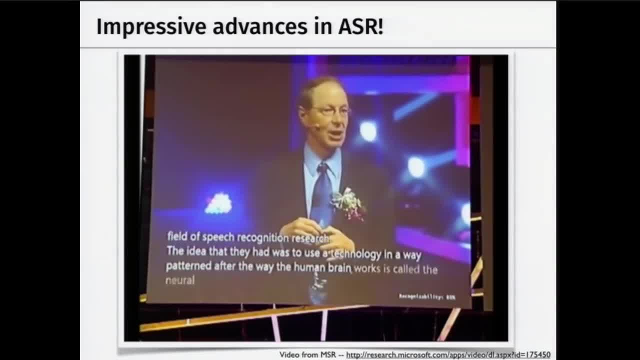 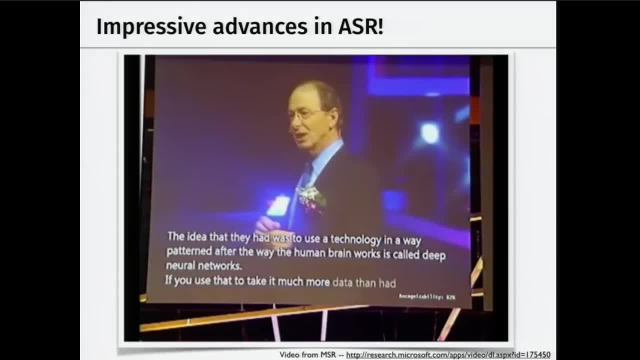 It's called deep neural networks, And to use that to take in much more data than had previously been able to be used with the hidden Markov models, and use that to significantly improve recognition rates So that one change, that particular breakthrough. 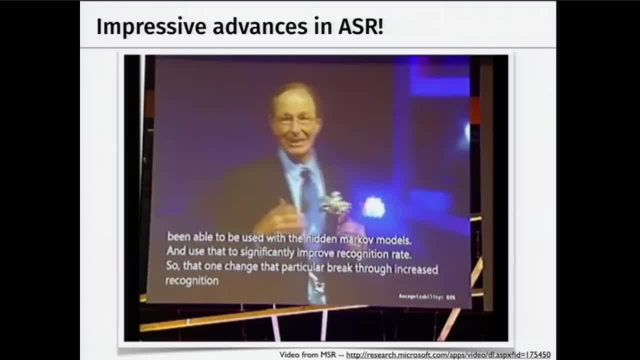 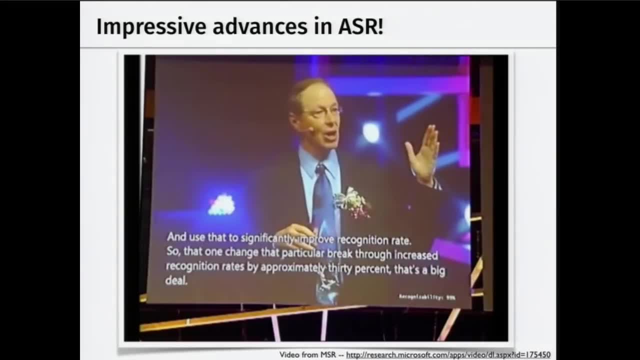 increased recognition rates by approximately 30%. That's a big deal. That's the difference between- Okay, So you can see, the transcripts are pretty faithful to the speech And this, I'm told, was not. it was actually happening in real time. 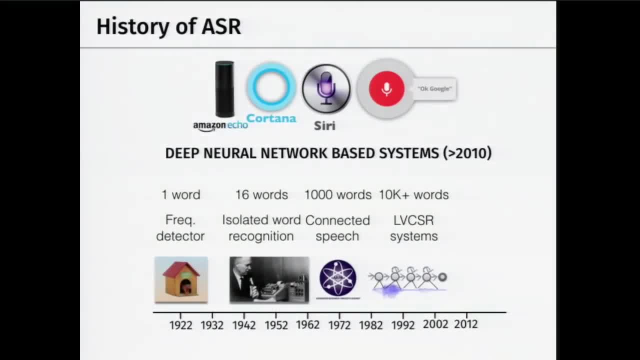 So that's really impressive. Okay, so, given all of this, so you might be wondering what's next. So whenever I tell people I work on speech recognition, I'm asked this question many times. isn't that problem solved? So what are you doing? 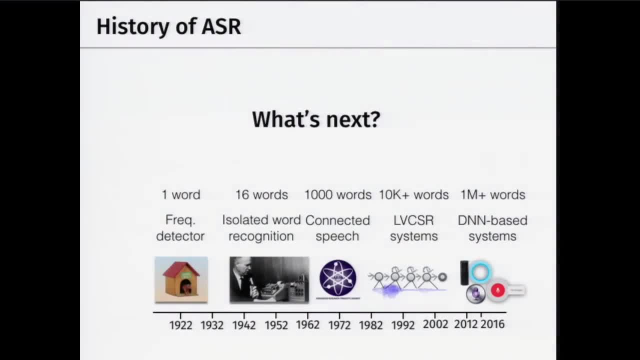 What are you continuing to work on, So okay? so just to kind of motivate this question and also kind of related to the topic that our team is working on, which is accent adaptation, I'll show you a video of our 12th president of India. 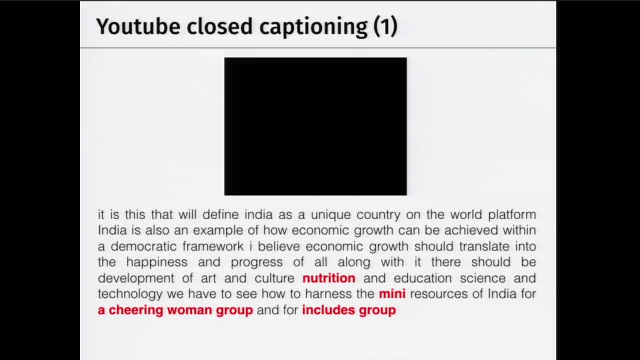 So this is Pratibha Patel. So she's sitting in a closed room and she's giving a speech, And this is YouTube's automatic captioning system, which is working. So this is a really state of the art ASR system. 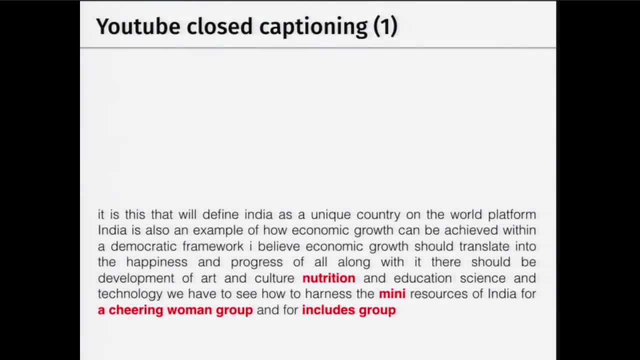 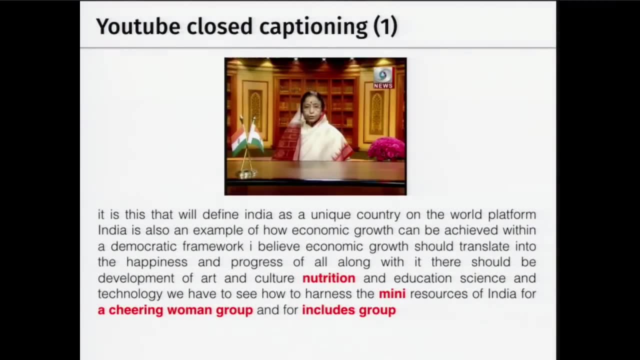 And I got this a few months back, So let's look at the video That will define India as a unique country on the whole platform. India is also an example of how economic growth can be improved and achieved within a democratic framework. I believe economic growth should translate into the happiness. 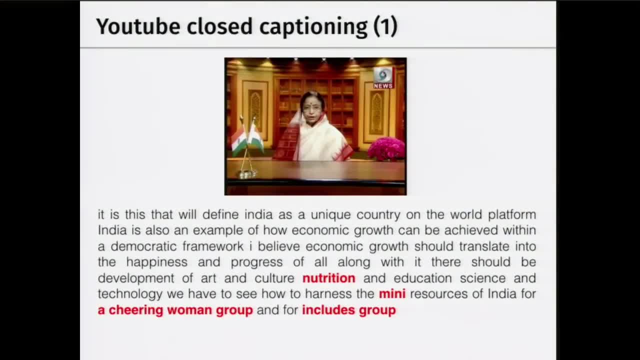 and progress of all. Along with it, there should be development of art and culture, literature and education, science and technology. We have to see how to harness the many resources of India for achieving common good and for inclusive growth. Okay, So the words in red, of course, are the erroneous words. 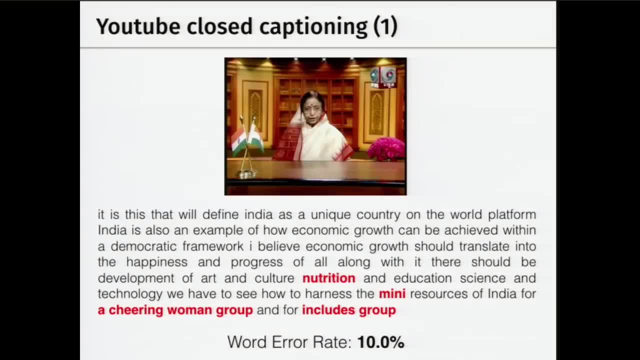 And this is not bad at all. So if you look at this metric, which is typically used to evaluate ASR systems, so this is the word error rate, So it's just the. if you take this entire word sequence and you take the true word sequence and 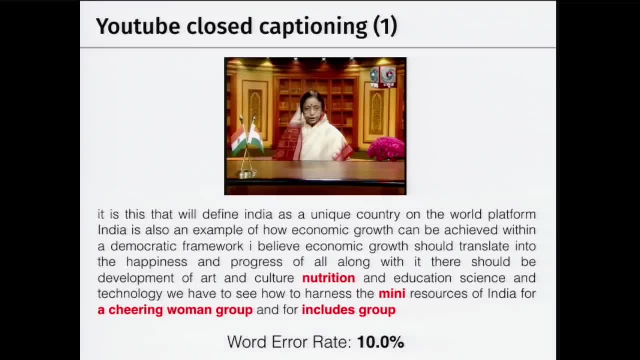 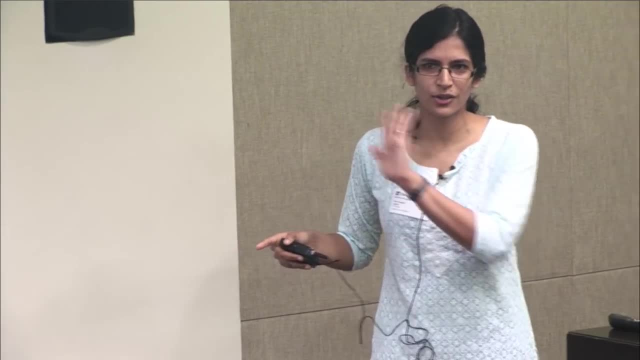 you compute an edit distance between these. So just align these two sequences and compute where the words are actually swapped for other words and where certain words are inserted And where certain words are deleted, and you get this error rate And that's 10%, which is fairly respectable. so that's not bad. 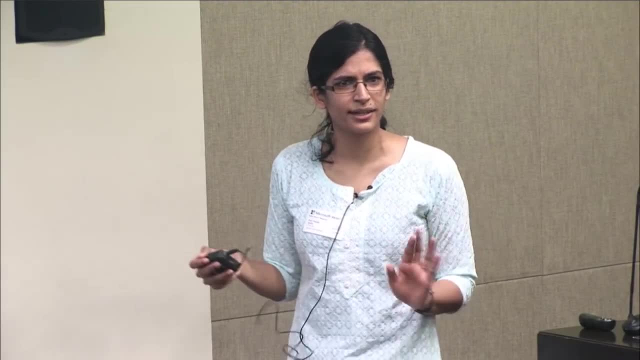 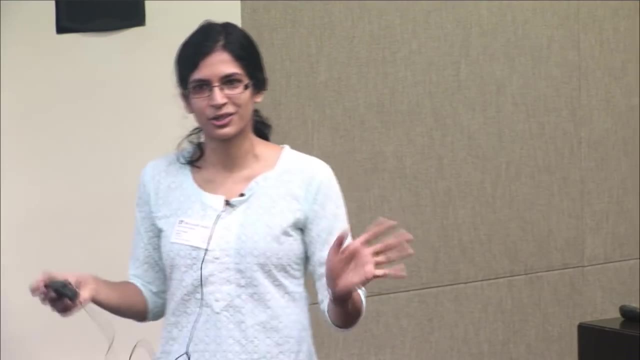 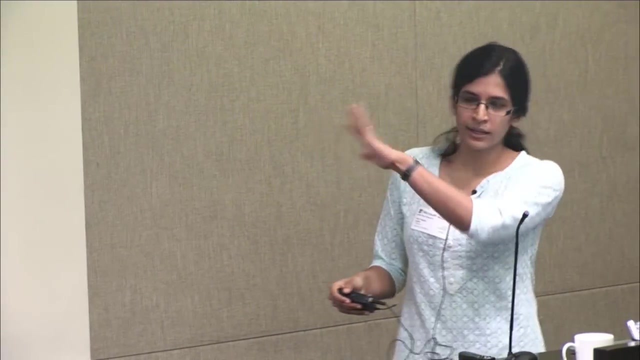 And that's because Google has a very, very well developed Indian English ASR system And Google actually calls all of these variants of English different languages. So they have Indian English, Australian English, British English, various variants of English, And their system is extremely sophisticated for. 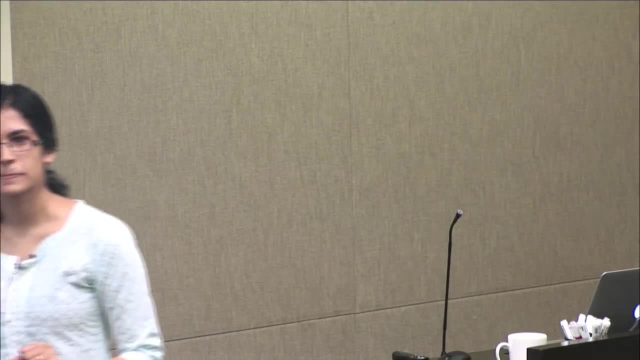 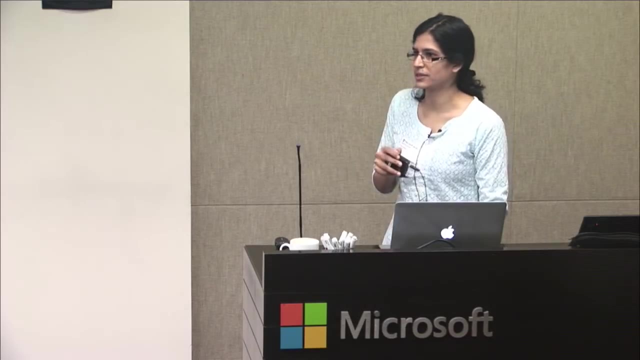 Indian English. Yeah, it's clean, it's quiet, Exactly, yeah. So now let's take speech from our 11th president, who is Abdul Kalam, And why I picked him is because he has a more pronounced accent. 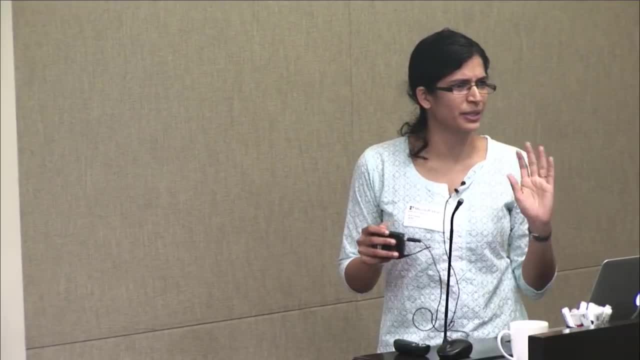 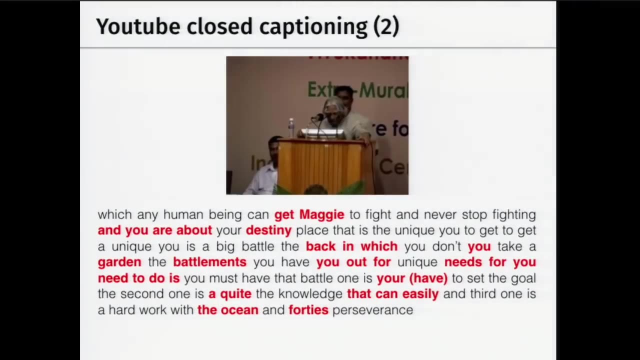 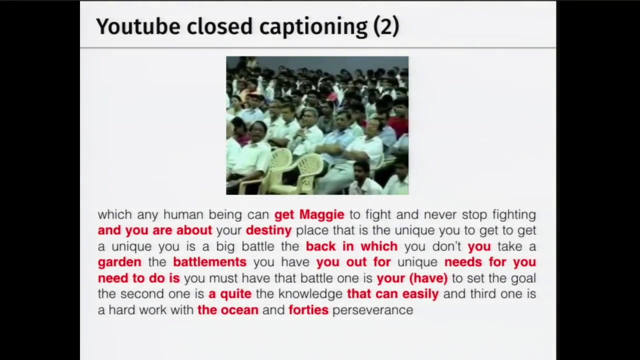 Most of you must have heard his speech at some point. So let's look at how- Which any human being can ever imagine- to fight And never stop fighting until you arrive at your destined place. That is the unique you. To get the unique you, it's a big battle. 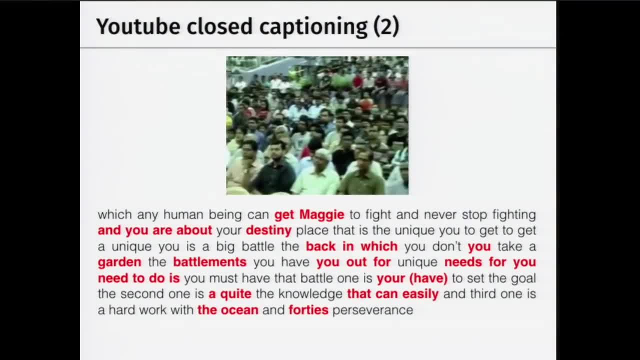 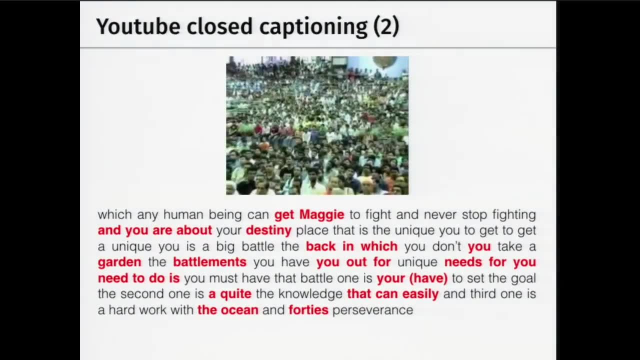 The battle means you don't need to take a gun. The battle means you have to have four unique things, four unique tools you must have in that battle. One is you have to set the goal. The second one is acquire the knowledge continuously. 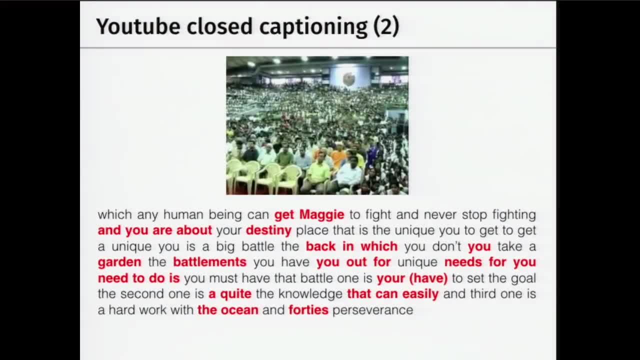 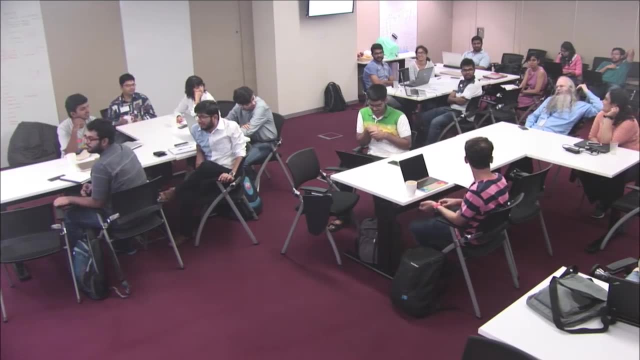 And third one, it's hard work with devotion. And fourth is perseverance. Okay, so I'm actually curious, Alan: how do you think you would have done with recognizing this? So I would definitely make errors, okay, Yeah, yeah. 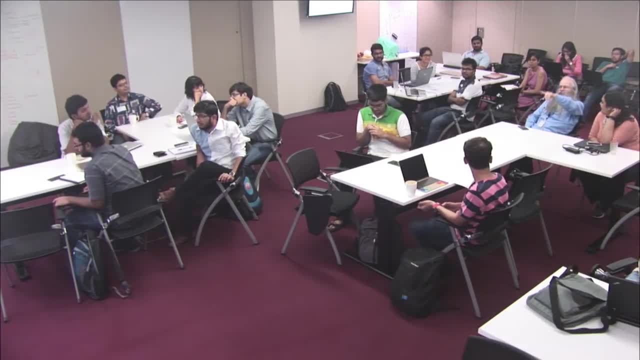 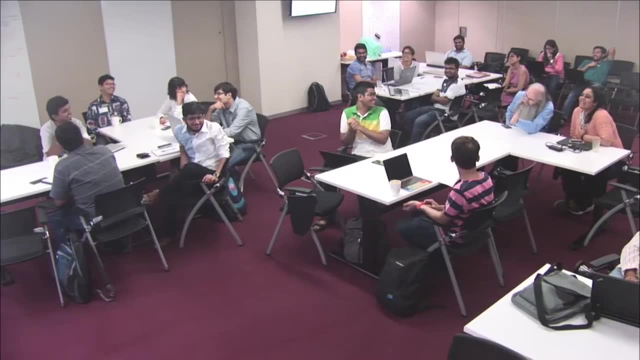 Because he is much more heavily accented. And what's really hard is, if you're following the transcript, I'm thinking, yeah, that's exactly what I said. No, no, no, no. I would use a language model and not just stick to it. 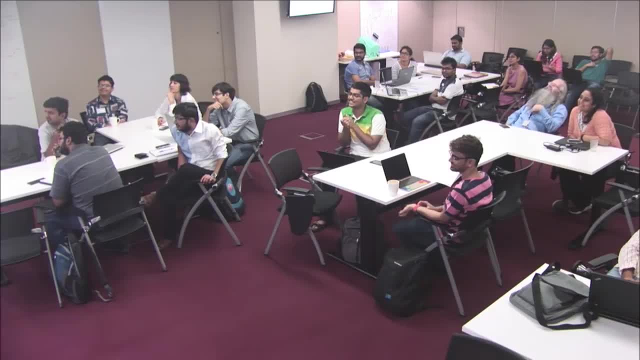 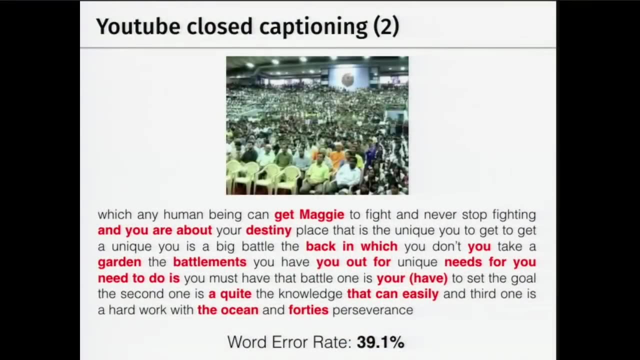 and not seeing the transcript. Yeah, yeah, I think most of us in the room are definitely gonna do better than this right, Definitely better than 39%. So actually, I've shown this video before And some people from the crowd said: but this is not fair. 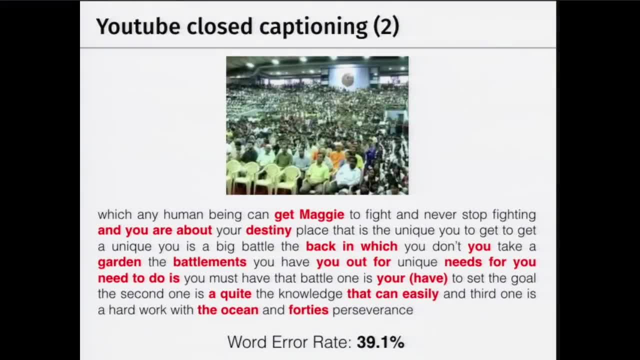 Because not only I mean cannot entirely attribute it to accent, because he's in this large room. It's more reverberant than the previous video. His sentence structure is quite nonstandard. He moves in and out of various sentences And, of course, reading. 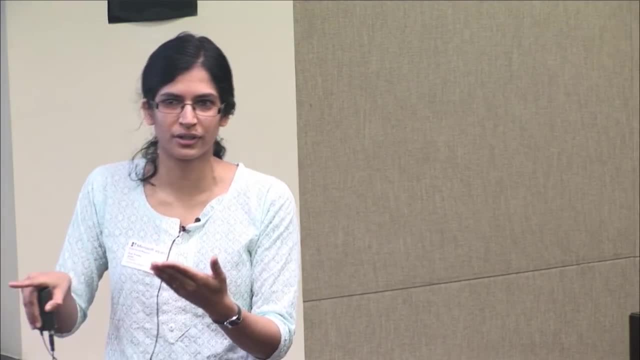 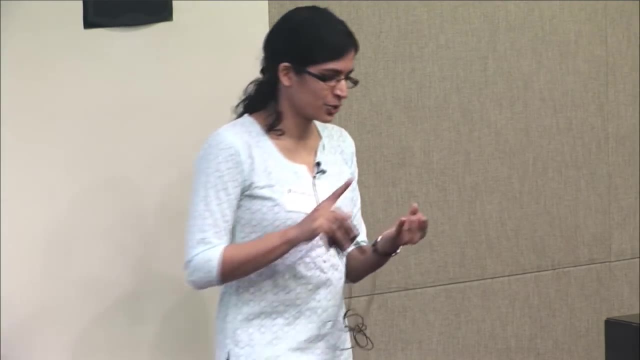 So it's hard. So the read speech has a very, very different kind of grammatical structure than this, right? So I said, okay, let's try to make it fairer, right? So I chose someone who is an American English speaker, but 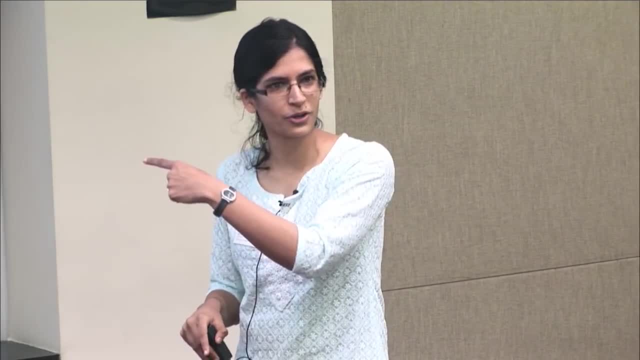 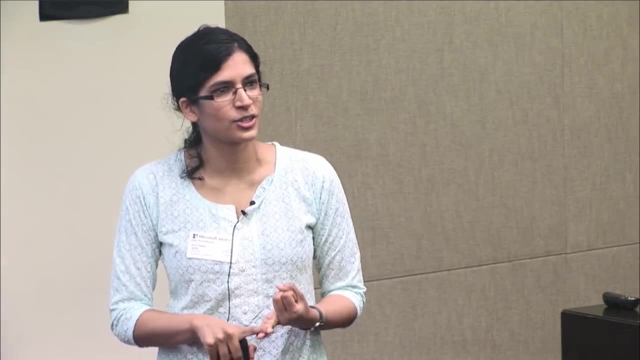 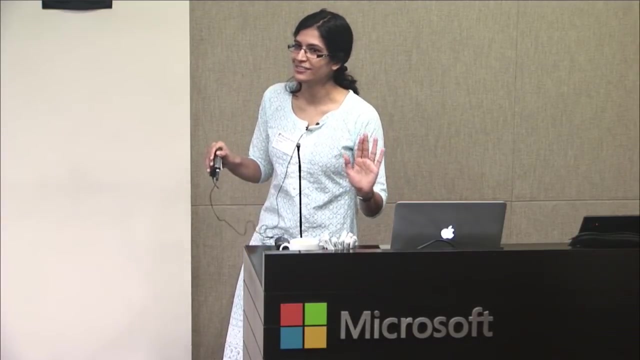 has an accent, Because my hypothesis is that accent had a lot to do with this misrecognition rate getting higher. So this is an American English speaker who has a strong accent and has very nonstandard word order, And so an obvious choice was Sarah Palin, if you know who she is. 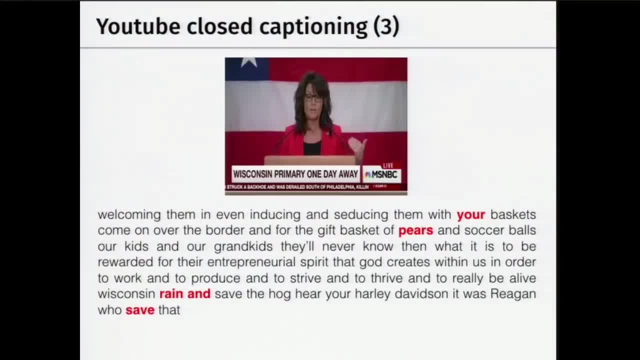 Most of you know who Sarah Palin is. okay, Illegal immigrants, welcoming them in, even inducing and seducing them with gift baskets. Come on over to the border and here's a gift basket of teddy bears and soccer balls- Our kids and our grandkids. they'll never know, then, what it is to be rewarded for. 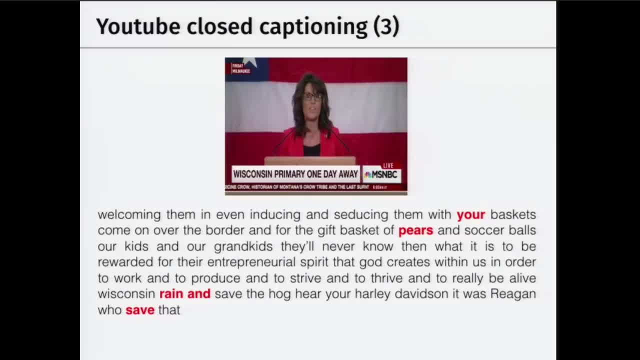 that entrepreneurial spirit that God creates within us in order to work and to produce And to strive and to thrive and to really be alive. Wisconsin: Reagan saved the hog. Here you're, Harley Davidson. That was Reagan who saved. Okay, so if I were to try and predict what the next word is, given her word context, 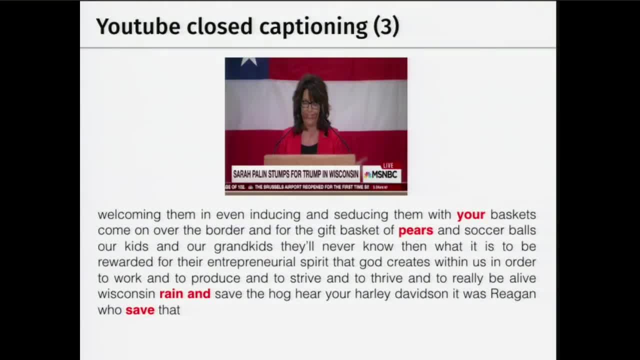 there's no way I could reproduce this, Because it's quite arbitrary, right? You have no idea what she's gonna say next. If you showed me that transcription, I would say: well, it's clearly mostly wrong. Nobody would actually say that. 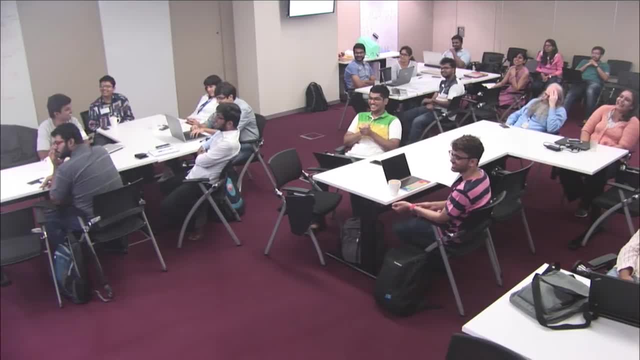 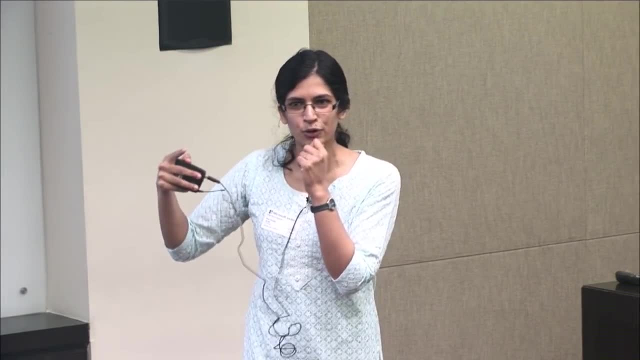 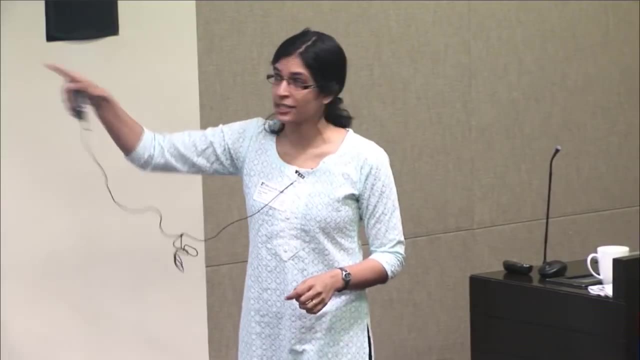 Yeah, so here, clearly, language model can only help so much, cuz this is really- it's quite arbitrary. She has a strong accent, but YouTube's ASR engines do have a lot of southern dialects in their training data. So at least- and she's also speaking to a large crowd in the open- 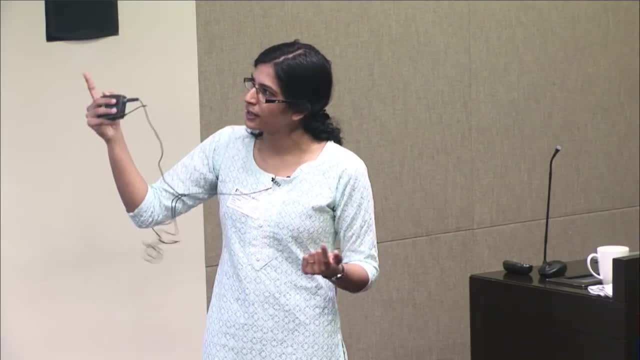 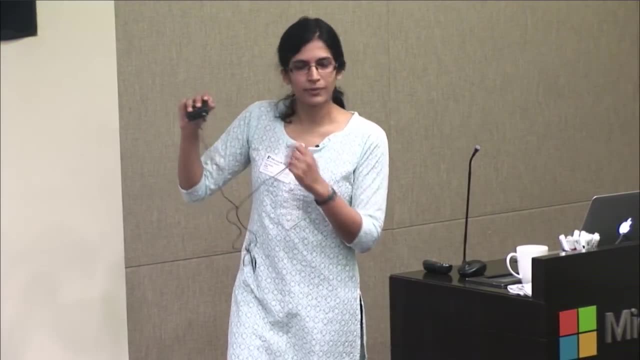 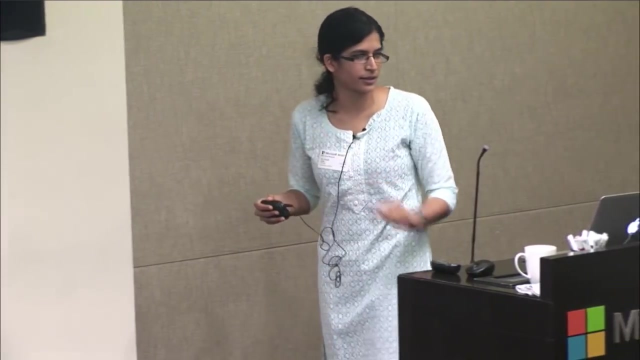 So the acoustic conditions are somewhat similar to the previous video, And the only difference is that the speaker in the previous video had a much more pronounced accent. So I'm not saying that it entirely had to do with the degradation in performance, but that certainly was a major factor in why the speech recognition engine didn't do as well. 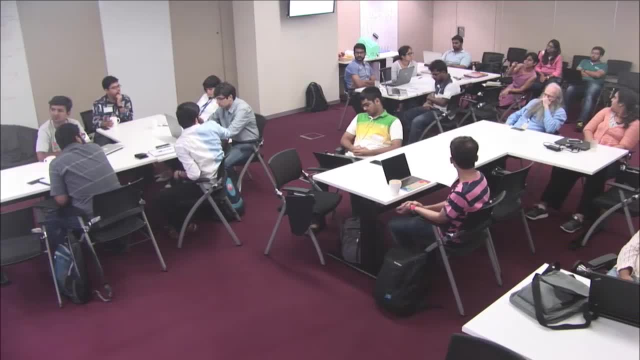 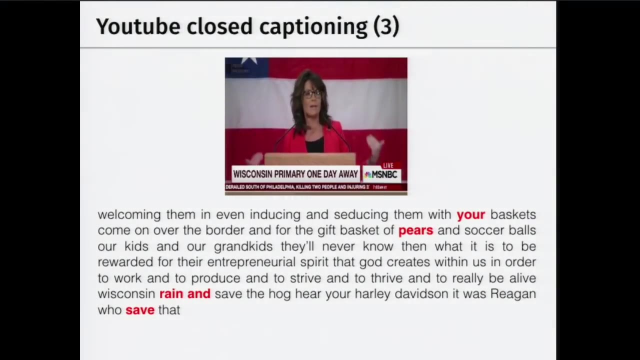 Yes, The second time it picked up correctly gift basket, but the first time it says your basket. So I think- Is that- Illegal immigrants, welcoming them in, even inducing and seducing them with gift baskets. Come on over to the border and-. 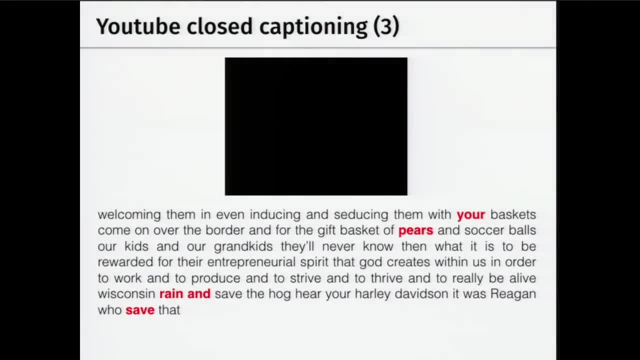 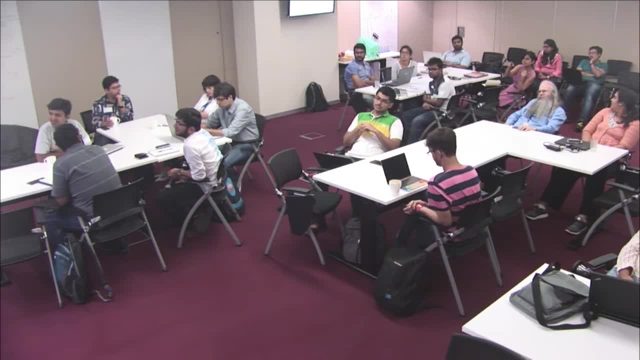 So what are you saying? It could not print for the first time that it's gift and it said your, but the next time it correctly identified-. I see, I see the second. yeah, yeah, So there are multiple things here at play. 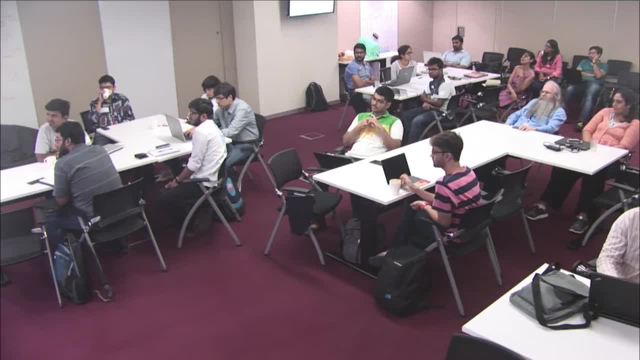 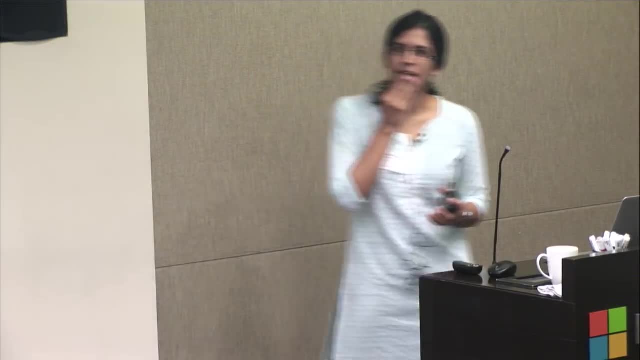 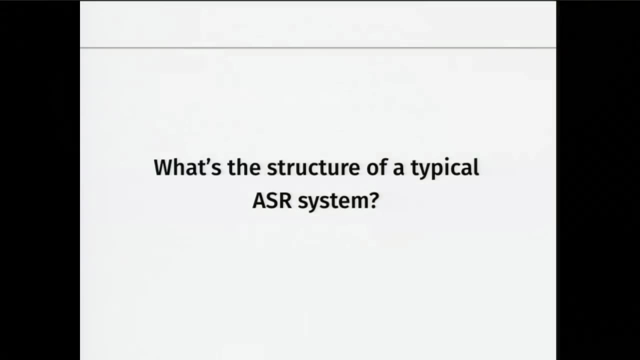 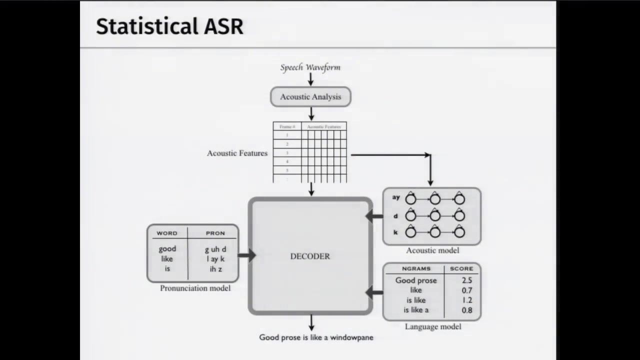 So maybe after I show the structure of an ASR system I can come back to this question. Any other questions so far? Okay, Okay. so let's actually move into what's the structure of a typical ASR system. So this is more or less the pipeline of what's typically in. 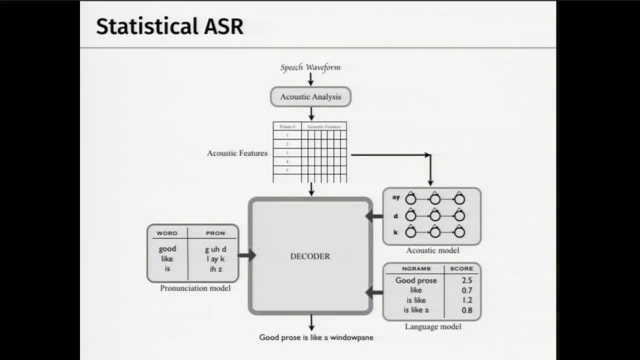 an ASR system. So you have an acoustic analysis component which sees the speech waveform and converts it into some discrete representation. There are features- if most of you are familiar with the term features- So the features are then fed into what's known as the acoustic model. 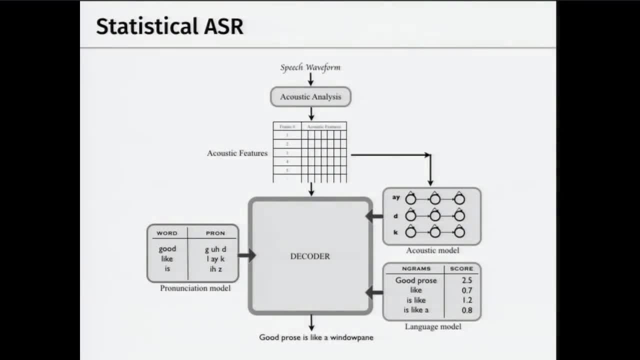 So actually, instead of explaining each of these components here, I'll kind of go into each of these individually and explain it more. So the very first component is just looking at the raw speech waveform and converting it into some representation which your algorithms can use. 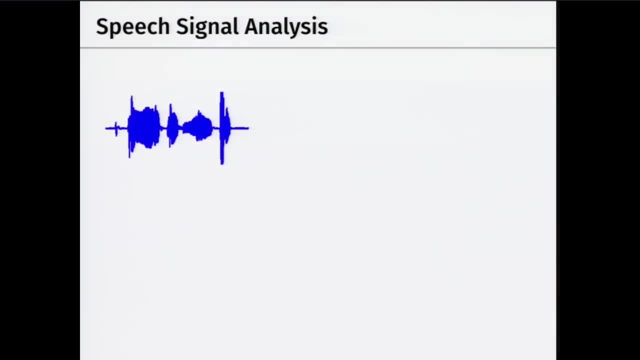 So this is just at a very, very high level. There's a lot of underlying machinery. I'm just giving you an overview of what's going on. So you have the raw speech signal, which then is discretized because you can't really work with this raw speech signal. 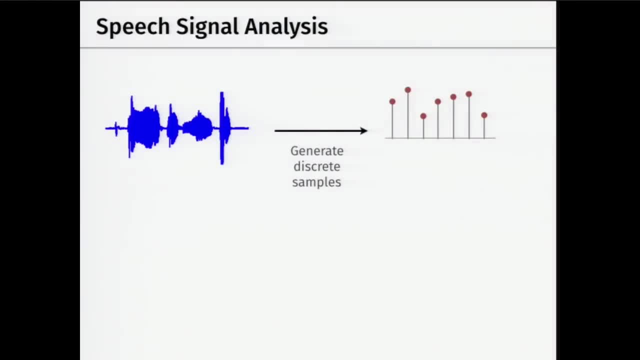 So you sample it and generate these discrete samples, And each of these samples are typically of the order of 10 to 25 milliseconds of speech, And the idea is that, once you have each of these, what are known as frames or speech frames- 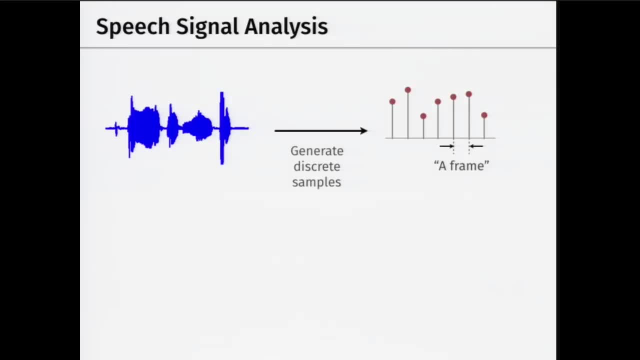 which are roughly around 25, sometimes even larger, but typically 25 milliseconds. Then you can extract acoustic features which are representative of all the information in your signal. And another reason why you discretize it at particular sampling rates is that the assumption is that within each 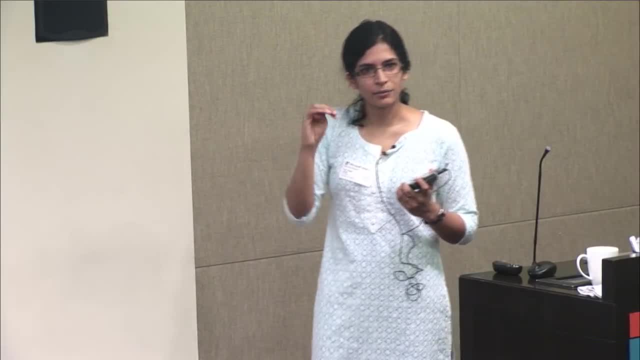 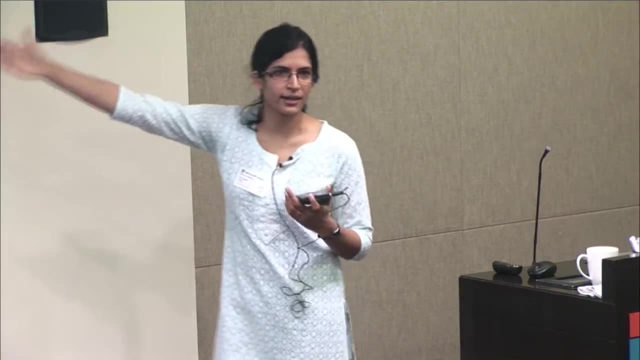 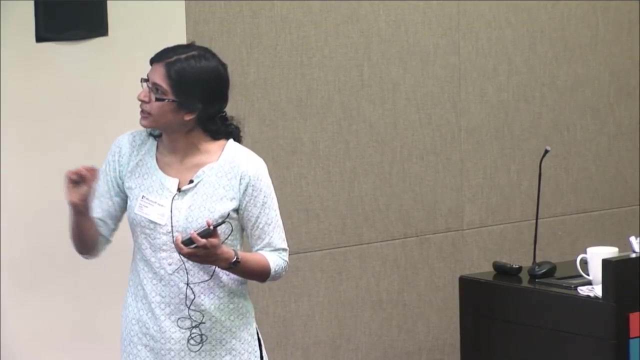 of these frames, your speech signal is stationary, And if the signal is not stationary within the speech frames, then there's going to be. you can't effectively extract features from that particular slice. So around 25 milliseconds of speech, yeah. So you extract features. 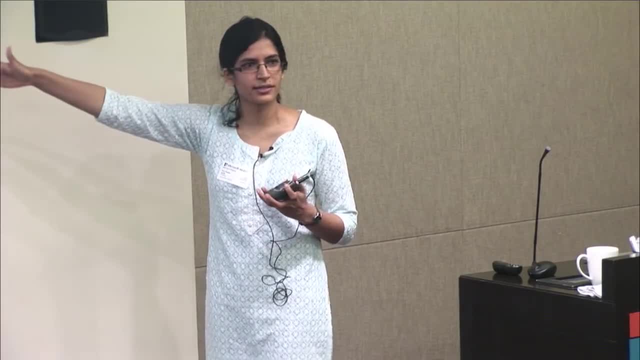 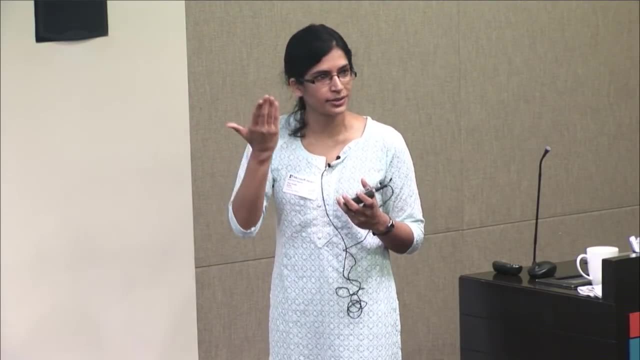 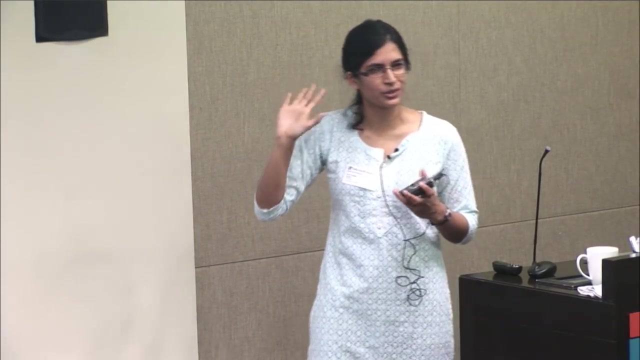 And this feature extraction is a very involved process and it requires a lot of signal processing know-how, But this is also kind of motivated by how our ears work. So actually, one of the most common acoustic feature representations, which are known as male frequency capstral coefficients or MFCCs- 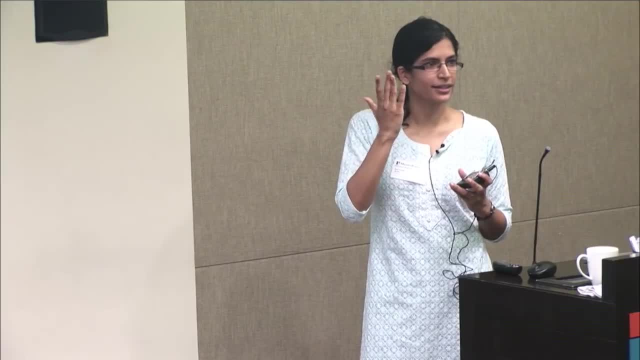 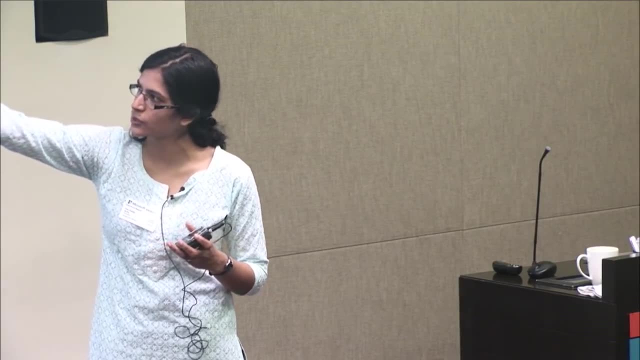 They're actually motivated by what goes on in your ear or the filter banks which apply in your ear. So that might be too much detail, so let's just think of it as follows. So you start with your raw speech waveform, You generate these tiny slices, which are also known as speech. 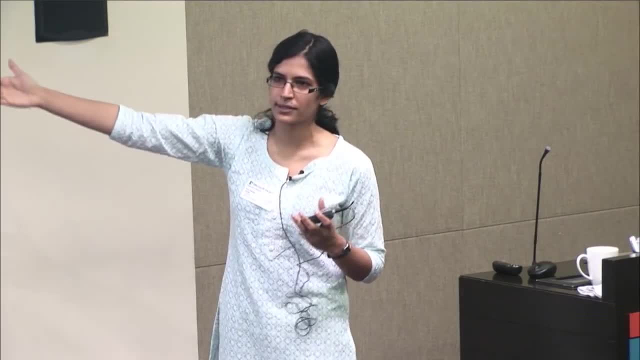 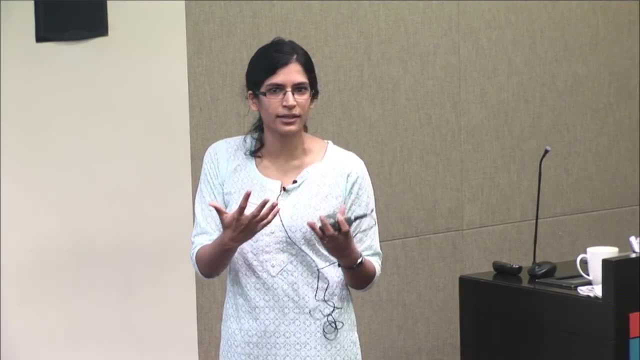 frames, And now each speech frame is going to be represented as some real valued vector of features Which is capturing all the information and as far as possible, is not redundant. So you don't have different dimensions here, which are redundant. So you want it to be as compact as possible. 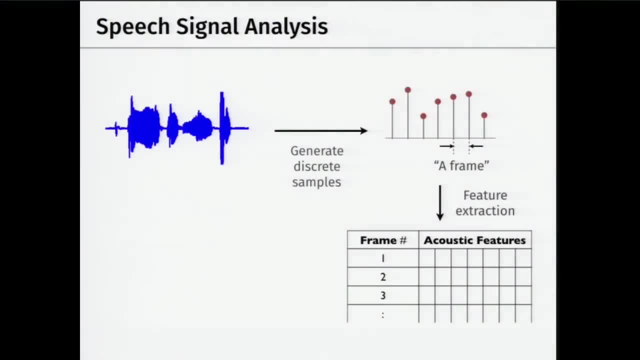 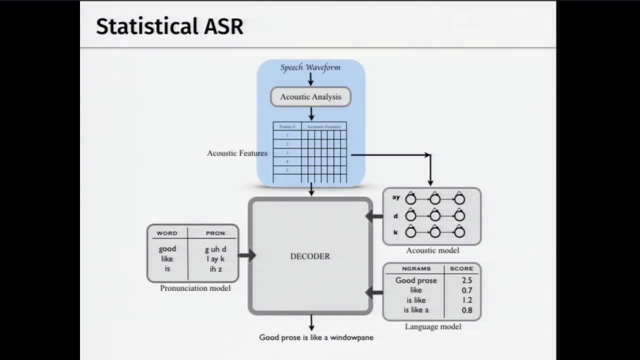 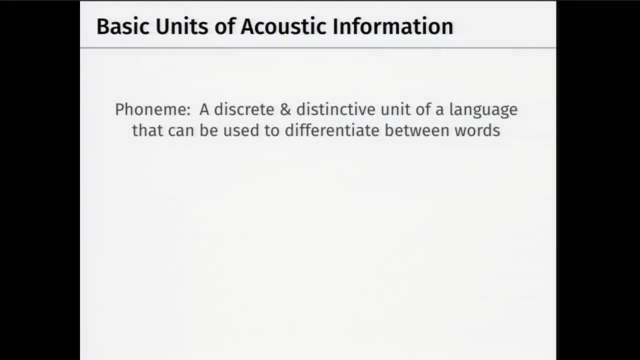 So now you have these features for each frame, And now these are your inputs to the next component in the ASR system, which is known as the acoustic model, And it's a very important component. So, before I go into what an acoustic model is for anyone, 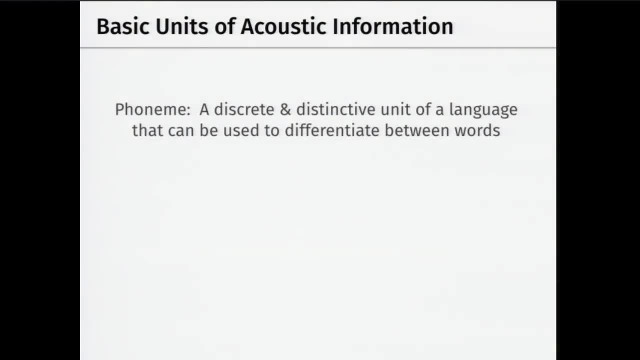 who's interested, probably in this crowd. everyone knows what a phone is because there's lots of linguists and many of you might have encountered it, But anyway. so a phone is just a discrete unit, or it's a speech sound in a language which can be used to. 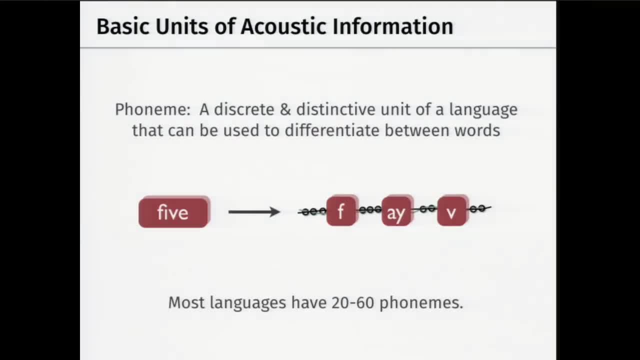 differentiate between words. So in ASR there is this approach which is known as beads on a string approach, And this is my terrible drawing of beads on a string. But you're, each word can be represented as a sequence of fonts, So five. here is a sequence of three of these speech sounds. 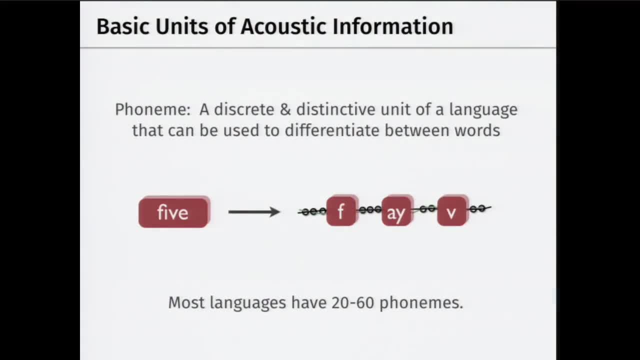 So the phone alphabet is very much like the alphabet for our languages. so in text, Except now, it's covering the sound space rather than the textual space. So phones are just the letter equal. the analogy of phones is letters in your written texts. 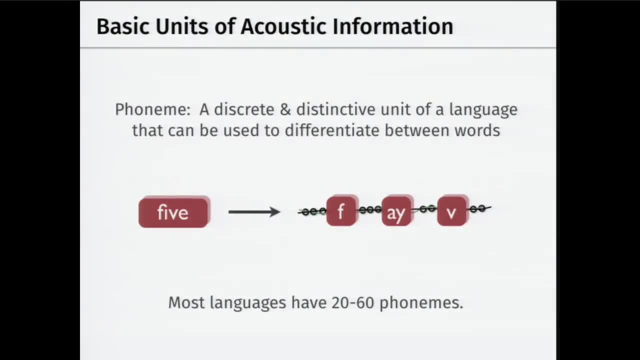 And each word can be represented as a sequence of fonts. So this mapping- so you might be wondering how do you know that five actually maps to this sequence of fonts? This is written down by experts in the language. So this particular mapping between the pronunciation of 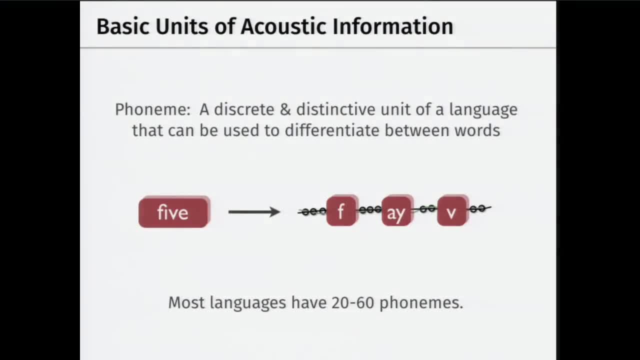 a word. so this is actually giving you how this particular word is pronounced, Because you know how each individual phone is pronounced And this pronunciation information is actually given to us by experts. So in English, of course, we have very well developed pronunciation dictionaries. 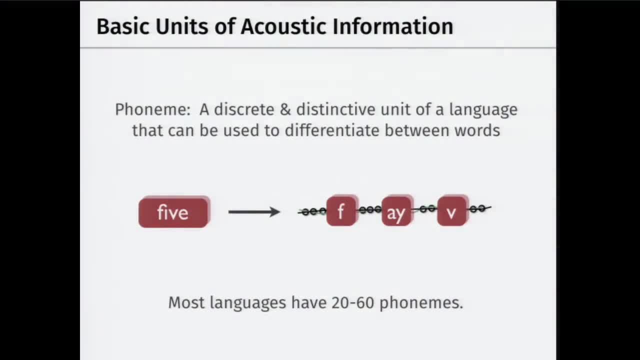 Where experts have given us pronunciations corresponding to most of the commonly occurring words in English, And actually we have CMU to thank for that. So one of the most popularly used pronunciation dictionaries in English is CMU Dict, which is freely available. 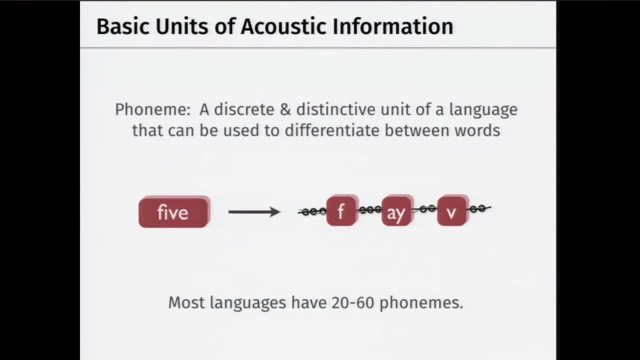 And it has around 150,000 words, I think, yeah, of that order, And that is actually one of the more extensive dictionaries. So typically you don't get. this is not a very easy resource to create, and it's clear why: because it's pretty tedious. 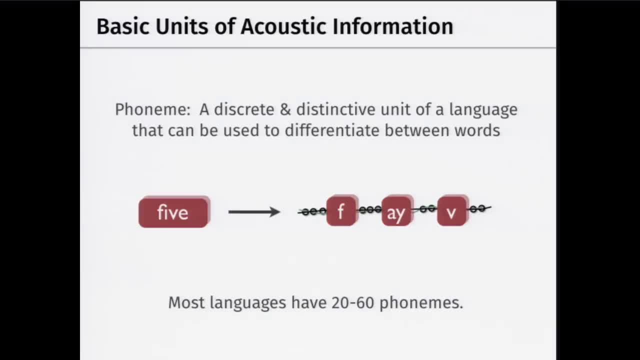 First of all you need to find linguistic experts in the language, and then you need to find what are the most commonly occurring words in the language, and so on. So this takes time and not many languages have very well developed pronunciation dictionaries. 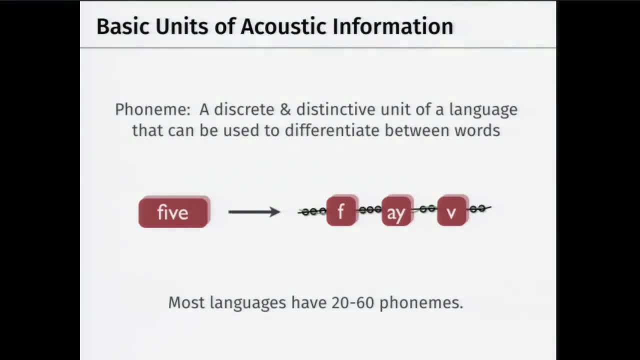 And most languages have around 20 to 60 phonemes. So the phoneme inventory size is roughly 20 to 60. And this is also something which needs to be determined by experts. What are the phonemes which are applicable to a language? 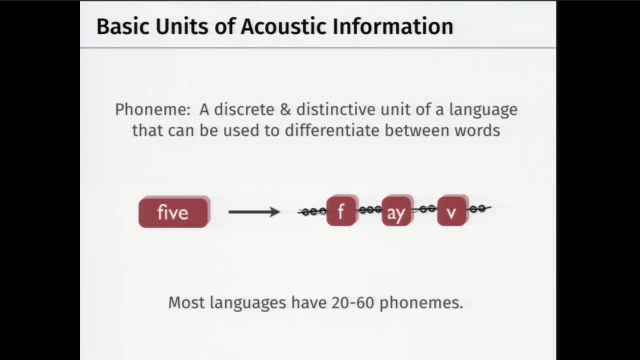 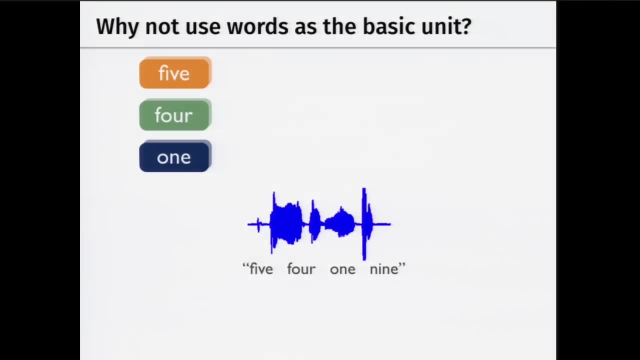 So this is a very language dependent characterization. What are the phonemes which are relevant to a particular language? Okay, so, given we have these units, okay, so one more slide Just to motivate. why do we need phones, even from a modeling? 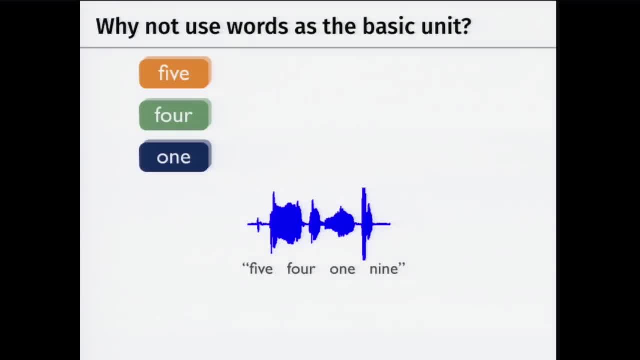 standpoint, So not just from the linguistic standpoint which is each of these. These sounds can be kind of discretized in terms of these phones, But even from a modeling standpoint, why are phonemes useful? Why not just use words instead of trying to split it into these? 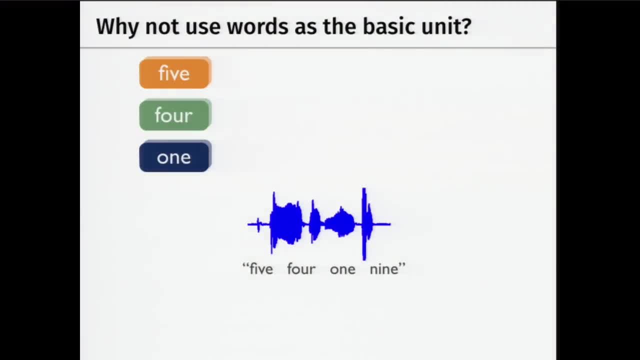 subword units. So let's look at a very simple example. So say that your speech waveform is this string of digits, 5419.. And say that during training you've seen lots and lots of samples of five, four and one. 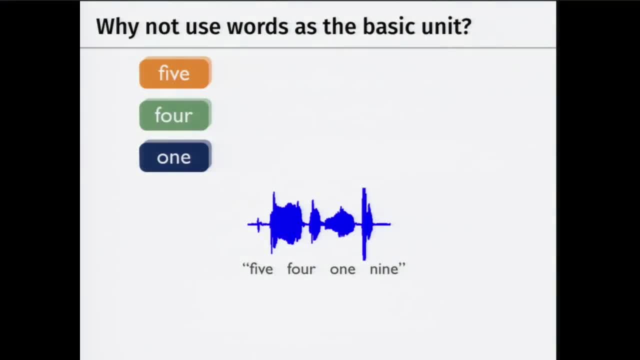 So now you can build models to identify when something is five and when someone said five, and when someone said four and when someone said one, But when you come to nine, so this is say during test time, when you're evaluating this particular speech utterance. 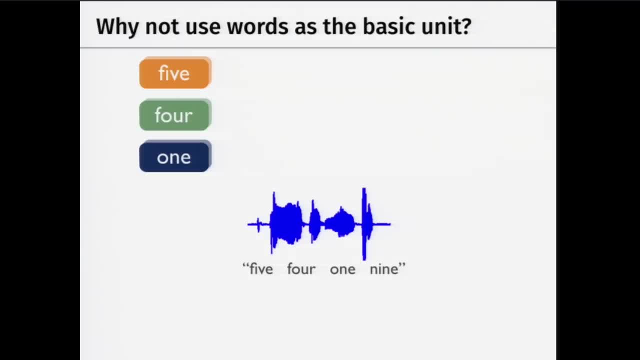 What do you do then if during training, you've never seen nine? Of course this is not reasonable here, because it's a very small vocabulary, but you can extrapolate when you move to larger vocabularies, right? So yeah, all of these words exist, but 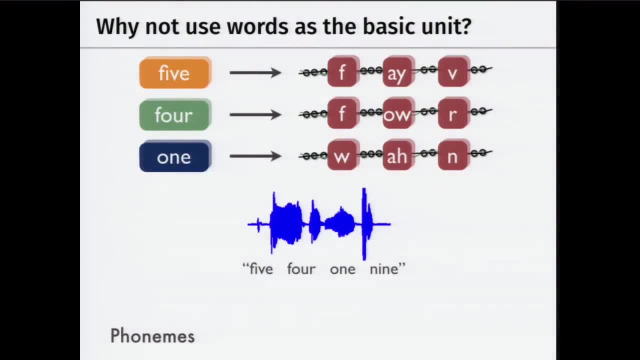 what do you do when you come here? What if we were to represent each of these words as their corresponding sequences of forms? So now, five is this sequence of phonemes. four: is this sequence of phonemes, one is this sequence of phonemes, and so on. 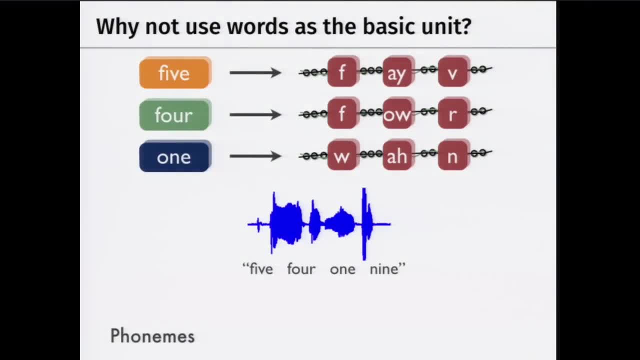 And now you've seen acoustic speech samples which correspond to each of these phonemes in your training. So during test time, when you see nine, you might be able to put together this string of phonemes because you've seen enough acoustic evidence for each of these individual phonemes. 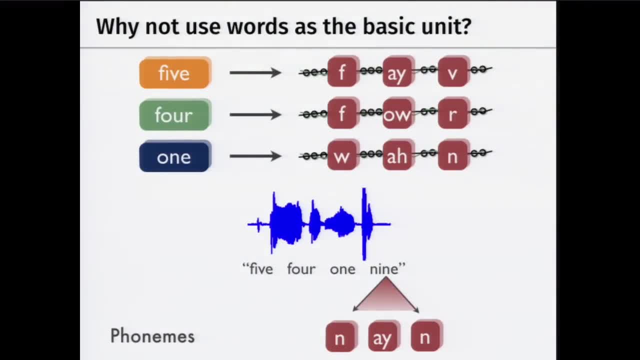 Is that clear. So it helps you generalize, just to move to a more fine grained inventory. But of course, that said, if you have a very limited vocabulary task and if you're likely to say that you're almost certain that during test time you're only going to get utterances which 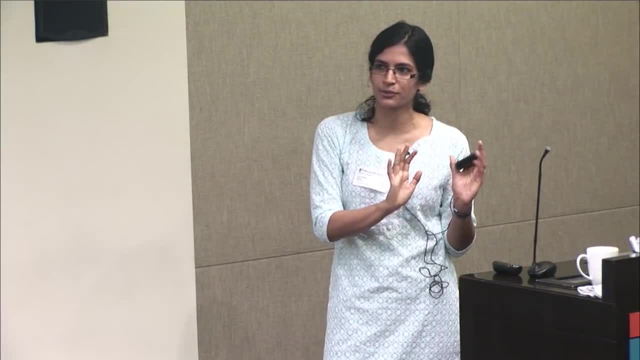 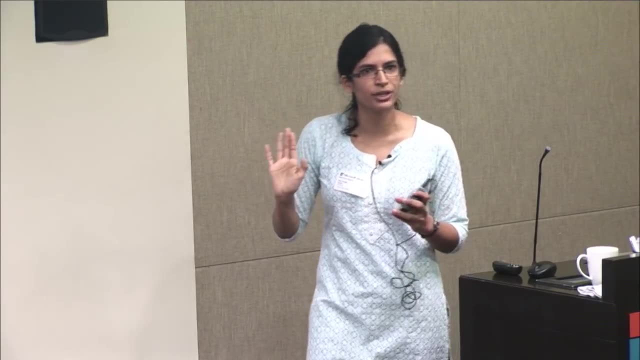 are going to stick to that particular vocabulary And if you have enough samples during training, you're probably well off just building word level models and not even moving to the phone level. But that is for very limited tasks. So most tasks you want to do this. 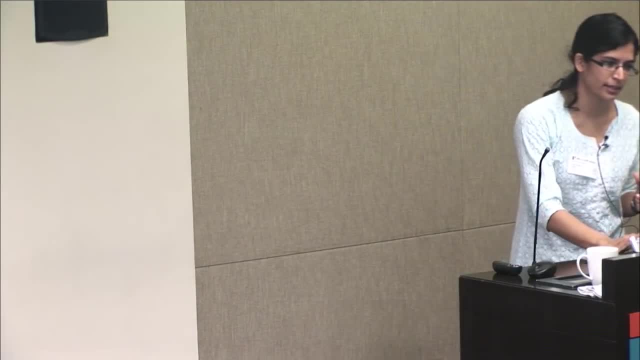 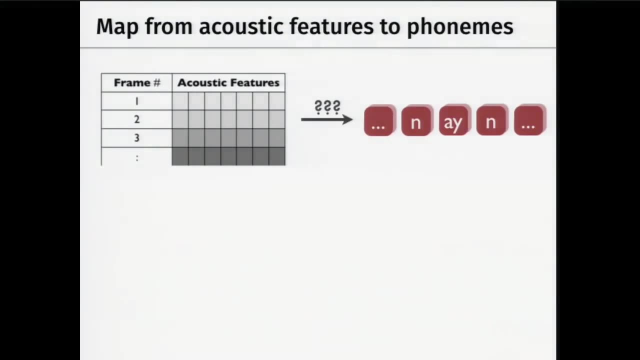 So you want to move to this slightly more fine grained representation? Okay, so that hopefully motivates why we need phonemes. So this is the problem, right. So I mentioned you have acoustic features which you extract from your raw speech signal. 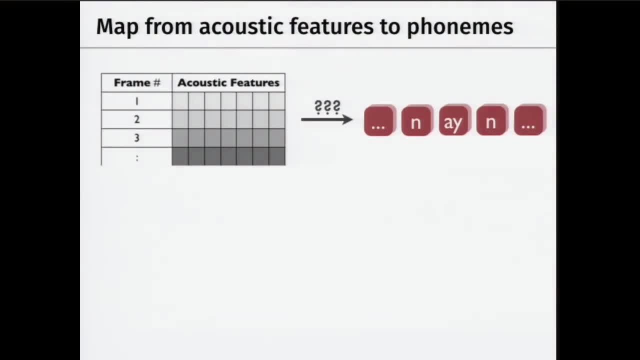 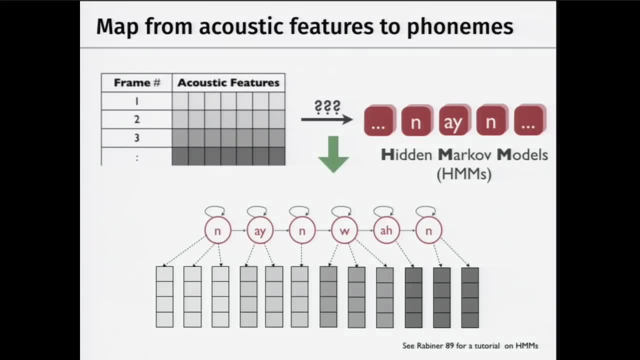 And you want the output from this acoustic model to be what is a likely phone sequence which corresponded to this particular speech utterance. So this model is typically so initially in the 80s and even now, actually hidden Markov models is a paradigm which is 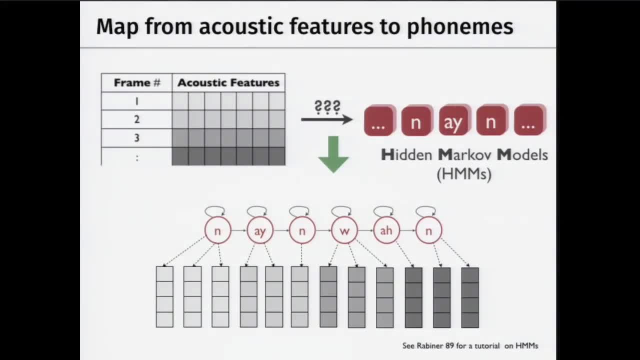 used to learn this mapping. So how do I associate a set of frames, a set of features? So when I say frames and features, they are kind of interchangeable, right? So each of these acoustic feature vectors corresponds to a speech frame. So how do I chunk how many frames are going to correspond? 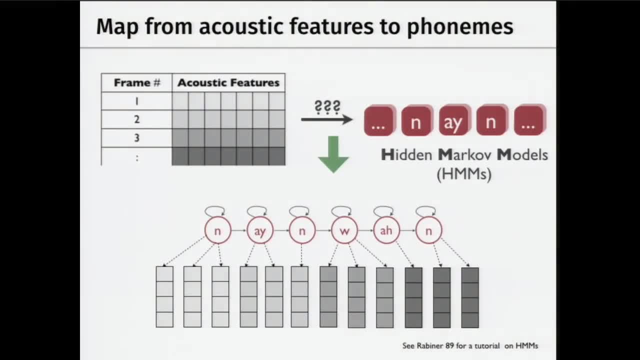 to a particular phone And here. so I've shown you a chain of what are known as hidden states in your hidden Markov model And all the so this is just like. think of it as a graph, And it's a weighted graph. 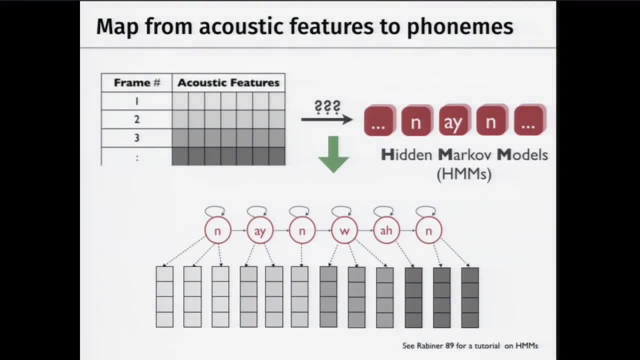 So here I've not put weights on the arcs, But the weights are all probabilities. So another thing is here. I've just shown you a single chain that is just a sequence of these phones And it's put together. But you never know that right. 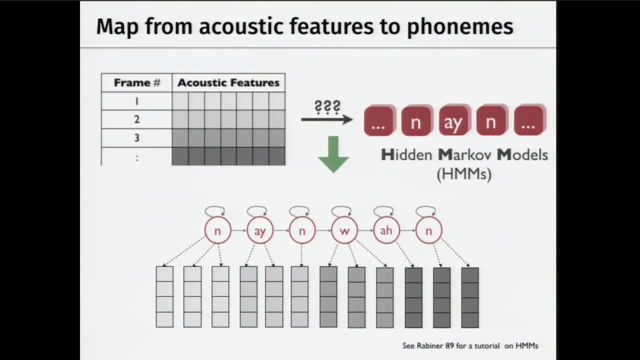 So at each point you can transition to any phone, because you don't know which phone is going to appear next. So the entire model is probabilistic, So you need to have lots of hypothesis as to what the next phone could have been. 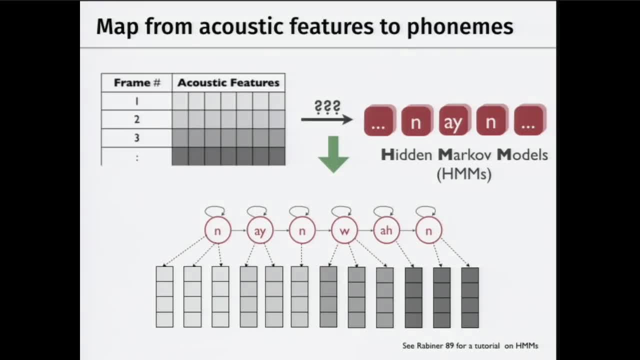 So here I've obviously simplified it by just showing a single chain, And then you have estimates which say that, okay, I think this initial ten frames most likely corresponds to a certain phone, And the transition probabilities, the probabilities which transition from one phone state to the other. 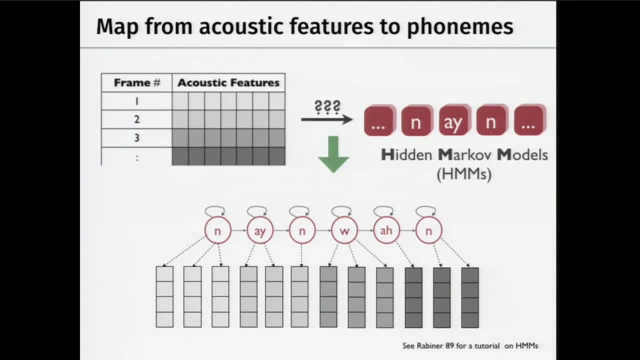 determine how many are going to chunk, how many speech frames are going to correspond to each phone, And once you're in a particular state, there are probabilities for having generated each of these vectors. So once I'm in, say this state, there's a probability for. 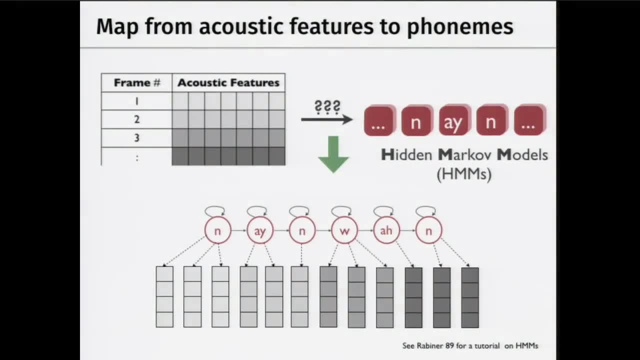 having seen this vector, given that I'm in this state, And those probabilities come from what are known as Gaussian mixture models, So it's a probability distribution which determines that. okay, once I'm in this particular state, this particular speech vector could be generated with. 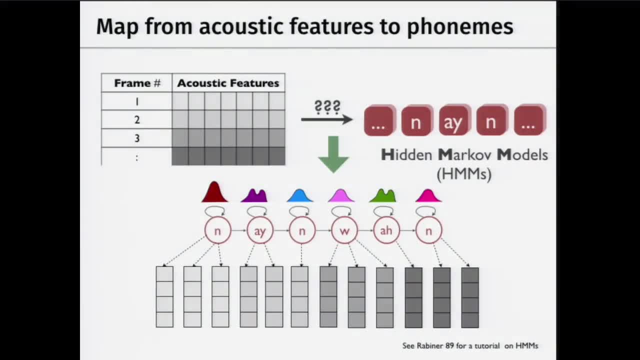 a certain probability, And how are these probabilities learned from training data? So that is the detail I'm not going to go into. yeah, Yeah, this is just the acoustic vector, That's it. yeah, So any questions so far? Okay, so this is. I've obviously glossed over lots and 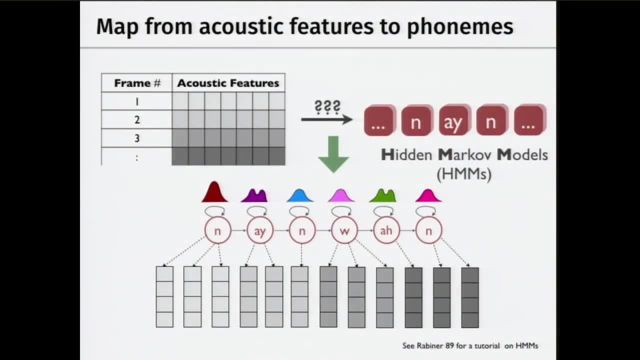 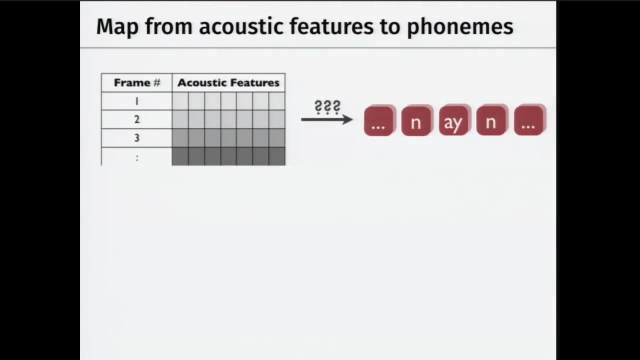 lots of details, But this is just to give you a high level idea of you have a probabilistic model which maps sequences of feature vectors to a sequence of forms. okay, So hidden Markov models were the state of the art for a long time. 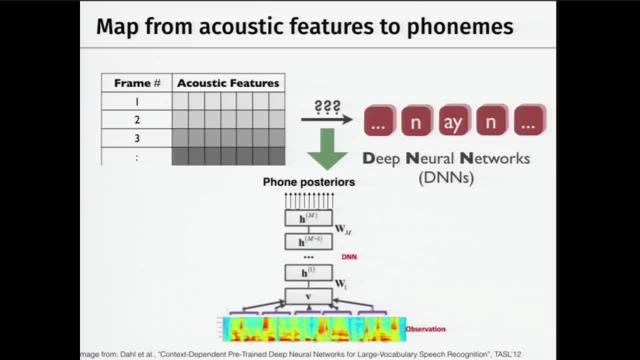 And now of course, we have deep neural networks for a similar mapping. So now you have your speech signal and again you're extracting fixed windows of speech frames And from these. so say that you're only considering a speech frame here, and then you have: I have a laser pointer, yeah. 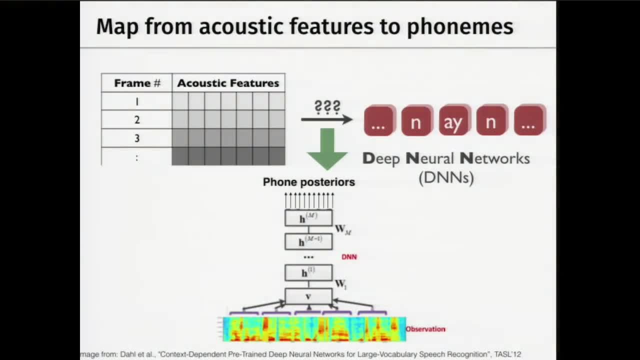 So say, you're considering a speech frame here, and then you look at a fixed window around it, a fixed window of frames around it, And you generate, you put all of these features together And that is your input to a deep neural network. 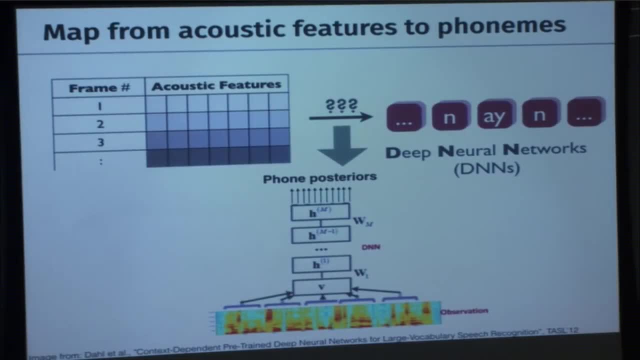 And the output is what is the most likely phone to have been produced given this particular set of speech frames. But this is a posterior probability over the phones, So I'm not going to go into details about what this is. But again, here you get an estimate of what is the phone. 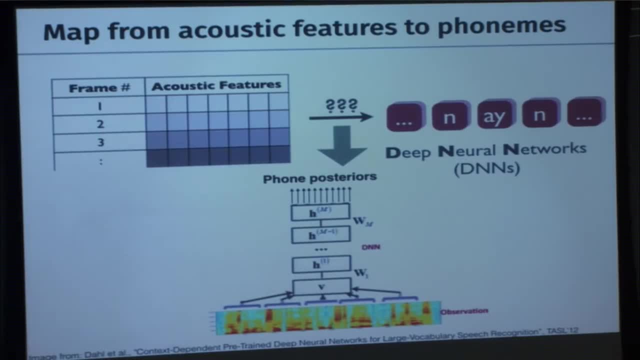 given a speech frame, what is the most likely phone? So this is the probability distribution over all the phones And there are two ways in typically how DNNs are used in acoustic models, So one is in the previous slide I mentioned. 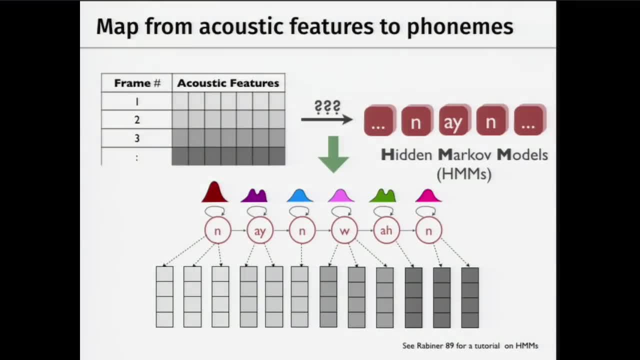 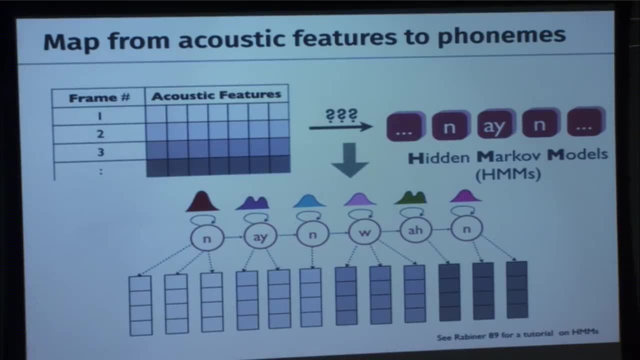 when you have HMMs, you have these states and then you have these probability distributions which govern how the speech vectors correspond to particular states. And these probability distributions are mixtures of Gaussians. But you could kind of not use mixtures of Gaussians here. 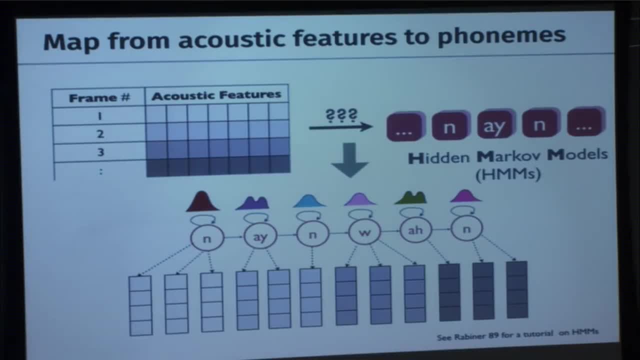 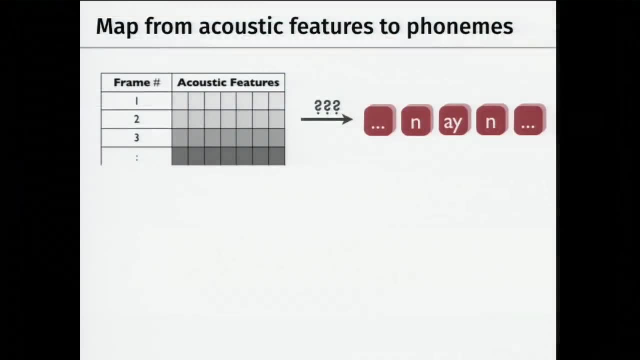 and instead use probabilities from your DNN. So that is one way in which the DNN and the HMM models can be combined and used within an acoustic model. So please feel free to stop and ask me any question. So at this point I'm not really clear if I'm going too technical. 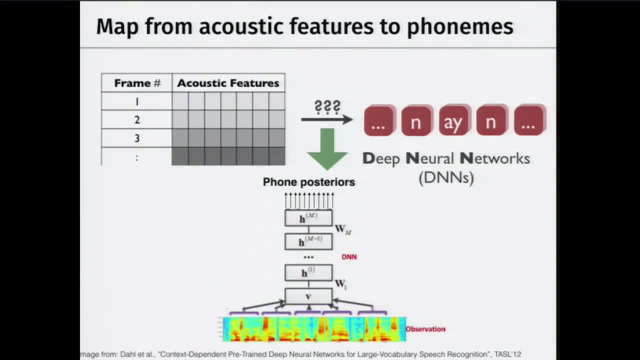 or so. please feel free to interrupt at any point. So this is so. the idea is that we want to map acoustic features to phone sequences and this is all probabilistic, So we are not giving you a one best sequence, We are saying this is the likely probability distribution of 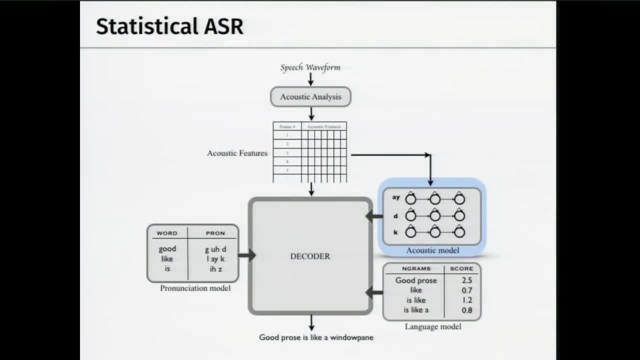 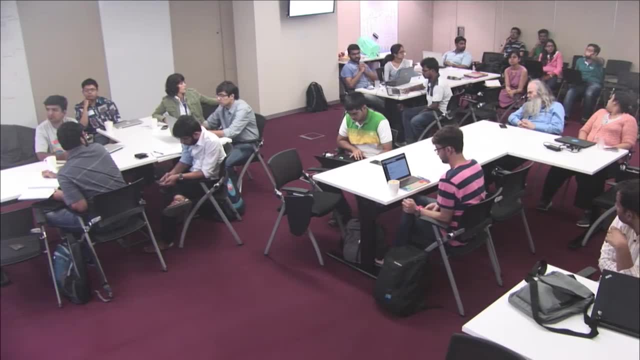 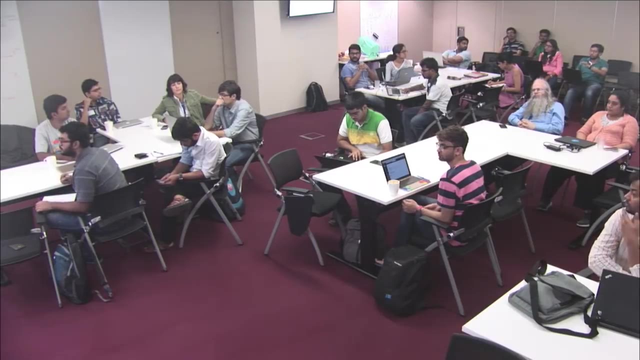 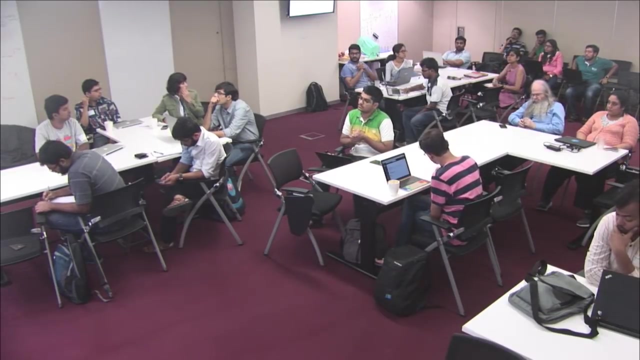 phone sequences. Okay, so that is the output from our acoustic model. Yes, Yeah, Yeah, Yes, exactly The observations of the acoustic features. and then you have probability distributions. How is so the probability distribution for the? so you're familiar with HMMs. 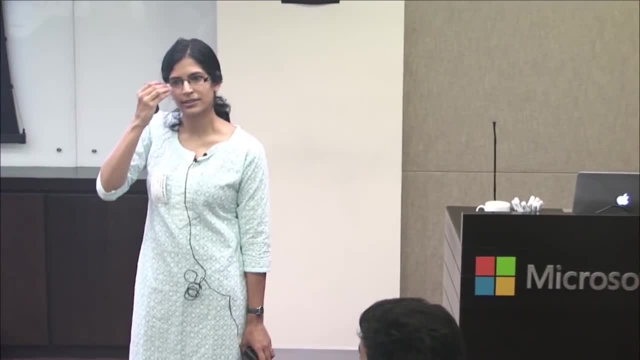 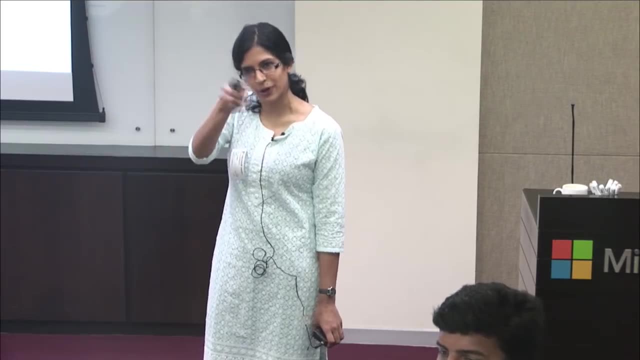 So you have observation probabilities. So your observation probabilities, either they can be Gaussian mixture models or your observation properties can be scaled posteriors from your DNNs. So it's just the probability distribution. your observation probability distribution can come from the DNN. 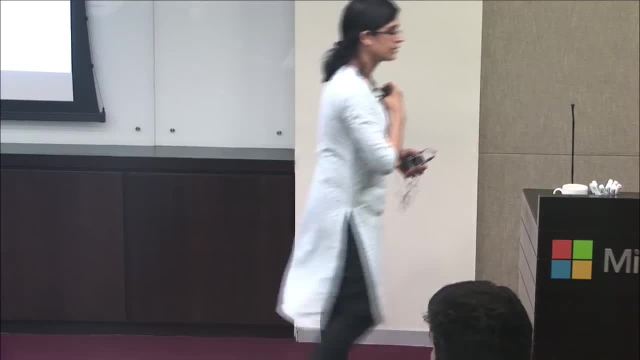 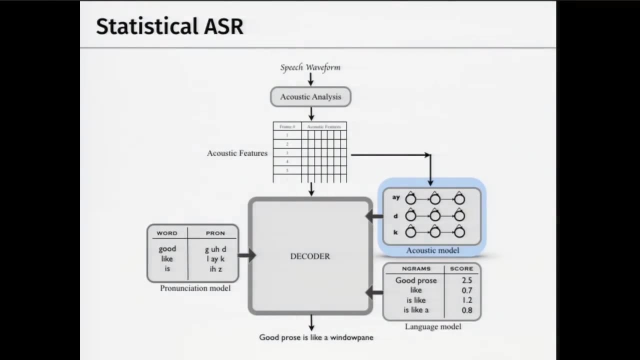 Yeah, Okay, so this is the acoustic model which produces phone sequences. So now we eventually want to get a word sequence right from the speech utterance. So this is just an intermediate representation, these phones. So now, how do I move from the phones to words? 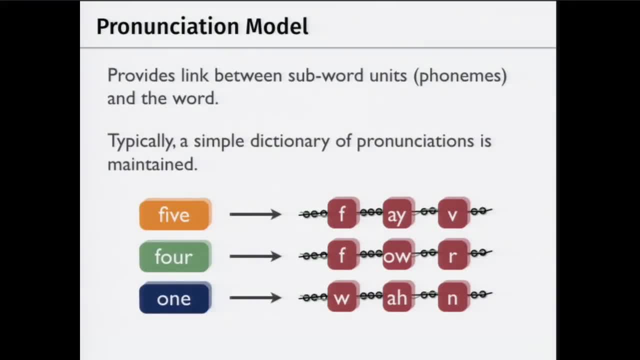 So I mentioned, we use these large pronunciation dictionaries. So this is the model which provides a link between these phone sequences and words. So here, typically, just a simple dictionary of words is maintained. So you have these large dictionaries which say that these words correspond to these sequences of phones. 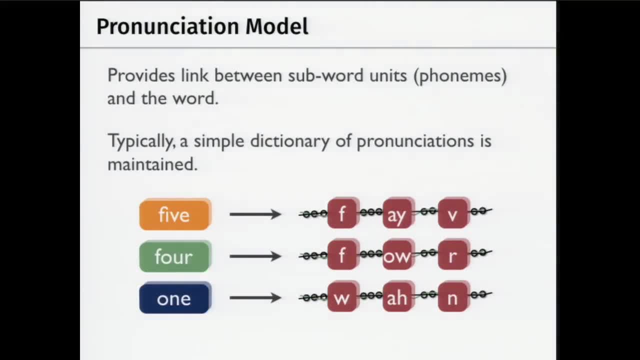 And this is the only module in an ASR system that is not learned. It's not learned from data. So the acoustic model was learned from training data And we'll come to the language model. that is also learned from data, but the pronunciation model is actually expert derived. 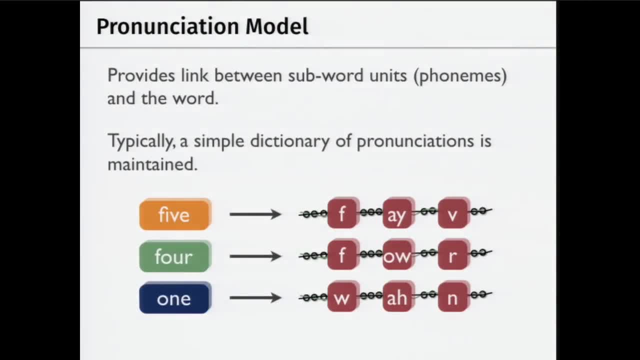 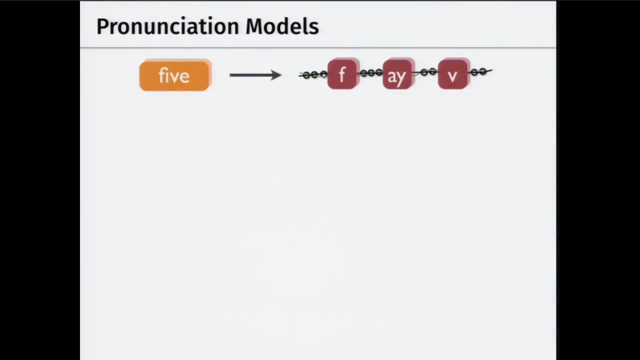 So an expert gives you these mappings. So I'll talk a little about some work I did during my thesis, which was on pronunciation models, And it's kind of hinting at how restricted this particular representation is. So I mentioned that each word can be represented as a sequence. 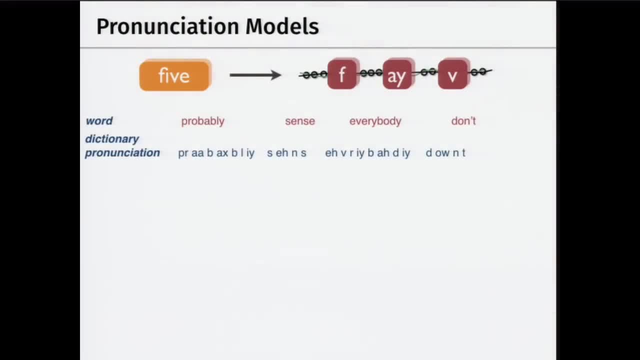 of phonemes. So we looked at a very popular speech corpus called switchboard, a subset of switchboard Which is very, very it's annotated at very detailed level. So not only do we have word sequences corresponding to the speech, we also have phonetic sequences. 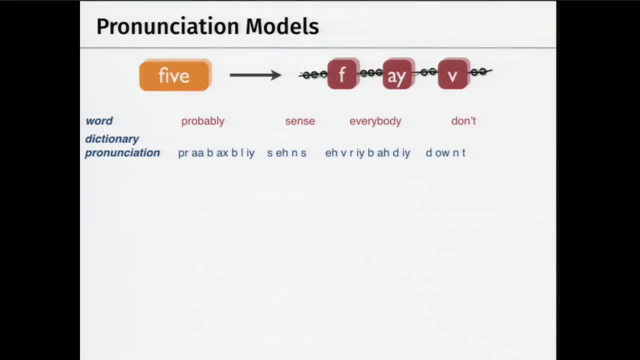 So it's also phonetically transcribed Meaning: someone listened to all of the utterances and wrote down the phone sequence corresponding to what they heard. And this was obviously done by linguists. And when I say phone, they actually listened to how the word was pronounced. 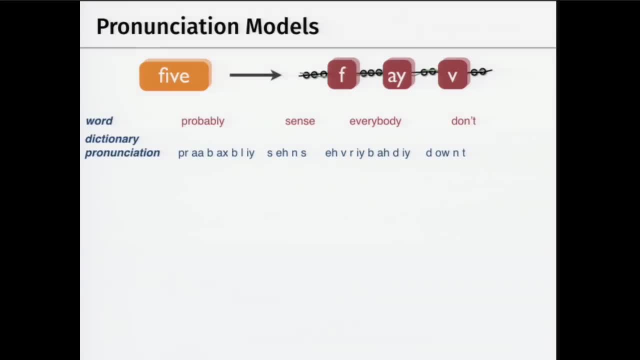 not what the word should have been according to some dictionary. And why I'm saying this is because there's a lot of pronunciation variation when you actually speak. So certain words, even though the dictionary says that it should be pronounced a certain way, because of our accents or 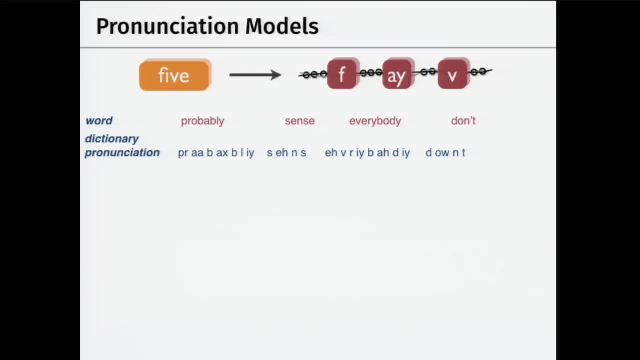 just because you're talking fast and so on, The word actually ends up being pronounced in an entirely different way. So for some data from this corpus, we actually had phonetic transcriptions which are giving us exactly how people pronounce those words. So if you one thing that really stands out from the data. so 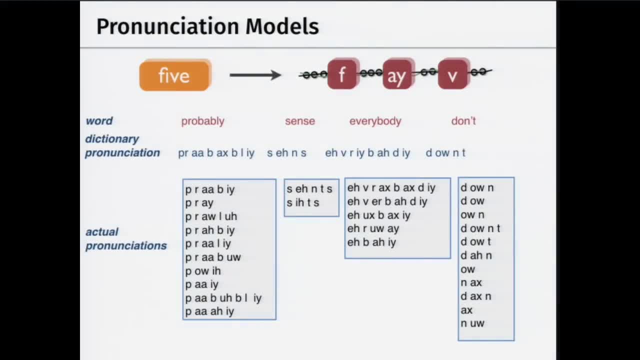 let's look at just four words, So this is probably sense everybody and don't. And the row in blue are the phone sequences corresponding to these words according to a dictionary. So this is how the word should be pronounced according to an American. so this is the American pronunciations. 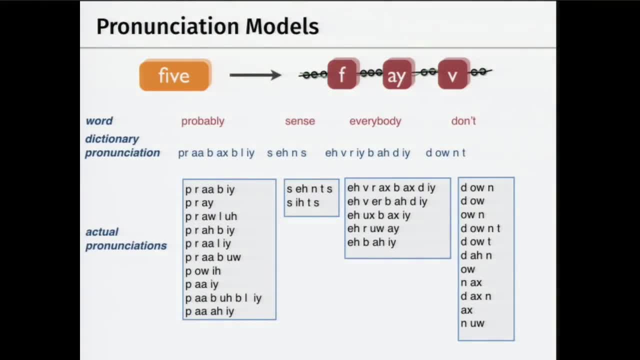 And these were the actual pronunciations from the data as transcribed by a linguist. So, obviously, what is the first thing that stands out here? There's no one. Yeah, definitely There's no one pronunciation corresponding to the word. 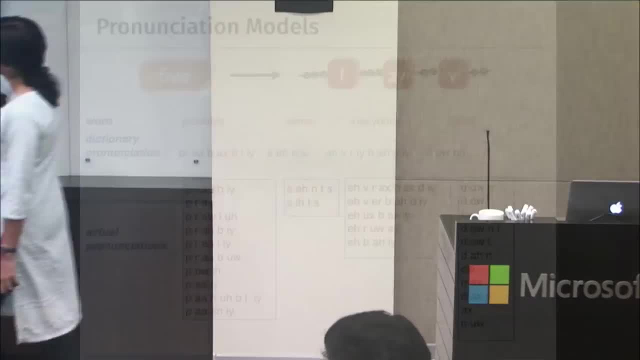 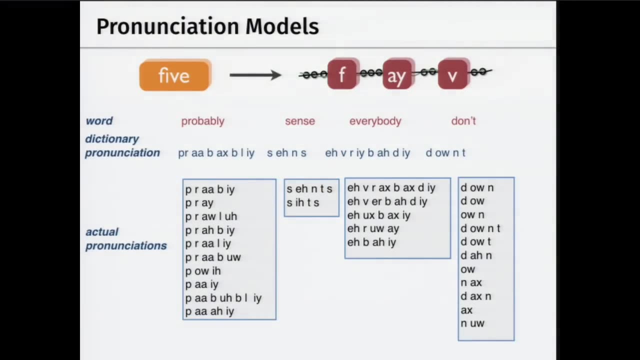 There are lots of possible pronunciations And you'll also see this is. you'll see lots of entire syllables are being dropped out of words. So, yeah, it's being very fast. It's wrong, but it's completely legible from the speech. 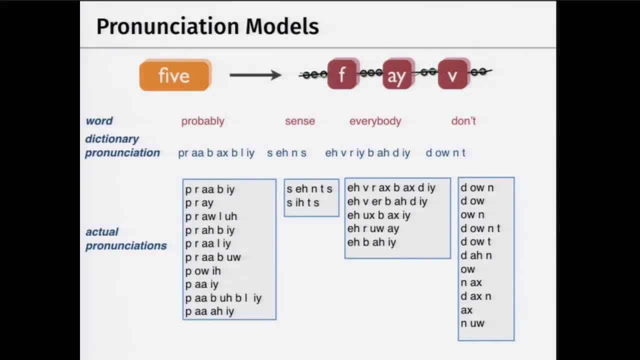 I mean just because of the context and so on, But they're speaking very fast. So if you actually look at the phonetic transcription, there are entire syllables missing And of course these are also perfectly legitimate pronunciations, right? 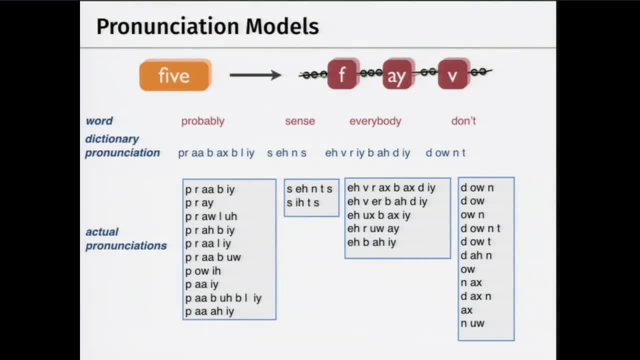 So sense when you say the word it almost feels like you're inserting a at the end before the last sound sense. So there are lots of alternate pronunciations for words And I don't remember the exact number but I think the average number of pronunciations they found for 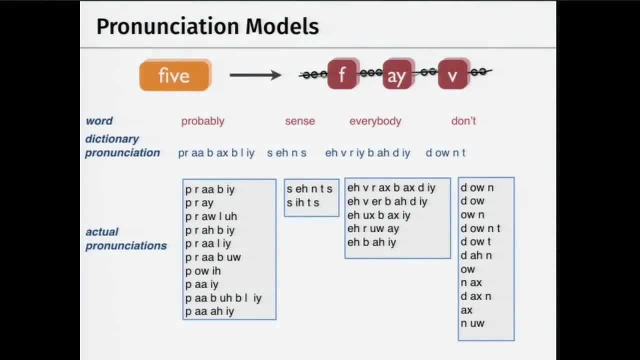 a word was of the order of four or five, So very far from a single pronunciation. Okay, so we thought, why not? So clearly there's a lot of pronunciation variation, And this was from a corpus which was of conversational speech. 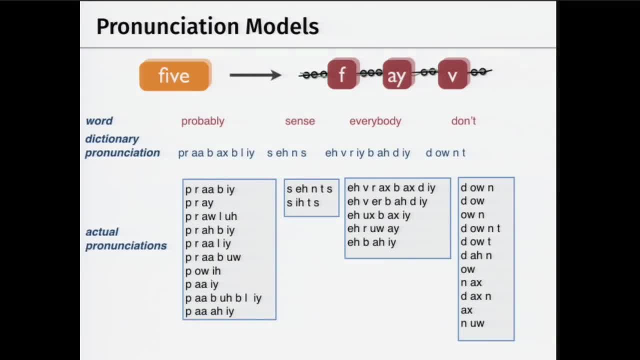 So it's not read speech, where people are speaking very fast and so on. Read speech tends to be more clear and they enunciate and they tend to stick more to the dictionary pronunciations. But of course you want to recognize conversational speech. 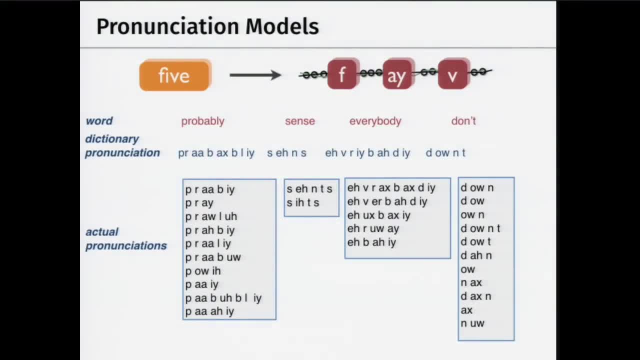 You're not always only going to recognize news broadcasters, You need to recognize spontaneous, day-to-day speech. So how do we connect? So how do we kind of try and model this pronunciation variation, How do we computationally model this? And so we thought, why not go to the source? 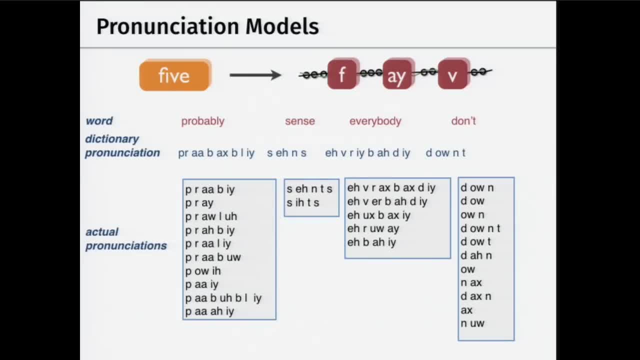 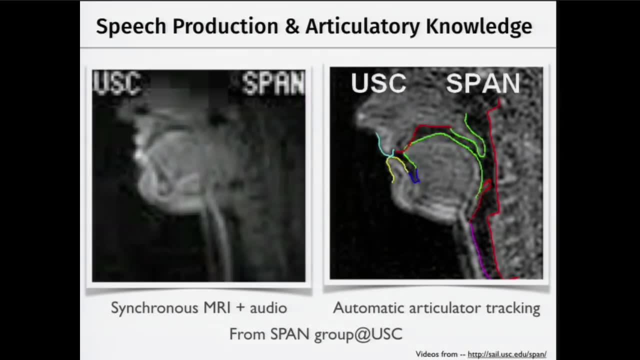 So what is creating these pronunciation variations? So it's your speech production system. So there are various. so before going into that, I'll show you these videos from the SPAN group at USC, which is led by Sreenarayanan. 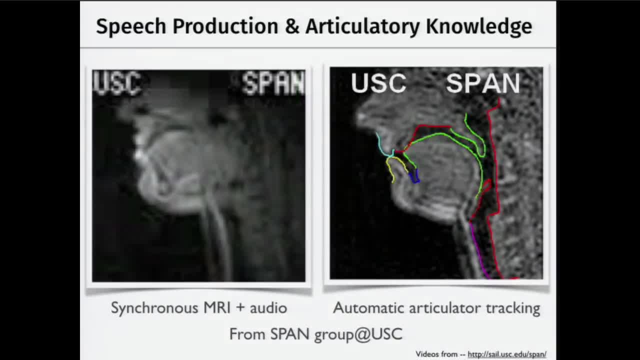 And they do really good work on speech production based models to model pronunciation variation and so on. So this is an MRI of the vocal tract And it's synced with the audio. so When it comes to singing, I love to sing French art songs. 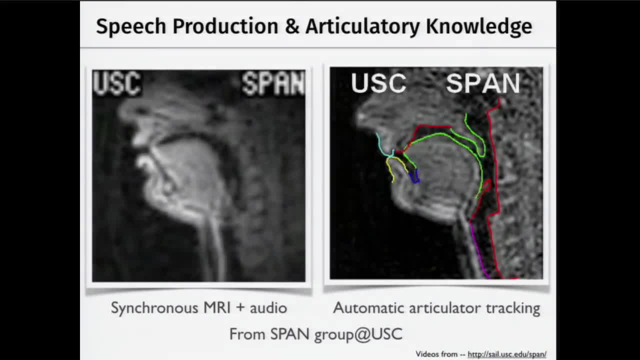 It's probably my favorite type of song to sing. I'm a big fan of Debussy, I mean, I also love operas, I love singing, and Mozart and Strauss. But when I listen to music, I tend to listen to hard rock or 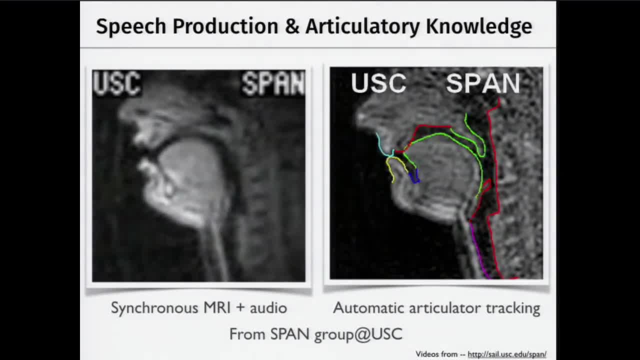 classic rock music, And one of my favorite bands is ACDC, And my favorite song is probably Back in Black, which I'll listen to over and over again in my room. Okay, so these various parts of the vocal tract which are moving are known as articulators. 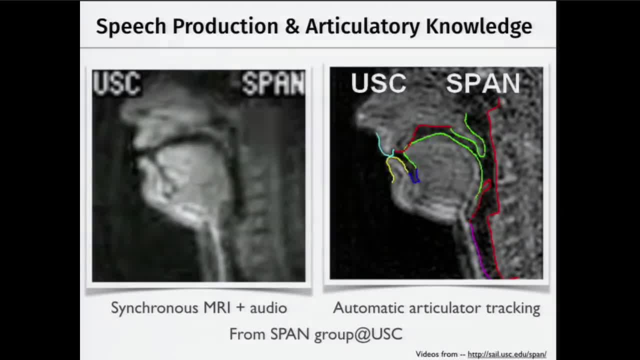 And the articulators move in various configurations and lead to certain speech sounds being produced. So they did some really cool work on actually- These are the movements that shape the speech sounds, Tracking the articulators automatically. This is really cool, So we didn't actually use these continuous contours. 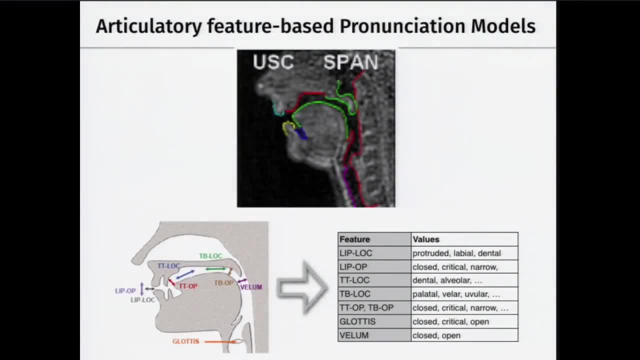 But we said: let's discretize the space. So there are these various articulators which move and there are various configurations of these articulators which lead to various speech sounds being produced. So if we can discretize the space and say that, okay. 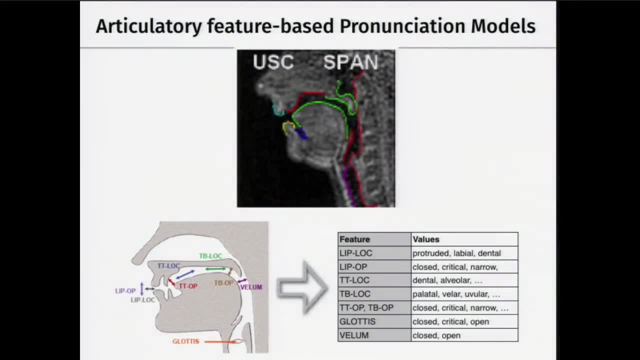 there are eight vocal tract variables And each of these variables can take one of n values. Then different value assignments to these tract variables can lead to different sounds. And this didn't just come out of the blue. there's a lot of linguistic analysis on speech production. 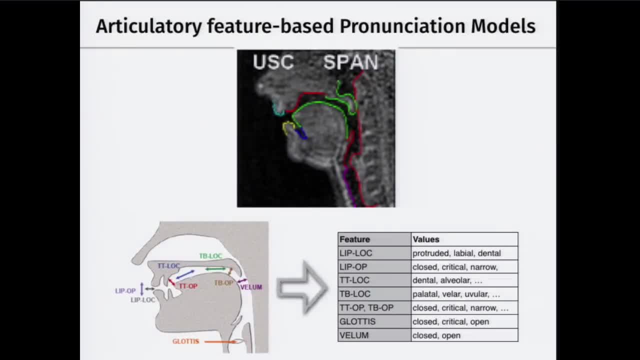 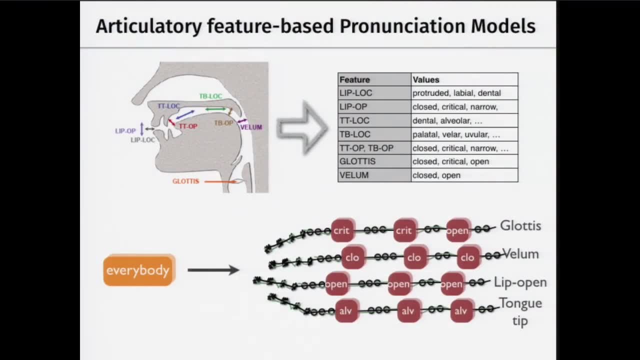 And there are lots of very well developed linguistic theories on speech production And we used one of them which is known as articulatory phonology. So I'll come to that in a single slide. So now everybody which used to be the sequence of phones. 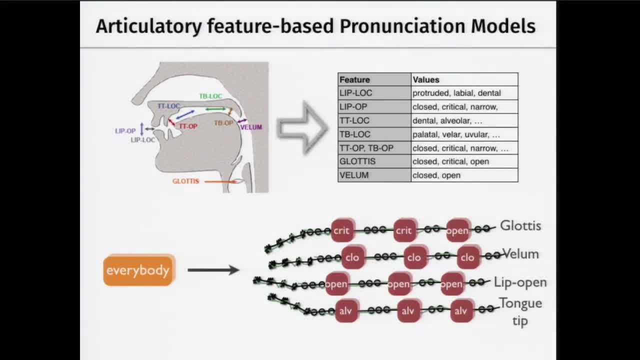 can now be represented as these streams of articulatory features. So if you have each variable which takes different values, now you'll have these quasi-overlapping streams of articulatory features which lead to a particular word and how it's being pronounced. And so why do I say they're overlapping? 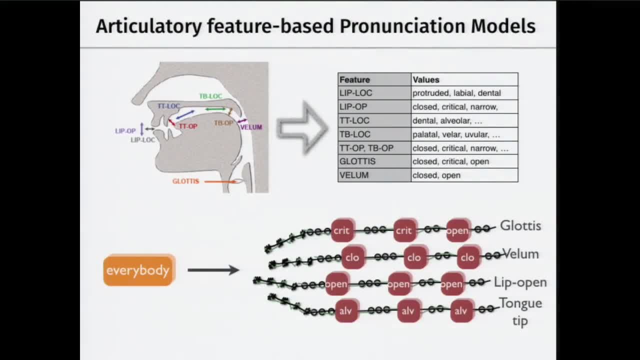 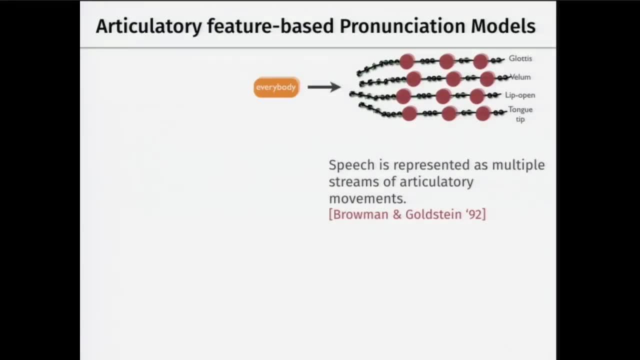 Because they're not entirely independent, right, So one feature can affect how another feature behaves. So this, this idea was. so we kind of got inspiration from this work on this theory called articulatory phonology by Brown and Goldstein. But they said that this representation of speech as just 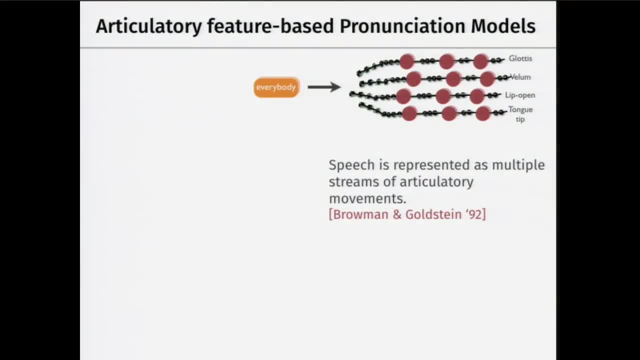 sequences of phonemes is very, very constrained and it's very restrictive. So let's think of speech as being represented as multiple streams of articulatory movements, And that actually gives you a much more elegant framework to represent pronunciation variation. So if I had to go back to the previous slide, 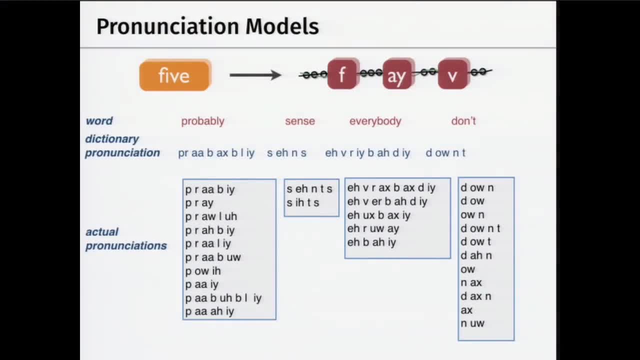 where I showed you all the various pronunciations to try and kind of motivate how you went from the dictionary pronunciation of probably to one of these things. It would require kind of deleting three phones, inserting some other phone, a huge edit distance in terms of. 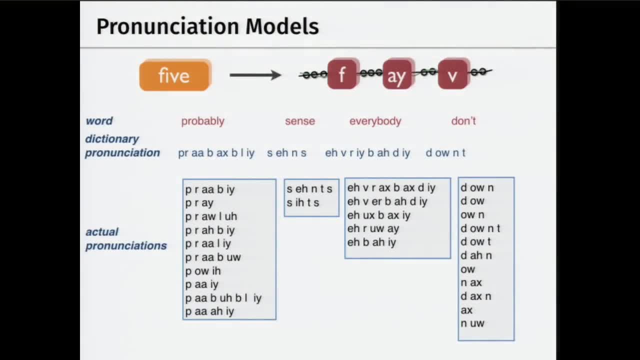 phones. So how do you actually motivate such a large deviation in pronunciation? But it turns out that if you represent pronunciations as these streams of features, you can explain pronunciation variation in terms of asynchrony between these feature streams. So just because certain features are not synchronously moving, 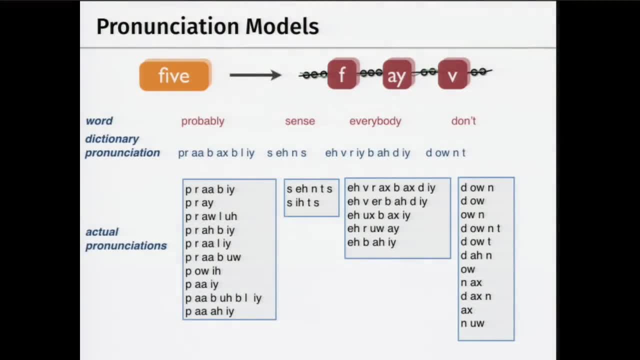 So say that you are producing a nasal sound and your next sound that you're producing is a bubble, But then there's certain remnants of the nasality which hold on, And so your bubble also becomes a little nasalized, and so on. 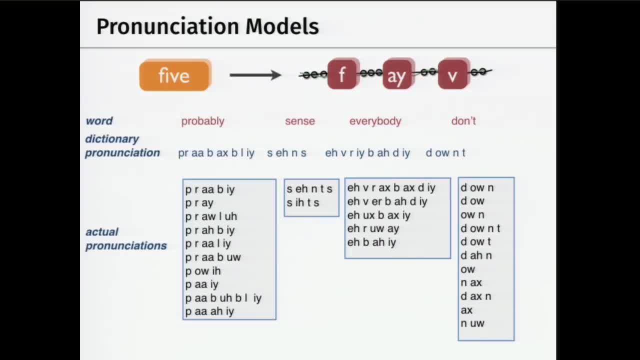 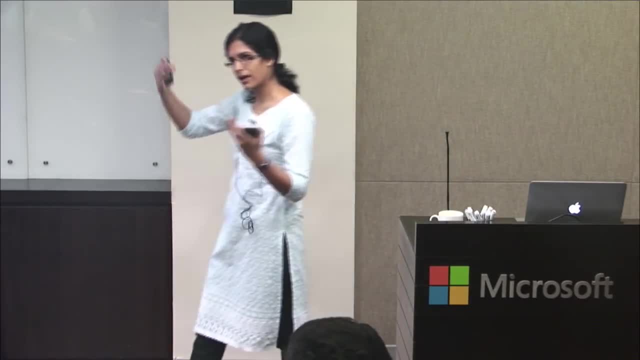 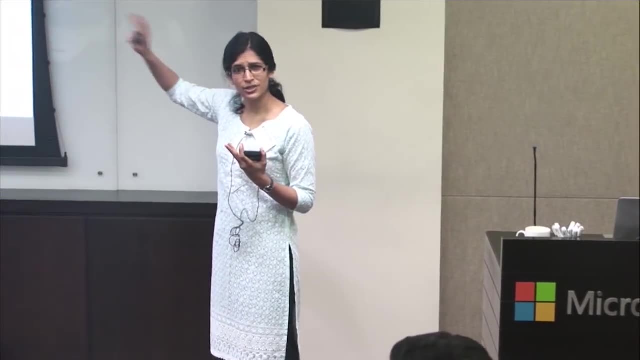 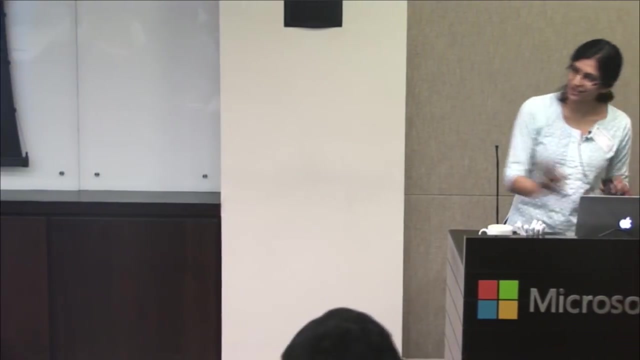 So there was an example which I thought may not have time to go into. So the idea is that this articulatory feature framework gives you more elegant explanations of pronunciation variation. It's certainly more elegant but it's very hard to model And we learned that the hard way I did during my thesis. 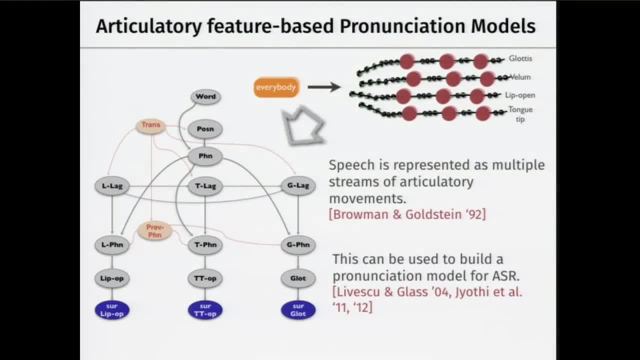 So we used this representation and we built what is in the olden days. These are called DBNs, which is not deep belief networks, it's dynamic Bayesian networks. So it's the olden day DBN. So it's just a generalization of hidden Markov models. 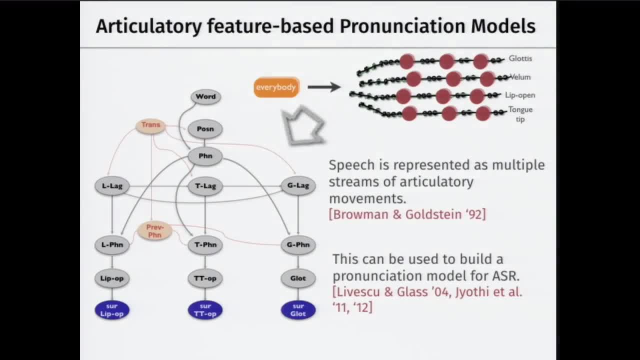 So the hidden Markov model that I described in the acoustic, what I was talking about, acoustic models- This is just a generalization of that particular paradigm. So you have various variables which represent each of these articulatory features, and then you can represent constraints. 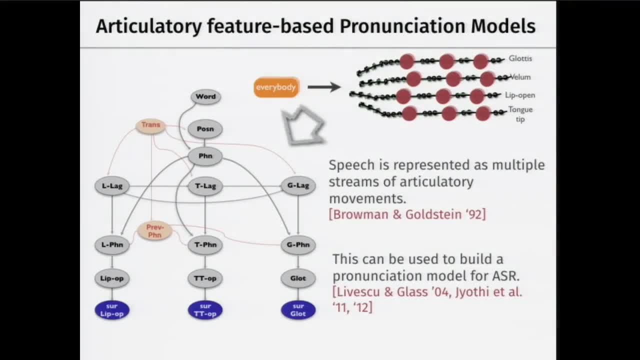 between these variables and so on. So just by yeah, Yeah, Yeah, I wish I had that slide. actually, If you don't mind, can I come to this at the end, Because there's a slide which clearly shows. 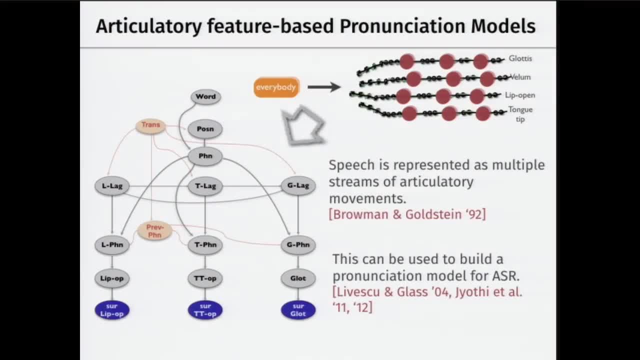 So when you say five, right, Yeah, Yes, yes. And now it's Yeah, Yes, Yes, So now, okay. actually we can take that as an example. So for so now I'll say: for so now, I'll break the first sound. 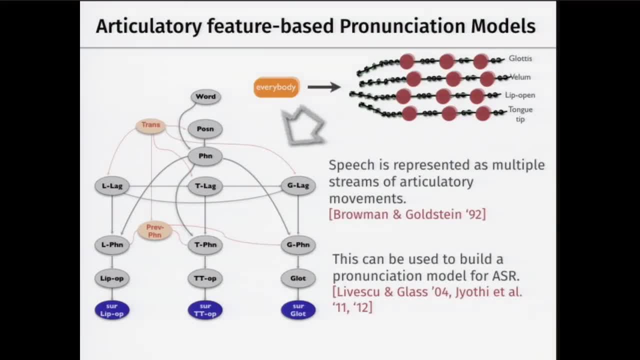 into these eight variables and the values it takes, The values it takes to produce the sound for. So you're, It's no, it's actually not a one-to-one map, So we left it, we kept it probabilistic. So it is mostly one-to-one, but it's not entirely one-to-one. 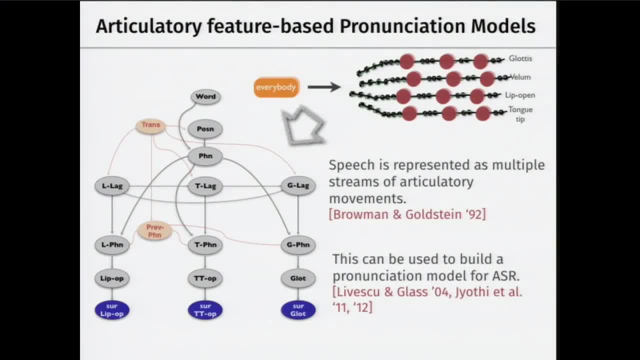 So we did allow for One-to-one Yeah. yeah, It's not a one-to-one mapping, Yeah, it's not a one-to-one mapping, but even if it was yeah. so actually, if I show you that example slide: 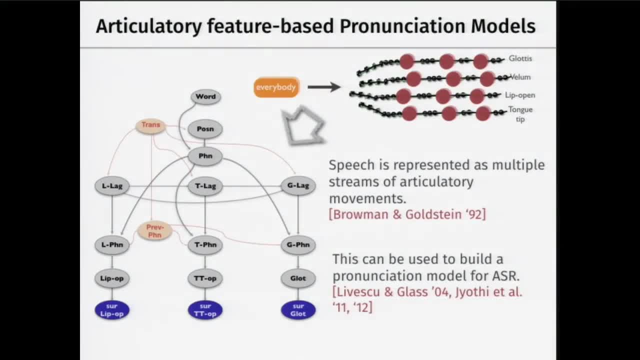 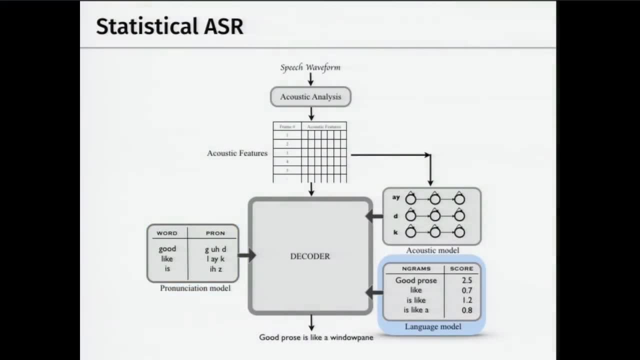 I can clearly explain it, So please remind me at the end of the talk. I'd like to show that. Okay, so that was the pronunciation model, And the final model is what's known as the language model, which many of you might actually be quite familiar with. 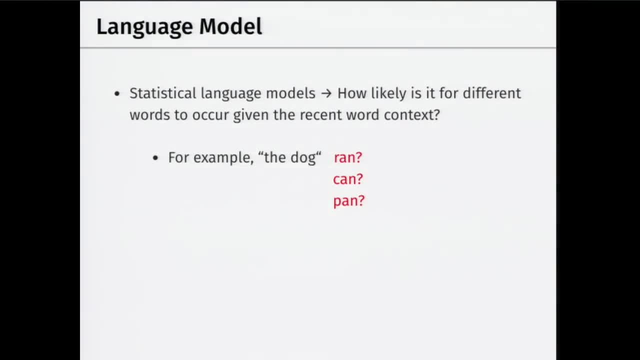 So language model is just saying so. again, in the pronunciation model your output was words. So now you've mapped a phone sequence to a particular word And now the language model comes in and say: how should these words be ordered according to a particular language? 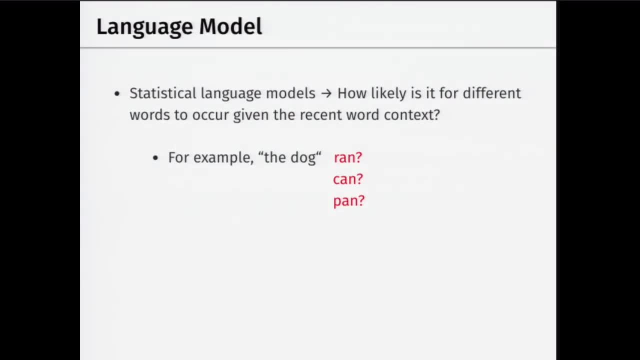 So the language model looks at lots and lots of text in that particular language And it finds occurrences of words together. And yeah, you have a question, Mm-hm. The first case was someone speaking Mm-hm. You said that you get to these phoneme sequences. 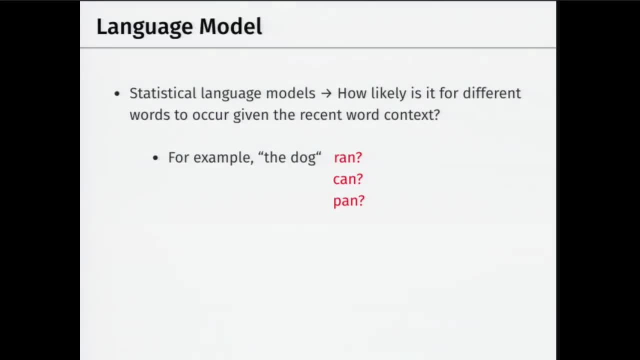 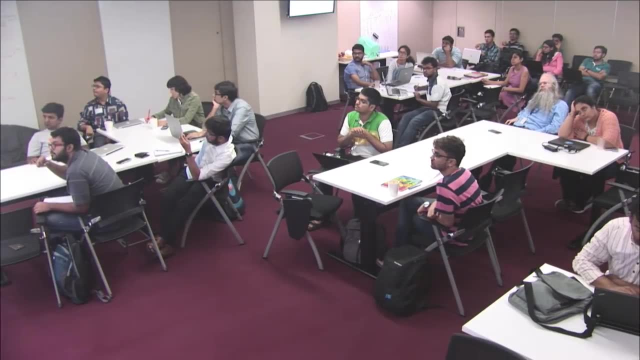 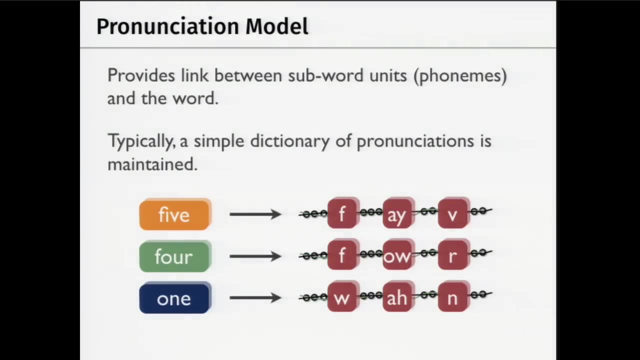 Yes, But so now you're coming to this language model. What about going from the phoneme sequences to words, The pronunciation model? So this one, right? So the phone sequence. so once I get a phone sequence, I can start mapping chunks of the phones to valid words in the pronunciation. 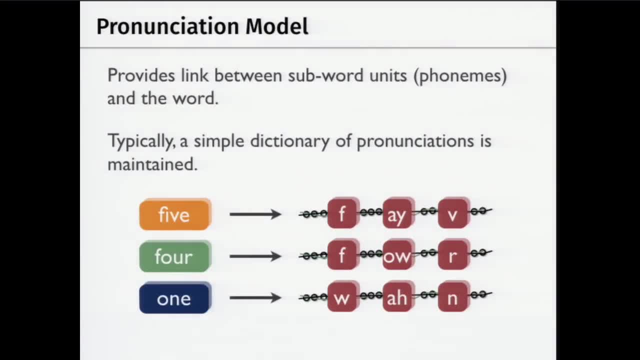 But that can be very wrong. phoneme sequences- Yes, Which do not correspond to any words Yes, absolutely So you could have. so the thing is you're not getting a single phone sequence right, So it's probabilistic. 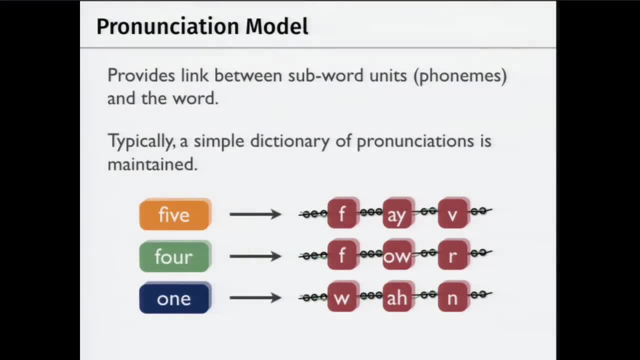 So you have probabilities for every phone sequence appearing And so even if it doesn't exactly match, maybe you will exactly match it with a lower probability. But when the language model also comes in and then the entire probability when you add up, 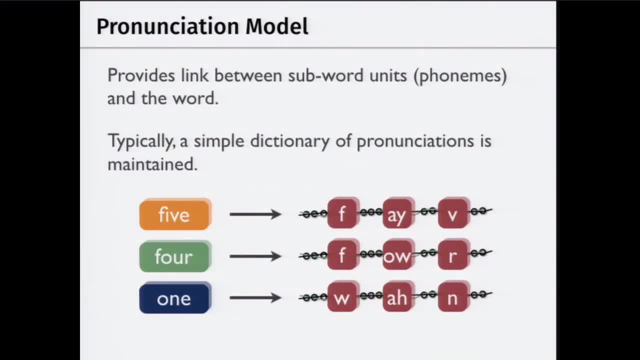 then you'll get kind of the most likely sequence: yeah, Yes, Usually these pronunciation models are not probabilistic. Yes, yeah, they're usually not probabilistic, It's deterministic, It's deterministic. You just have one sequence of, typically. 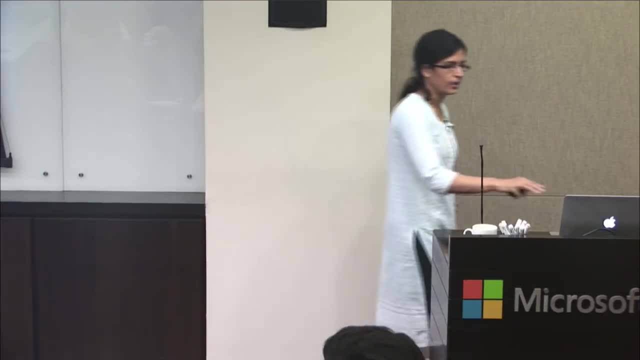 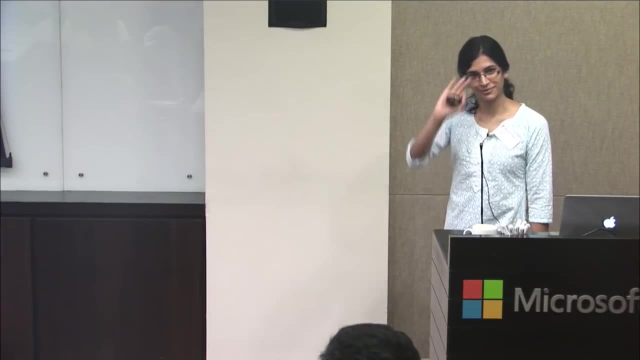 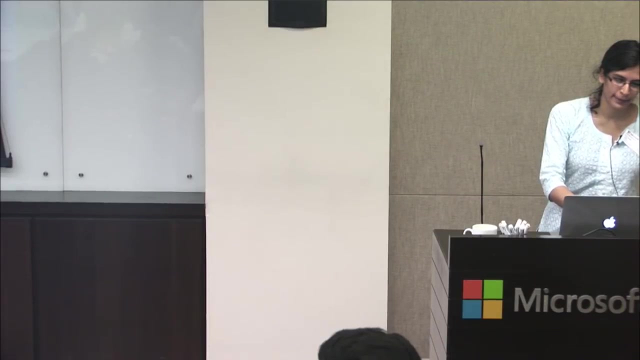 you just have one sequence of phones which corresponds to a word, But it can be probabilistic also. Yeah, exactly, The one I was building was too probabilistic. There are too many probabilities. Yeah, Okay, so here of course. so if you saw the word context, 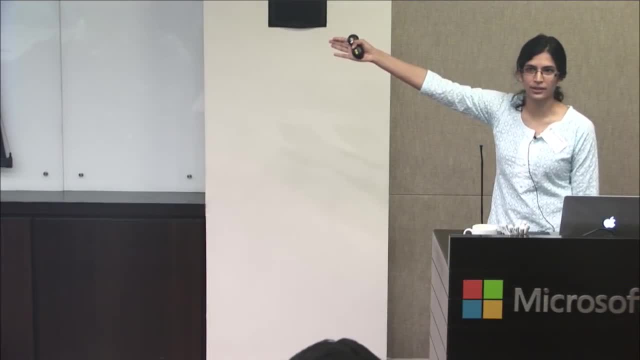 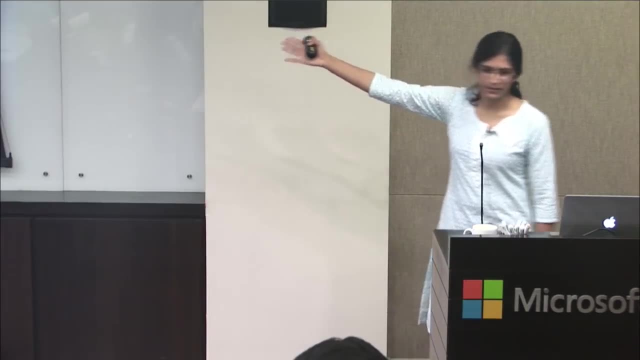 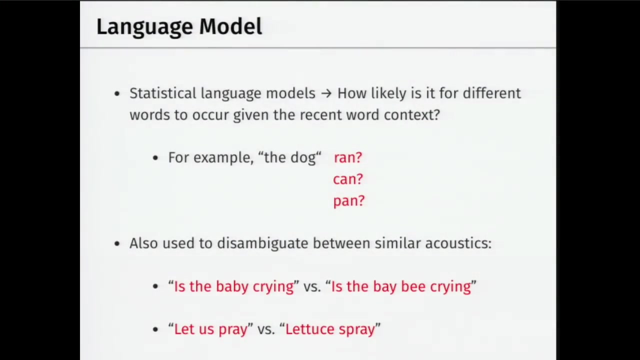 the dog. Obviously, the most likely next word to follow this particular word context is ran, maybe even can, but definitely not pan. So pan would have a very, very low probability of following the dog, And the language model is also coming to actually related to 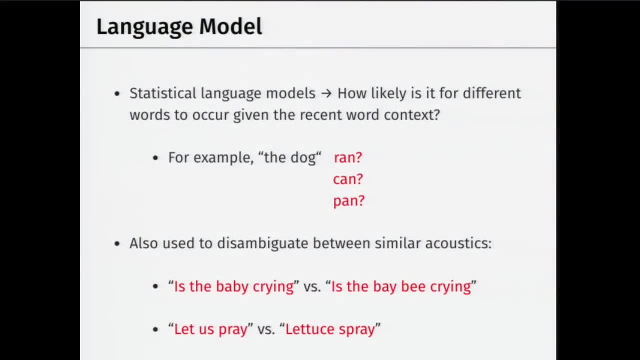 your question. The language model is very crucial because it can be used to disambiguate between similar acoustics. So say that your utterance was: is the baby crying? It could also very well map to this particular word sequence, But obviously the first word sequence is much more likely. 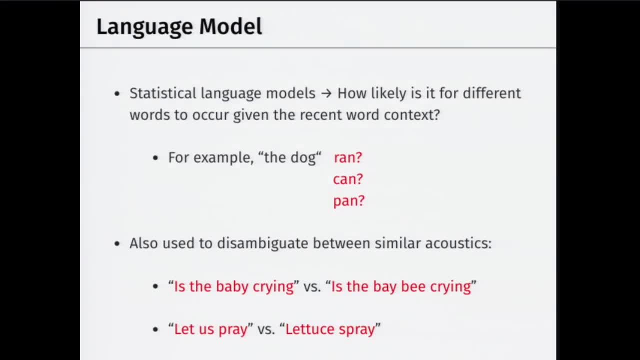 Because if you look at large volumes of English text, is the baby crying is probably a much more likely word ordering than is the baby crying. and then let us pray and let us pray. So if you have identical acoustic sequences, your language model has to kind of come in and do its job well. 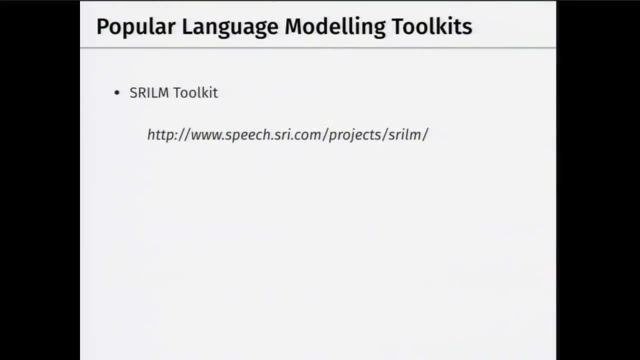 Okay, so I just wanted to put this here if you wanted to use language models in your work. So SRI-LM. so actually, Alan also mentioned about SRI in his talk, So they have put out this toolkit which is extensively used in many communities. 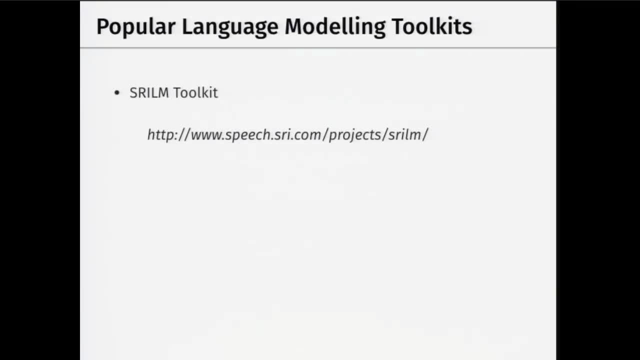 So it's known as the SRI-LM toolkit. It has lots of inbuilt functionalities implemented, So this is a good toolkit to use. Another toolkit which is getting quite popular nowadays is the Ken-LM toolkit, Which handles large volumes of text. 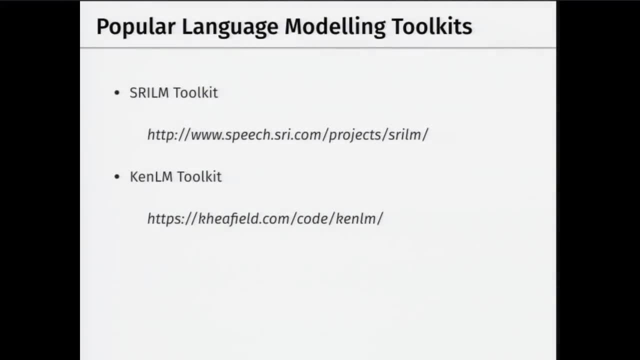 Very, very efficiently. So the data structures which they've used to implement this toolkit are much more sophisticated. So this is much faster, Ken-LM, But probably you only need to use this if you're dealing with very large volumes of data. 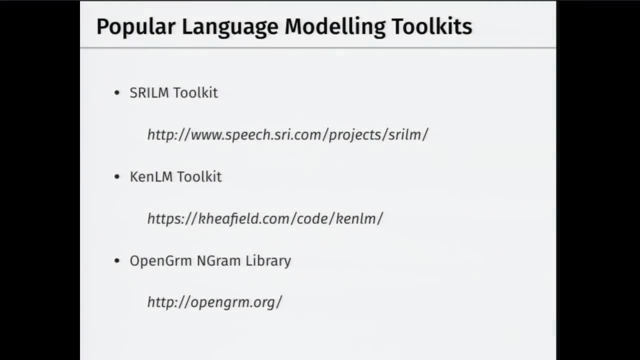 And there's also this OpenGram Ngram library. So if you like finite state machines, if you like working with finite state machines, you want to represent everything as a finite state machine, then this is the toolkit for you. So OpenGram Ngram- it was developed by me. 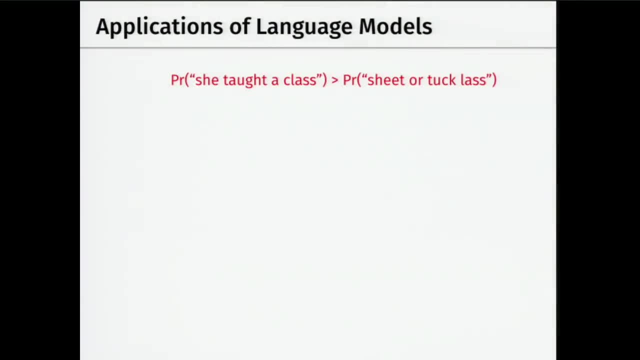 It was developed by Google. Okay, so language models. like I mentioned, it has many applications, So speech recognition is just one of them. Machine translation is another application where language models are heavily used. Handwriting recognition, optical character recognition- all of these also would use language models on either. 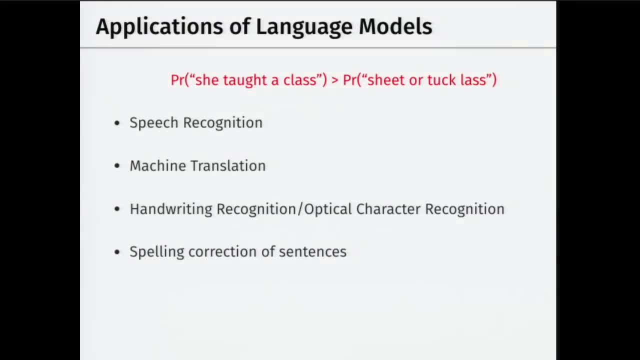 letters or on characters Spelling correction. again, language models are useful here Because you can have language models over your character. space, Summarization, dialogue, generation, information- the list is really long. So language models are used in a large number of applications. 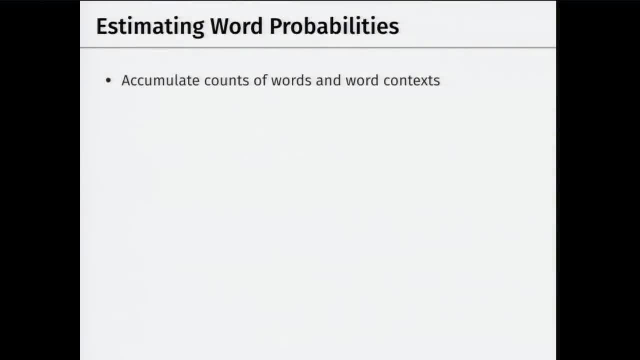 So I just want to mention this one point about language models. So we mentioned that you look at these word contexts And you look at counts of these words in these word contexts over large text corpora in a particular language. How often do these particular set of words appear? 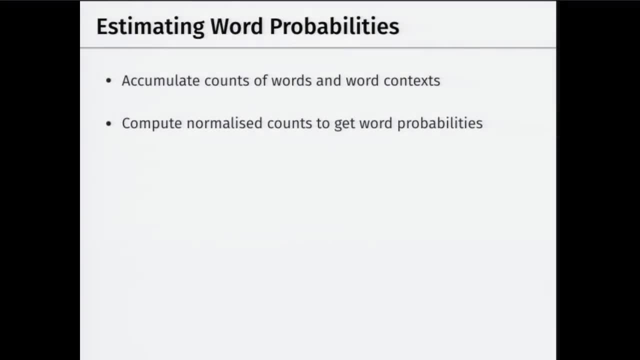 And then you compute some relative counts So you see, okay, these chunks appear so often and these are the total number of chunks, And so you get some relative counts So it'll give you some probability of how often you can expect this particular chunk to appear. 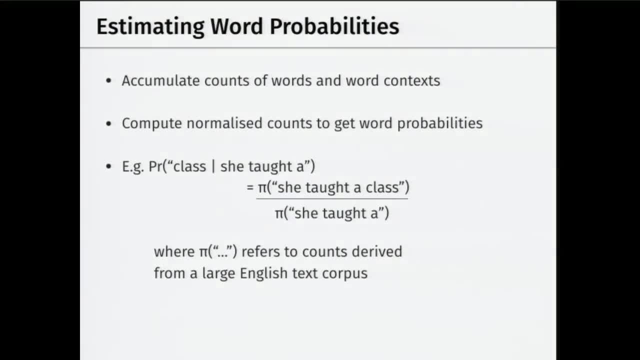 So just to kind of slightly formalize that. So this very, very popular language model which is used are these Ngram language models, And the idea is really straightforward. So you just look at co-occurring- either two words or three words or four words. 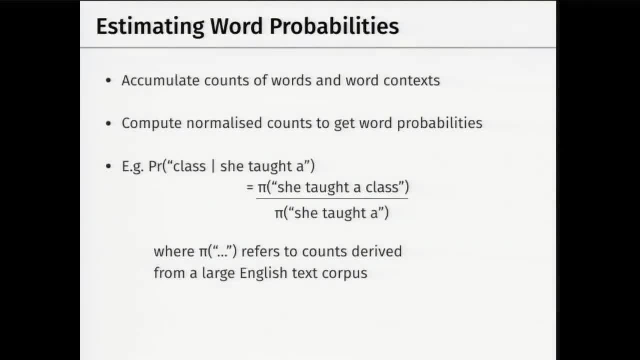 So if N is two, then you're looking at bigrams, If N is three, you're looking at trigrams, N is four, fourgrams and so on, And Alan mentioned yesterday, if you're already looking at fivegrams, you can pretty much reconstruct English sentences. 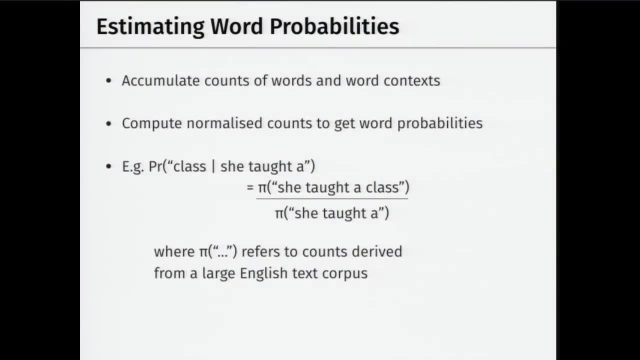 really well. But of course then you're running into really really large number of Ngrams As you increase the order of the Ngram. So here I'm looking at a fourgram. So the fourgram is: she taught a class. 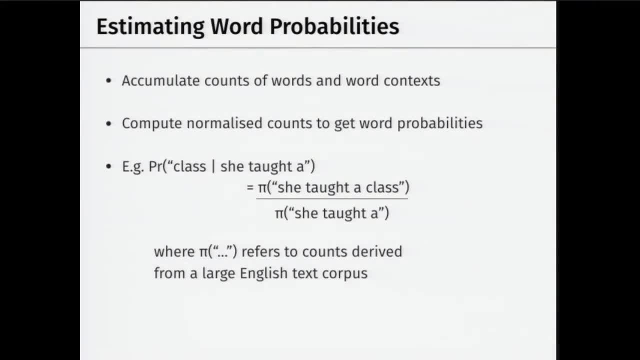 So what is the probability of this particular fourgram? That is, the word class follows this particular word context: she taught her. So you look at counts of she taught a class in large volumes of English text And then you normalize it with the counts of she taught her. 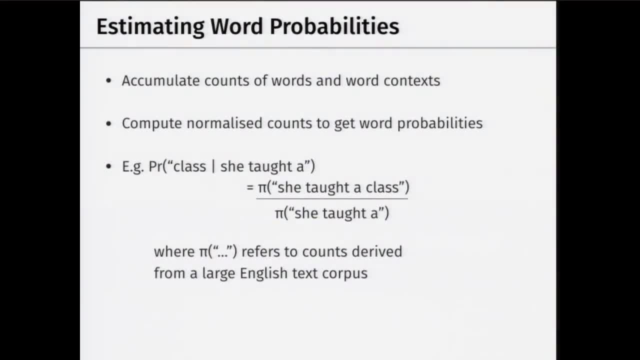 which is the word context. So how often does class come after this particular word context? So what is the obvious limitation here? Yeah, exactly. So this is: we'll never see enough data. We're always going to run into Ngrams. 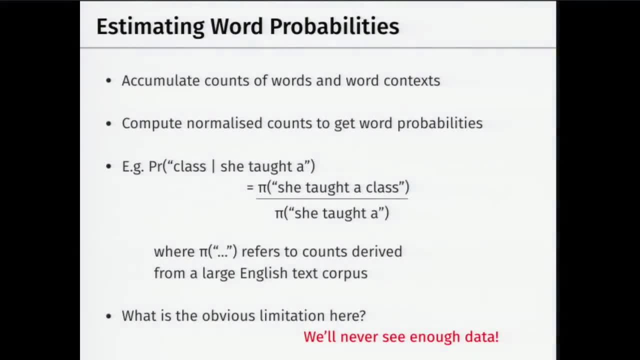 which we're not going to see in the text corpus, And this is actually. this happens far more frequently than one would even expect. Even if you have really really large databases of Ngrams, you're going to run into this issue. So just to make sure that this is true. 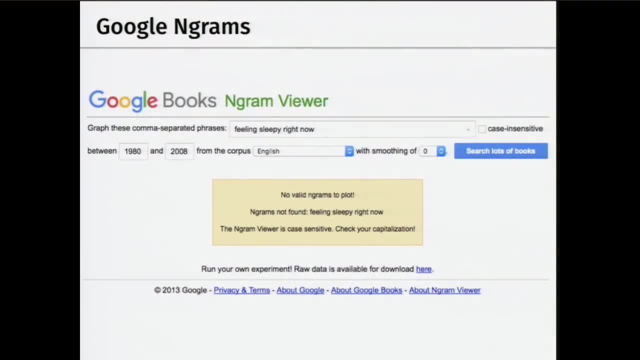 I went into this Google Books, So Google Books has accumulated lots and lots of Ngrams from all the books which are available on Google. This is in English, So you can actually plot how the Ngrams have appeared in books over some particular time frame. 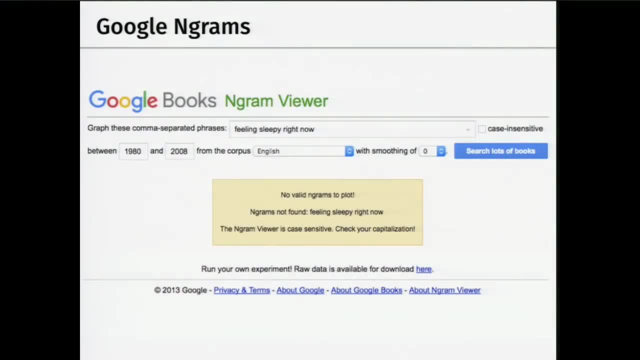 So you can go and play around with this if you've not seen this before. So I just typed in this particular fourgram, which hopefully is not very relevant to this crowd. So feeling sleepy right now And there weren't any valid Ngrams at all. 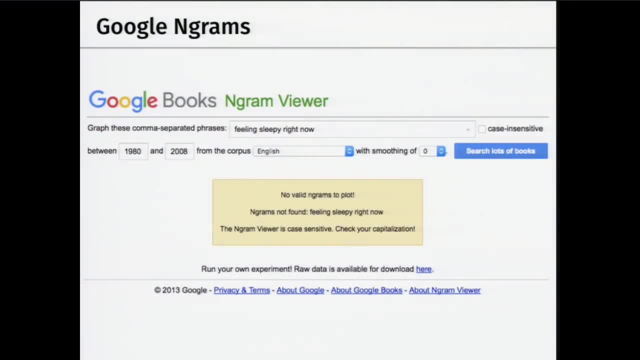 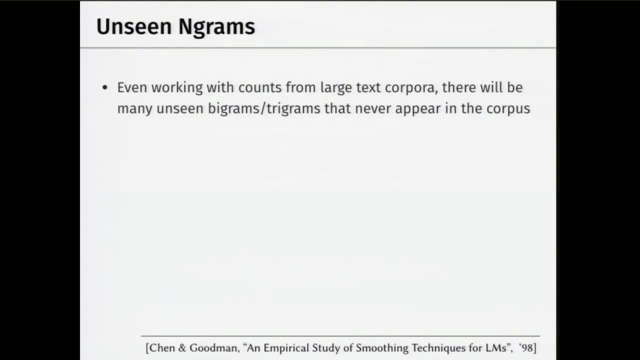 And this is not a very, very rare fourgram right, And even feeling sleepy right. None of them appear in text. So this is a problem which occurs actually very, very frequently. So even when you work with these counts from very 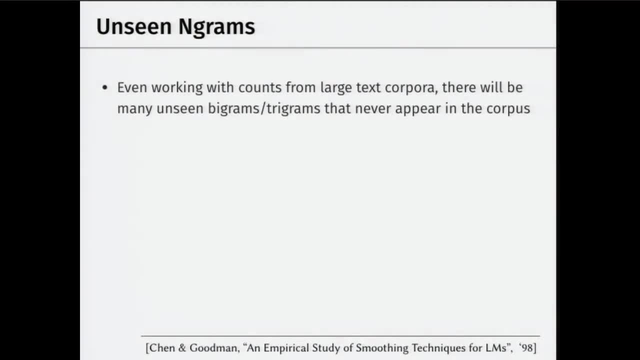 very large text, corpora, you're always inevitably going to run into this issue, which is you're going to have these unseen Ngrams which never appear in your training data. And why is this an issue? Because during test time, when you're trying to reorder words, 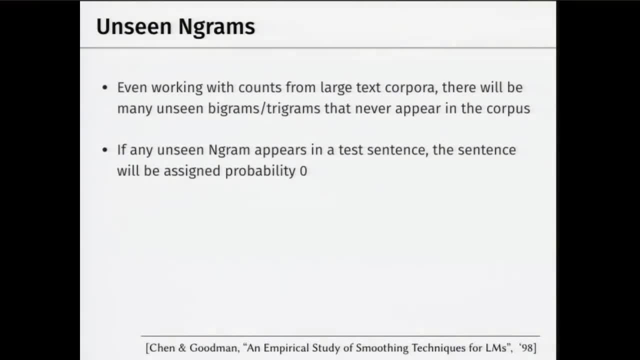 according to your particular language model, and if any of these unseen Ngrams appear in your test sentence, then the sentence is going to be assigned a probability of zero because it has no idea how to deal with this unseen one. So there is this problem with what are known as unsmoothed 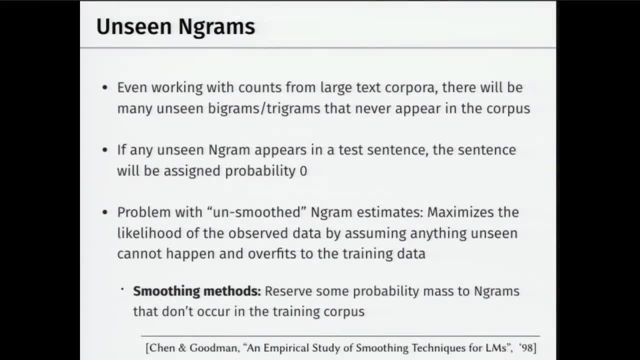 Ngram estimates And I wanted to make it a point to actually talk about this, because Ngrams are only useful with smoothing. So these unsmoothed Ngram estimates, like I mentioned, you'll always run into these unseen Ngrams and 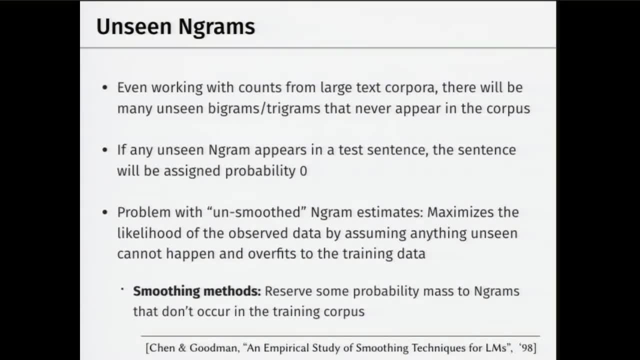 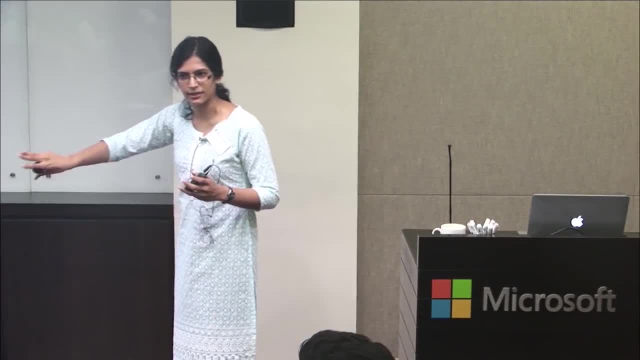 then what do you do? So there are a horde of what are known as the smoothing techniques. So you're going to reserve some probability mass from the seen Ngrams towards the unseen Ngrams, And then there are questions like how do you distribute that probability mass across the 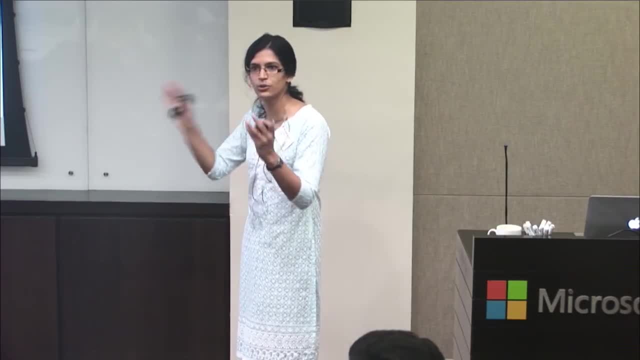 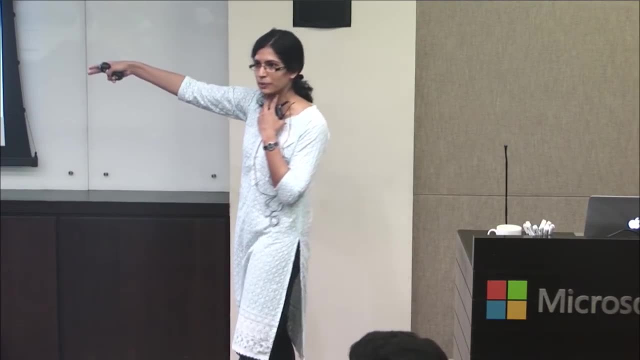 unseen Ngrams And there are various techniques for that as well, like how do you distribute that remaining probability mass? So there's kind of a lot of work on smoothing methods and it's very useful to make Ngram models to make them effective. 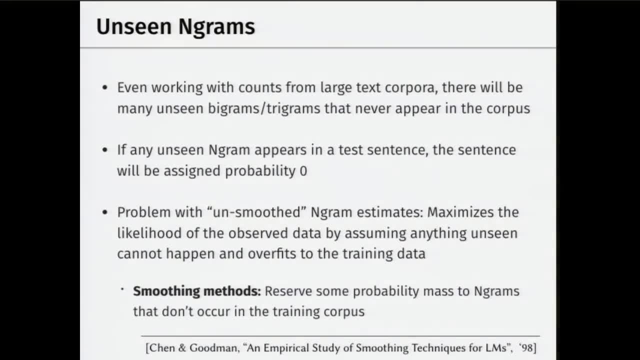 So for anyone who's interested, I would highly recommend reading this 1998 paper by Chen and Goodman. Actually, Goodman was at MSR. I don't know where he is now- So this is an empirical study of smoothing techniques for LMs. 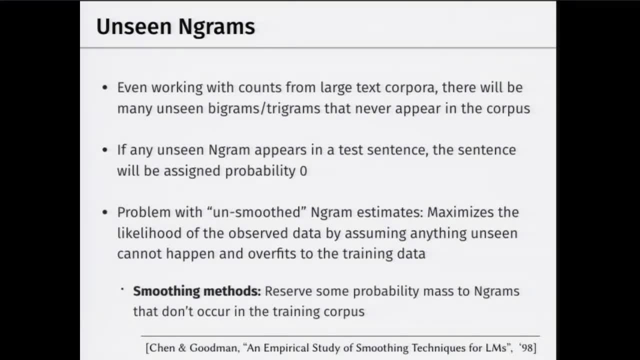 I highly recommend this. It's kind of long, but it really gives you a very deep understanding of how smoothing techniques help. Don't be fooled by the 1998.. It's still very relevant today, because Ngrams are very relevant even today. 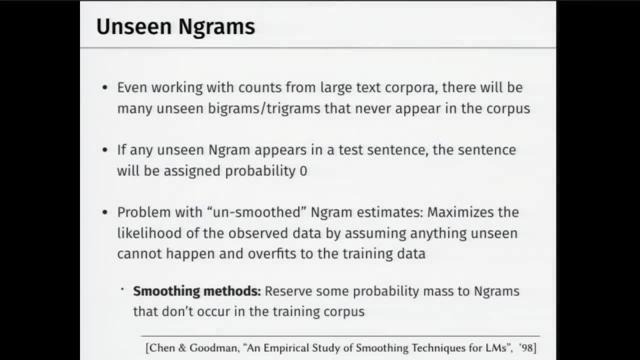 So Ngrams are not going anywhere. So I'm not talking about what the latest language models are, but these days in speech recognition systems we've moved towards these, what are known as recurrent neural network based language models. So that's neural network based, but I believe it's still not. 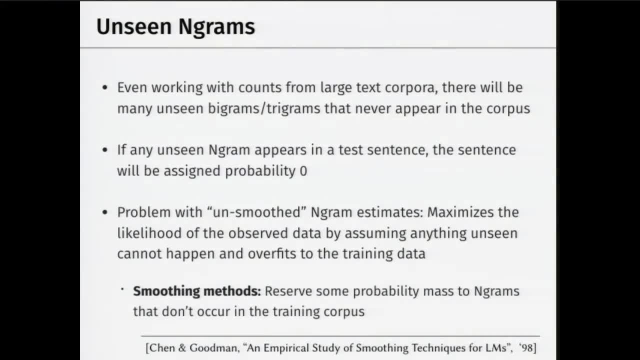 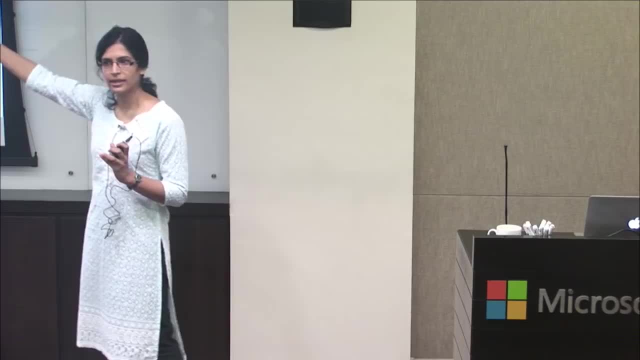 folded into a lot of production systems because it's not very fast. So many of the production level ASR systems probably still use Ngrams and then do a rescoring using recurrent neural network language models. But yeah, so Ngram models are still very. 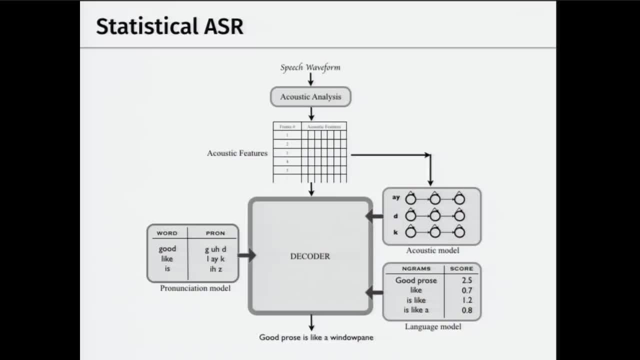 very much. There's a lot of research in the picture. Okay, so we've already covered each of these individual components, but there's this big component in the middle right which is the decoder, And that's actually a very important component. 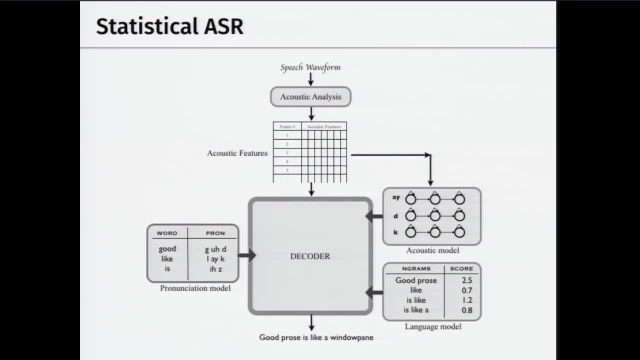 So I have all of these parts of the ASR system which are giving me various estimates of what is the most likely phone sequence, what is the most likely word sequence, and so on, But finally I just want to get the most likely word sequence. 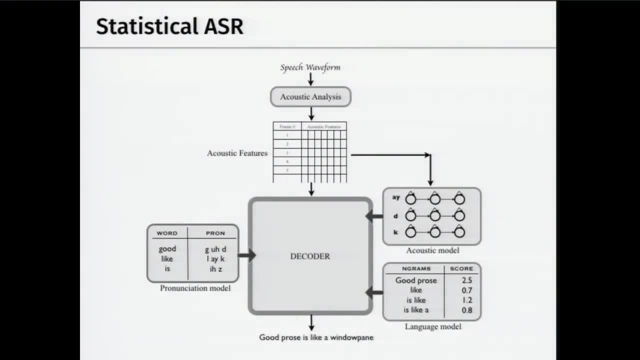 corresponding to speech utterance, And so then it's a search problem. So I have these various components And now I need to search, putting all of them together, I need to search through this entire space. So, just looking at the very simple example we started with, 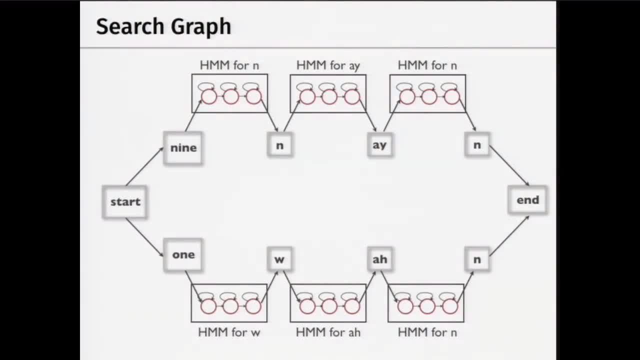 this is what a naive search graph would look like. So you start at a particular point and say that you only expect it to be nine or one, just these two words. Then you need to transition to nine. So here every single arc doesn't have a weight. but 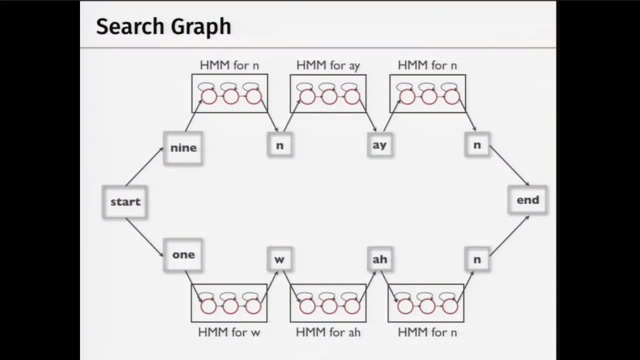 these are all weighted Because they all come with their associated probabilities. So from start you can transition into either producing the word nine or one. But each nine is a sequence of phones And each sequence of each phone corresponds to its corresponding HMM, which has its own probabilities. 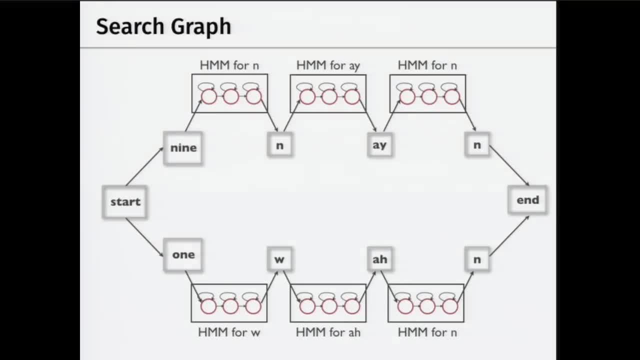 So this is already. you can see this is quite a large graph just for these two words, And at least a half decent system will be looking at at least 20,000 words out of 40,000 words. So you can imagine how much this search graph blows up. 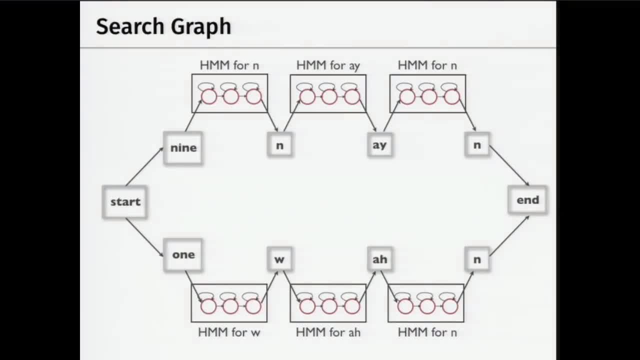 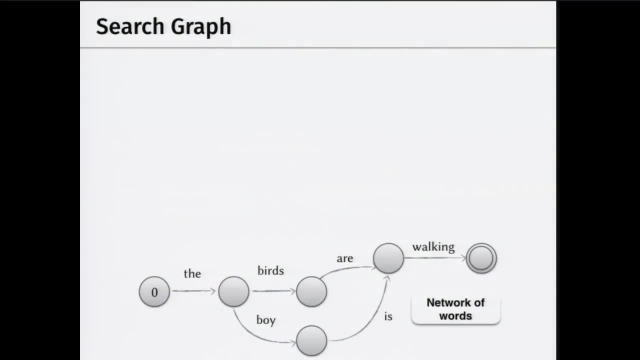 So these are really large search graphs And I think I have another slide. Yeah, so if you have, say, a network of words as follows: So the birds are walking, the boy is walking. This is really simple, right? This is not an N-gram model. 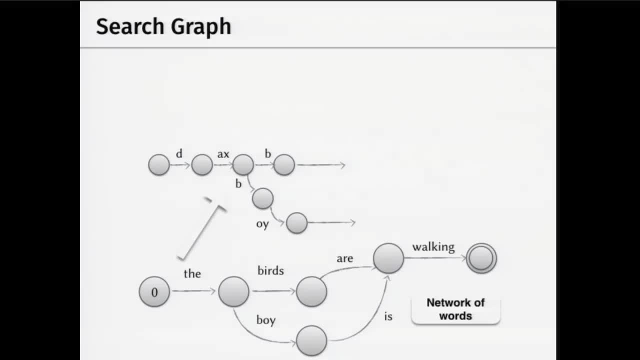 This is just. this is highly constrained, right. And so now, each of these are now going to map their corresponding phone sequences, So the birds and so on, And each of those phones now are going to correspond to their underlying HMMs. 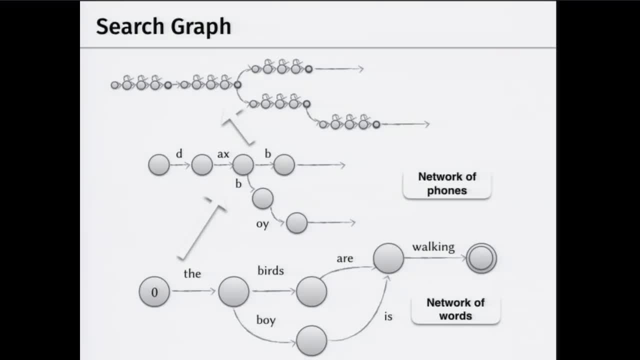 And very quickly the graph blows up. So if you look at so, just to give you an estimate, vocabulary size of around 40,000 gives you search graphs of the order of tens of millions of states and arcs. So these are really large graphs. 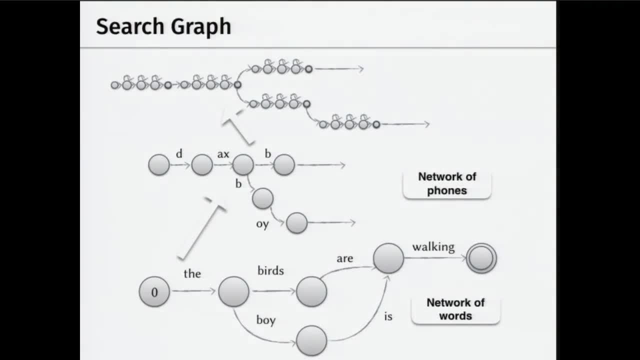 And so now we need to search through these graphs and see what is the most likely word sequence to correspond to the speech utterance. So you might be wondering: how do you? can you do an exact search through this very, very large graph? And the answer is no. 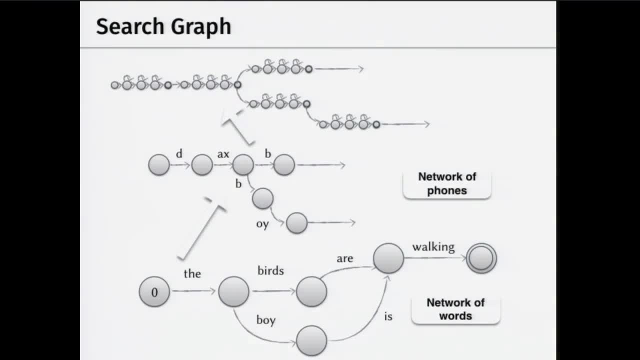 You cannot do an exact search through this graph because it's just too large, So you have to resort to approximate search techniques, And there are a bunch of them which do a fairly good job. So none of these speech systems that you work with are actually. 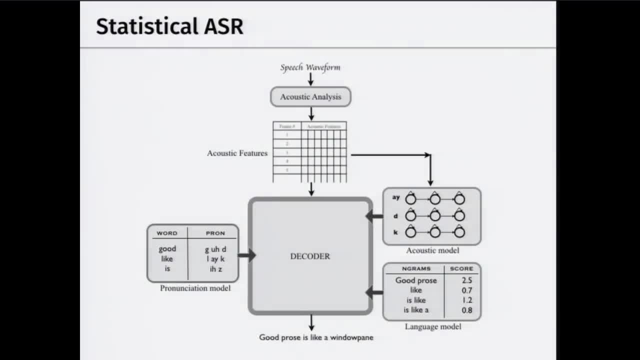 doing an exact search through this graph. Okay, so that's the decoder. So any questions so far. So this is the entire kind of pipeline of how an ASR system works. Okay, so everyone is with me, right? So I want to kind of end with this new direction, which is kind 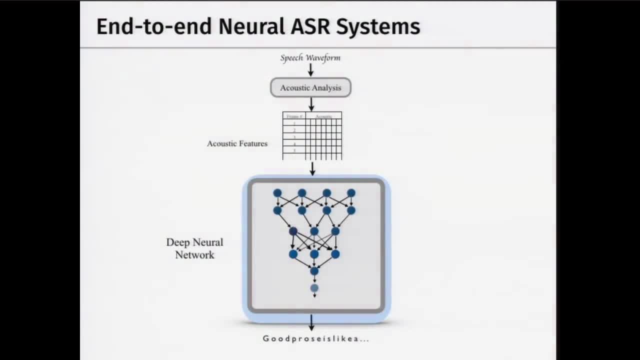 of becoming very hot nowadays And they are known as these end-to-end ASR systems. So I showed you all of these different components which put together make up an ASR system. But lots of people are interested in kind of doing away with all of those components. 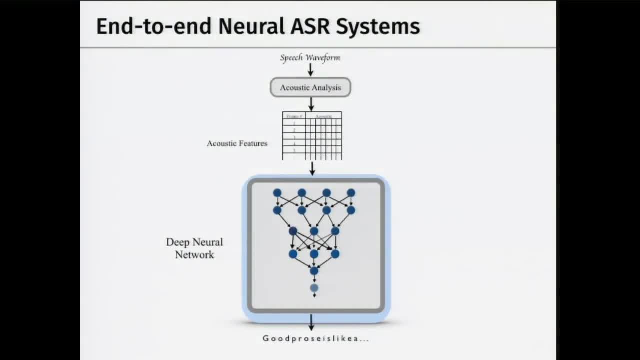 Let's not worry about how a word splits into its corresponding phone sequence, Let's just directly learn a mapping from acoustic features to letters. So this is just to characters. So directly go from speech vectors, so these acoustic vectors to a character sequence. 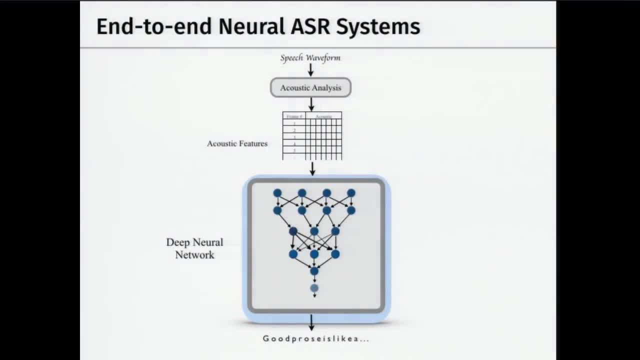 And then you can have character language models which rescore the character sequence and so on. So this one kind of nice advantage of this is that because you're getting rid of the pronunciation model, which is that you're not now looking at phones at all- 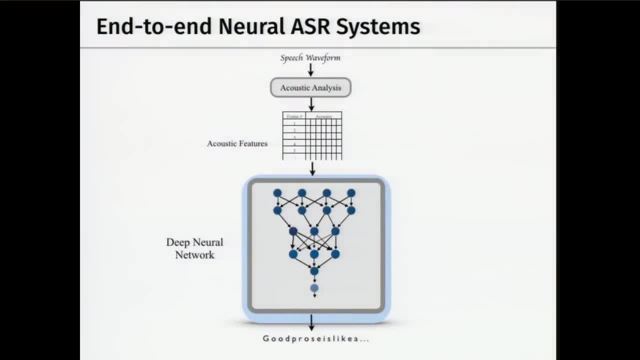 You don't need that mapping the word to phone mapping, which typically is written down by experts and that changes for each language. So now you want to build a new system for a new language. If this worked really well, then all you need is speech and 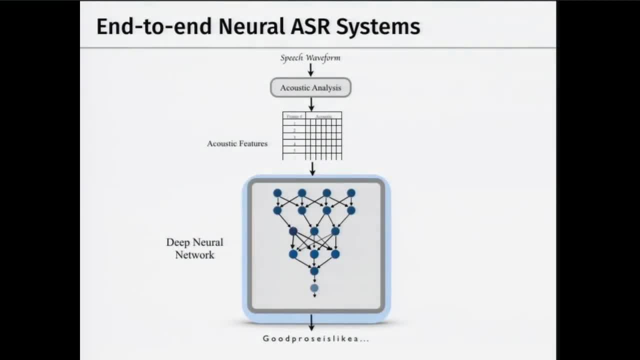 the corresponding text. But the catch is you need lots and lots of this for this to work well, for these kinds of end-to-end systems to work well. So just for people in the crowd who are interested in these kinds of models, I'll just put down a few references which you can read. 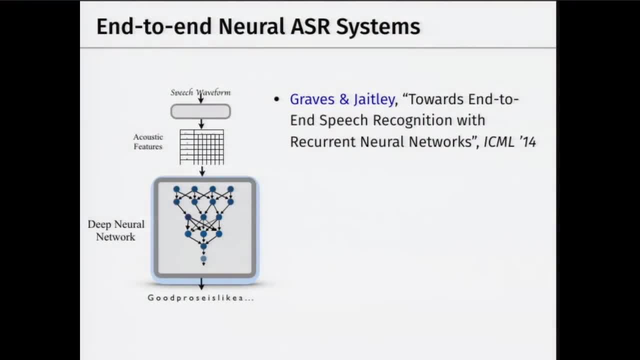 So the first is this paper which came out in 2014 and kind of started off this thread of work which is this end-to-end speech recognition with recurrent neural networks. So I won't go into details at all about the model, This is just for. 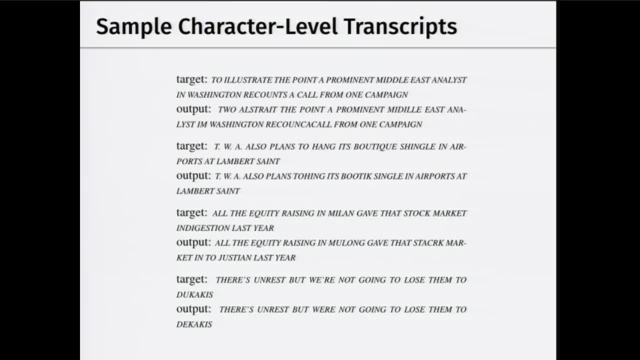 you to jot down if you want to go later and read it up. But I'll put this up, which is kind of their sample character level transcripts which they get out of their end-to-end systems. So here they have a bunch of target transcriptions and 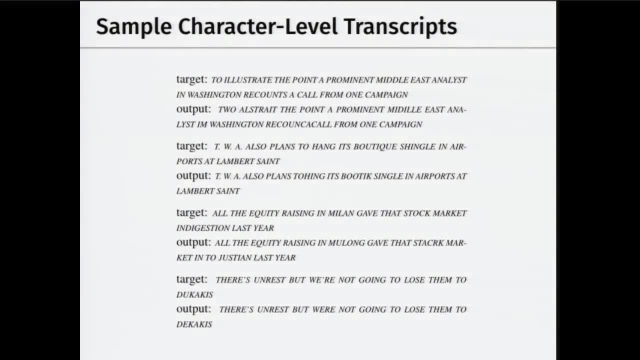 the output transcriptions So you can immediately see. so this is without any dictionary, without any language model. So this is directly mapping acoustic vectors to letters so you can see obvious issues like lexical errors. You can see things where you have phonetic similarities. so 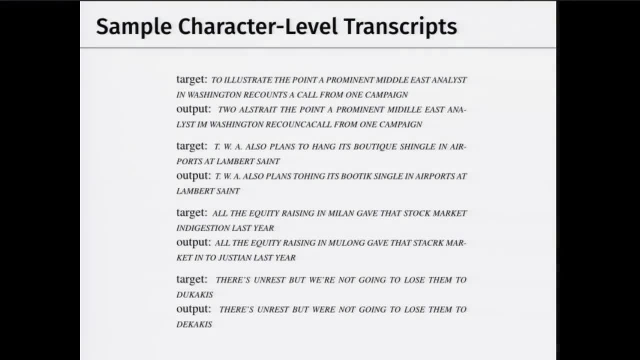 shingle becomes single. Then there are words like Dukakis and Milan, which are apparently not appearing in their vocabulary. So that is another advantage of these character models. So in principle, you don't care about whether you've ever seen this word in your vocabulary, because you're only predicting. 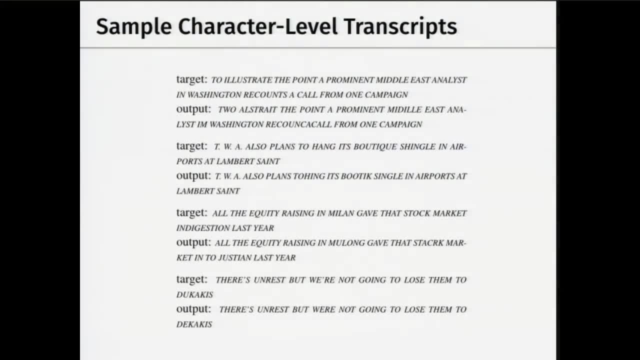 one character at a time. So it should recover out of vocabulary words. But this system doesn't actually do that too well. It does, yeah, So they just had this without the dictionary, without a language model, But their final numbers are all with a language model and 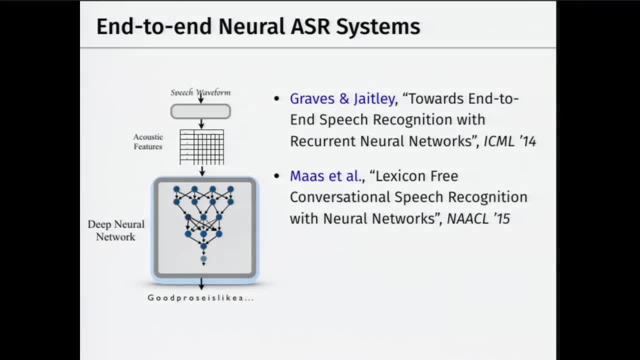 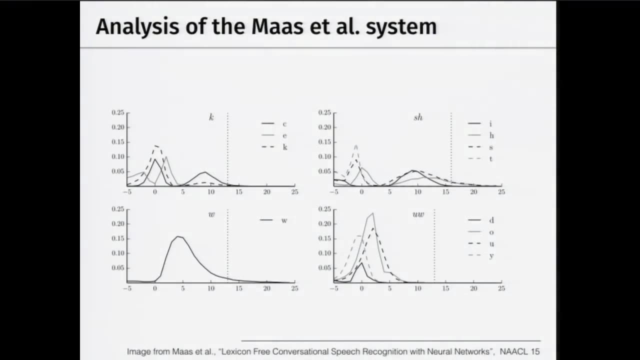 a dictionary also, actually. So the second kind of improvement on this paper was by Ma Sattal, who again explored a very, very similar structure to the previous paper in 2014.. And they had this kind of interesting analysis which I wanted to show. 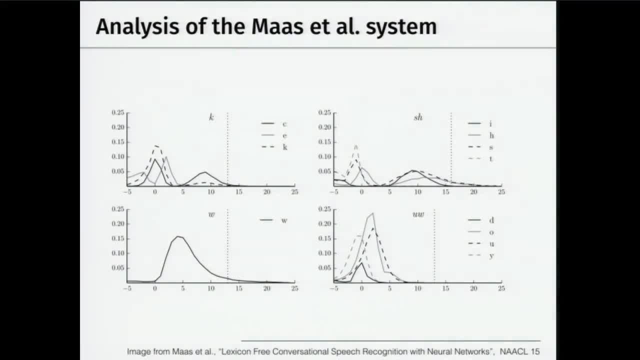 So on the x-axis, you have time, And each of these graphs correspond to various phones. So remember, in their system there are no phones at all, But they just accumulated a bunch of speech samples which correspond to each of these phones. 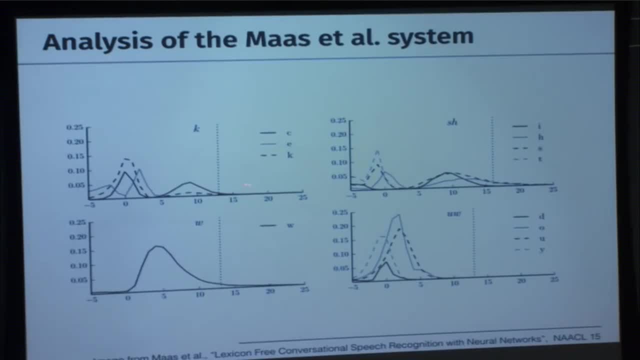 And averaged all the character probabilities corresponding to those particular phones. So here you can see that K obviously comes out, but so does C. So the letter C also corresponds to the K sound, And interestingly for sure. so this is the phone, sure? 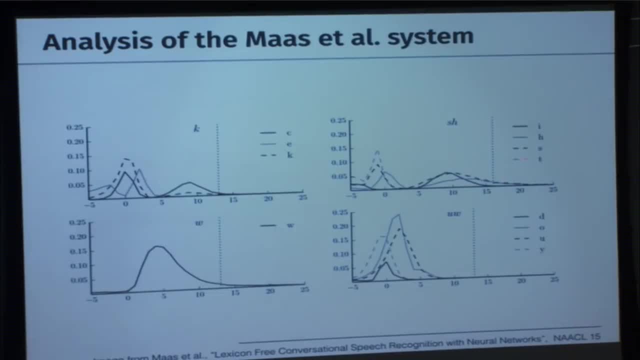 So S and H. so SH definitely comes out, But so does TI, because, as in shun, T-I-O-N, So you would pronounce that as sure right. So that actually comes out of the data, which is pretty cool. 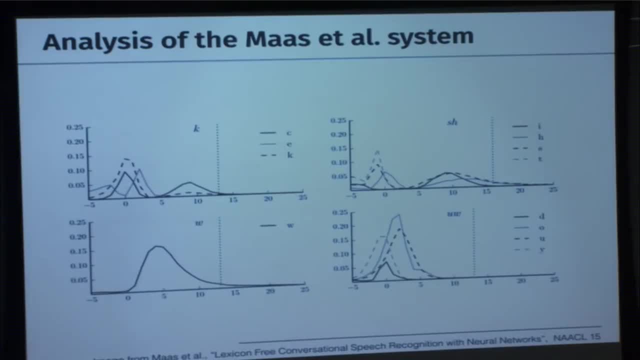 So this, yeah, So this was a nice analysis. So they do only slightly better than the previous paper. And yeah, So the x-axis is time in frames, You can think of it in speech frames, And these are just the character probabilities, yeah. 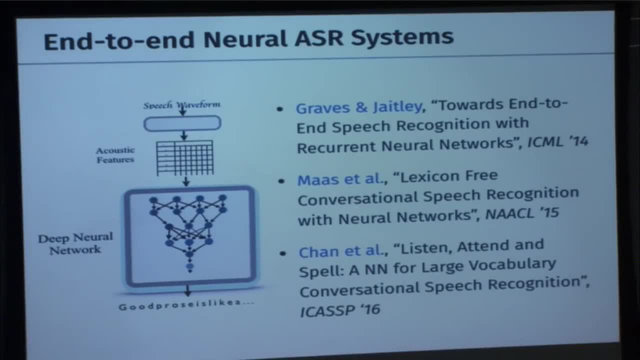 So the last system, which came out in 2016, and kind of significantly improved over these two, uses this very popular paradigm now in sequence-to-sequence models, which are known as encoder-decoder networks or sequence-to-sequence networks, Which was first used for machine translation. 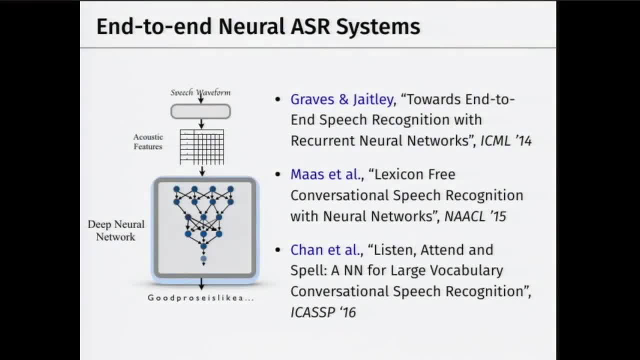 And now they applied it to this particular problem and also included what is known as attention, And all of these bells and whistles together definitely make a difference, But I want to mention that end-to-end systems and this whole pipeline are not yet close to the entire standard. 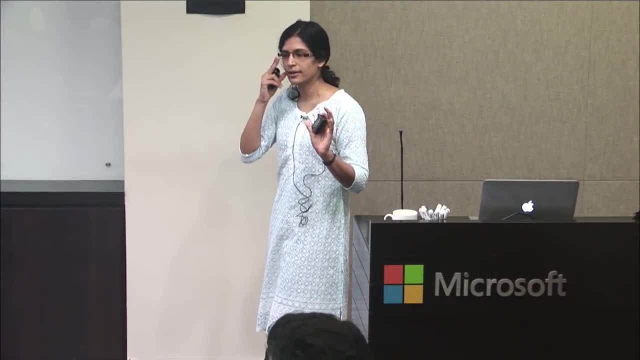 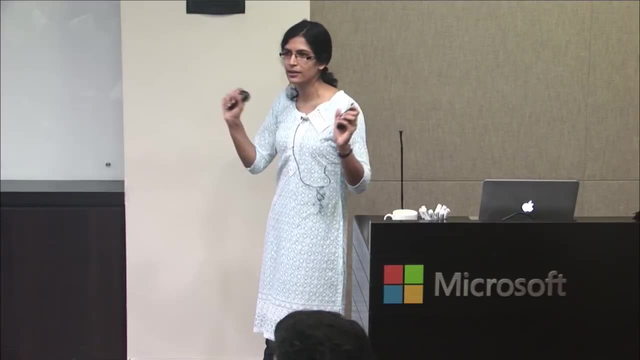 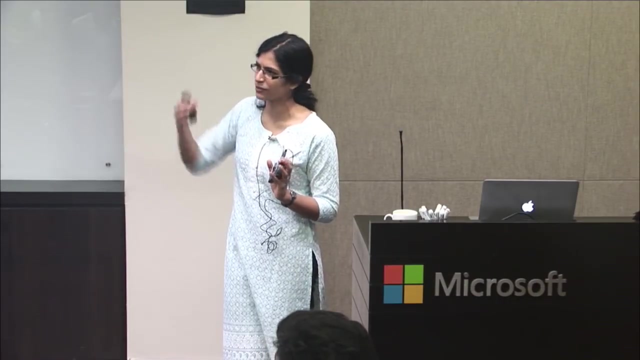 pipeline that I showed you earlier. So people would really like to bridge the gap between end-to-end systems and this whole pipelines, Because clearly these are much more at least easier to understand in some sense, at least from a modeling standpoint, Although it's not easier to understand what it's doing. 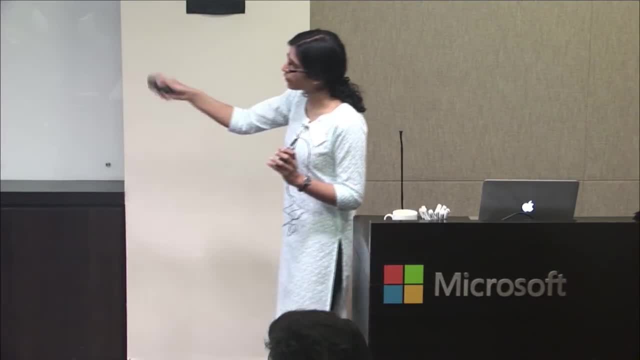 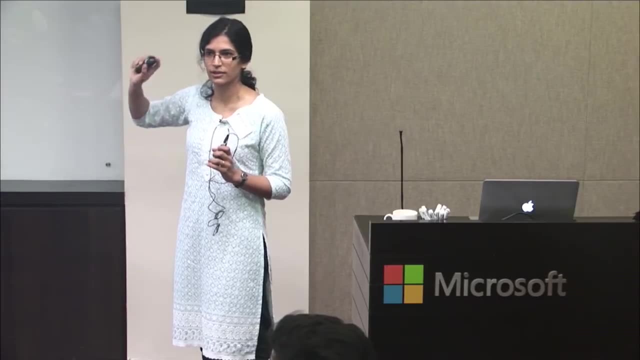 Yeah, so there's a lot of work going on in this particular area, But these systems require lots of data, lots and lots of data to train. And that's because not only are you trying to understand what are the underlying speech sounds in the speech utterance, 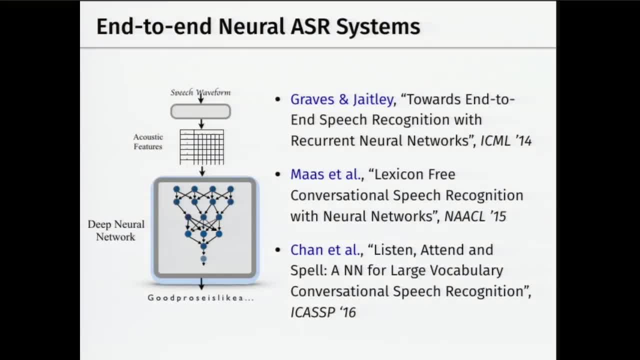 you're also trying to understand spelling. You're trying to figure out what spelling makes sense for a particular utterance, And clearly, for a language like English, where the orthography is so irregular, it's a hard problem, And so these models require large amounts of data. 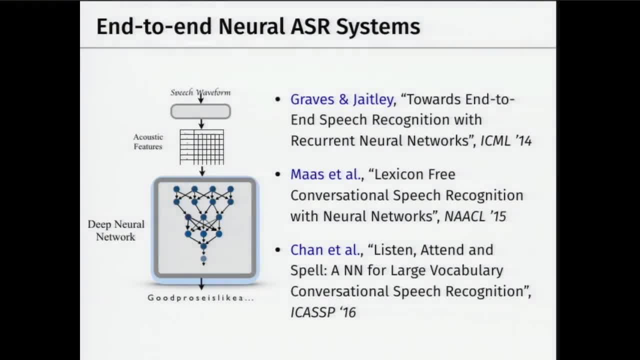 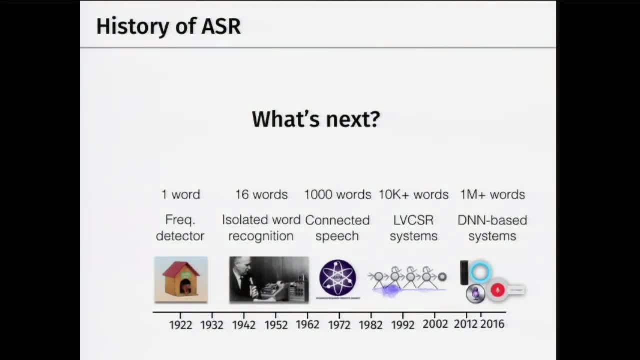 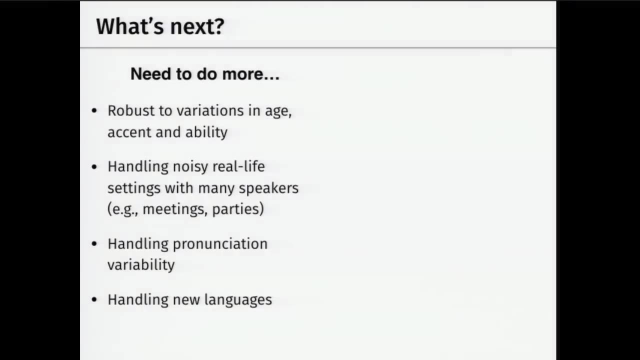 So I'm going to come back to this question I posed initially, which is what's next? So what are all the kinds of problems that we could work on if anyone was interested in speech recognition? So I think there are lots of next steps. 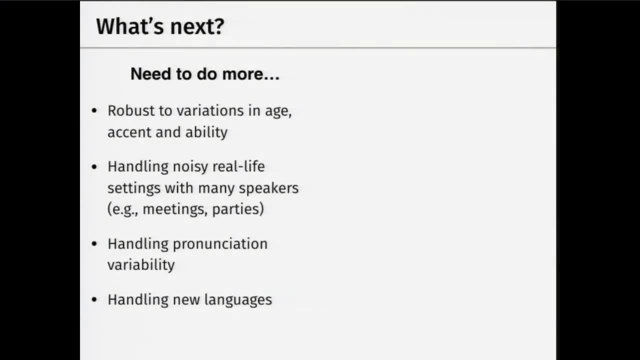 So one is, you need to do more to make ASR systems robust to variations in age, accent of speech- accent, of course- which is why we are working on that problem. And also- this is another thing which people are interested in- 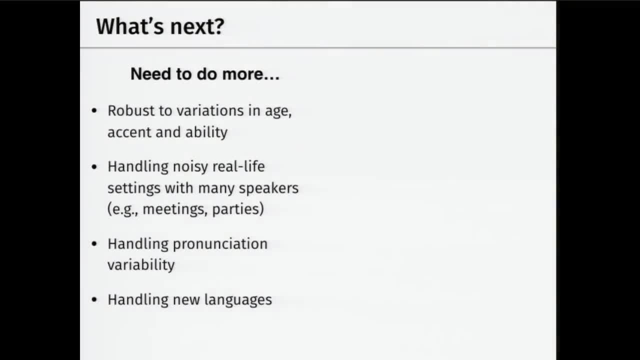 so just speech ability. So there are people say with speech impediments, they stutter or they have other issues And they're not able to speak as clearly as maybe all of us in the room. So how can we kind of adapt ASR systems to work well with? 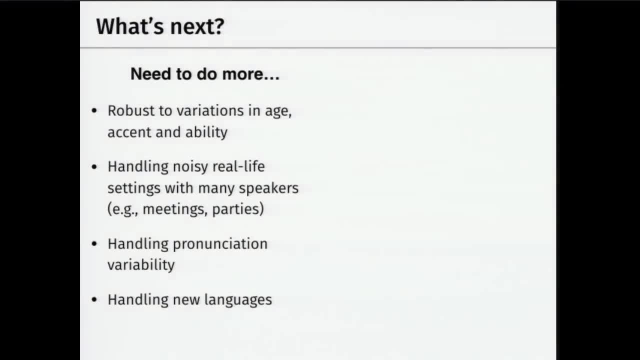 those people And this is a real, very challenging task. So how do you handle kind of noisy real-life settings with many speakers? This goes back to kind of Alan's dream of having a bot which is sitting in a meeting and kind of transcribing and 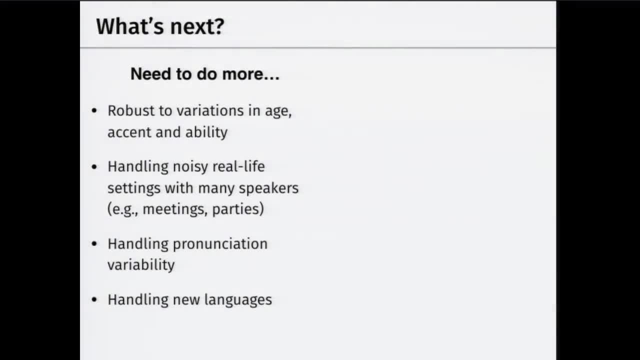 figuring out what is going on. So that would also involve the underlying ASR system in that bot would have to figure out that. okay, these are all the interfering speakers. This is the main speaker. This is the speaker. I need to kind of transcribe. 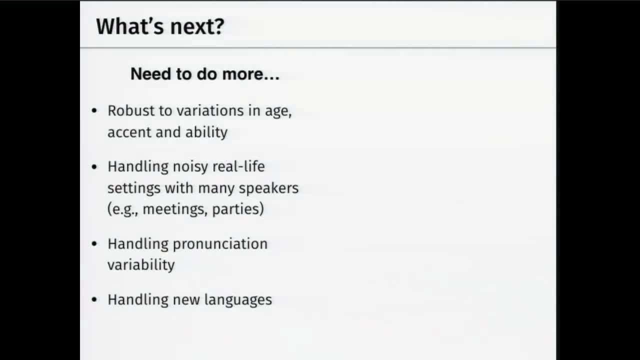 I need to haze out the other interfering speakers and so on, And this is not the state of the art for these kinds of meeting speech tasks. it's not very low. The error rates are not very low. This is actually. it's handled pretty well now. 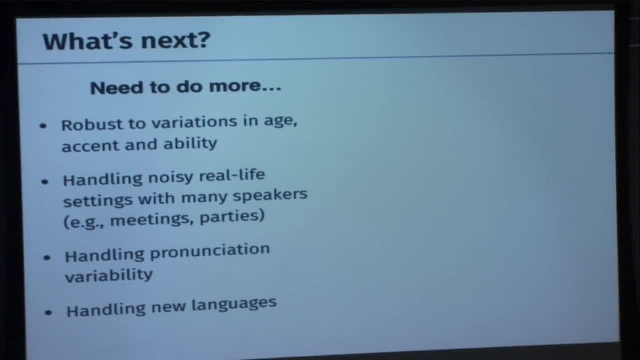 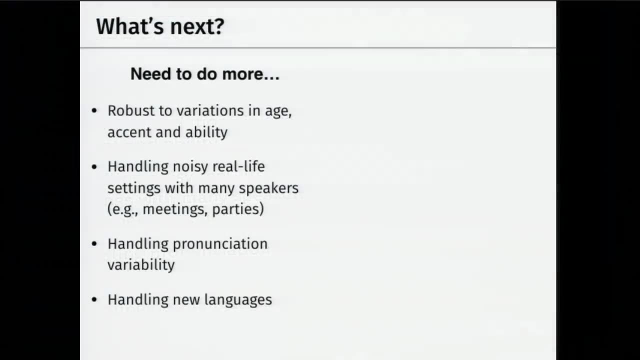 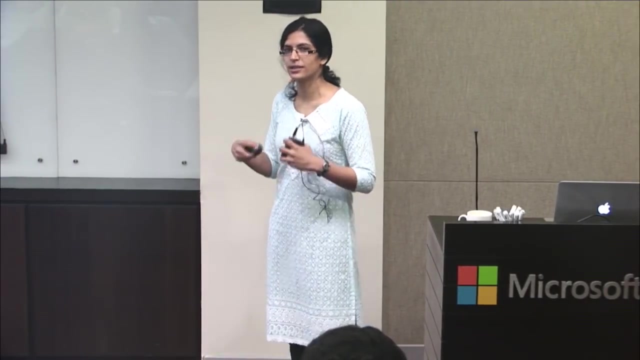 If you have lots and lots of labeled speech. this pronunciation variability is actually captured in the acoustic model itself. But handling new languages currently, I mean, the only way to do a good job is to go and collect lots and lots of data, Which, at least personally to me, is unsatisfying. 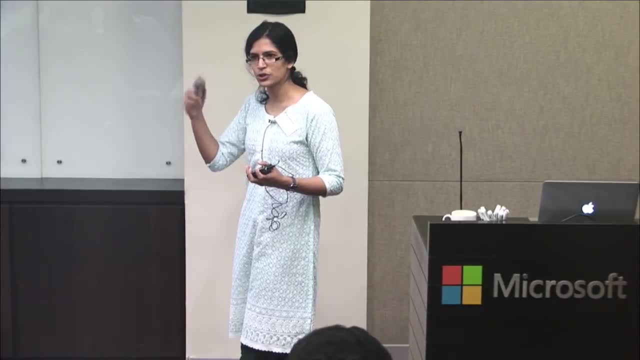 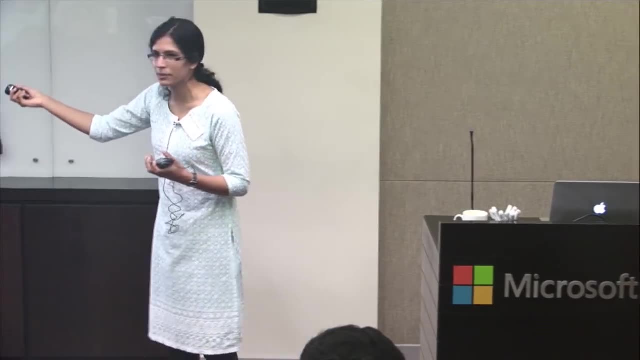 So it seems like if you have existing models, you should be able to adapt them with not bizarre amounts of labeled speech, At least if they're somewhat related. we should be able to do a half-decent job by taking existing models and adapting them to the new language. that 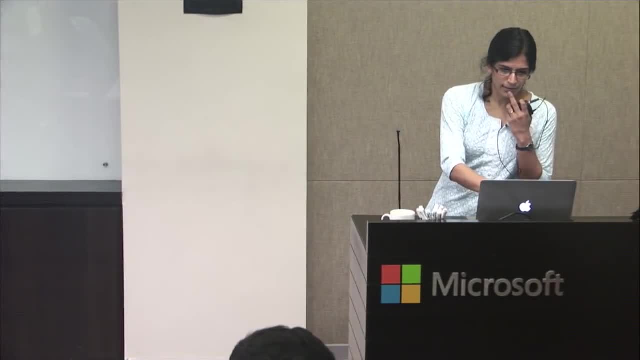 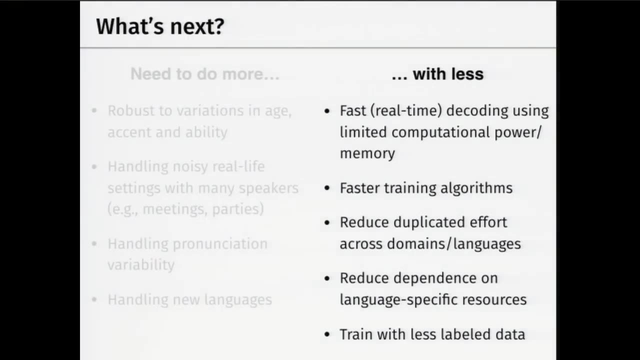 we want to recognize or the new dialect we want to recognize. So there are these problems And I think that so in computer science we are always trying to do things faster and to be more efficient, right, Both computationally and trying to do things faster from both. 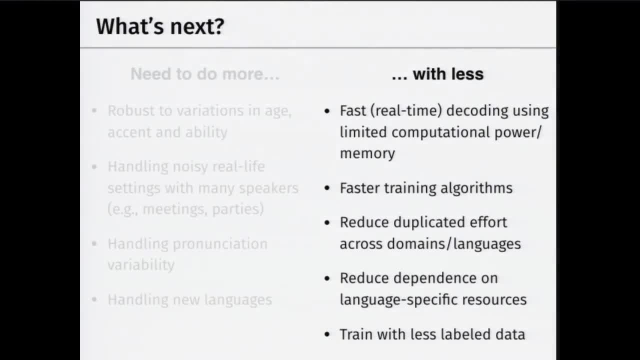 the computational power standpoint and memory standpoint. But we should also try to be resource efficient, right? We don't want to keep going and collecting more and more data every time we come up with a new task, So can we do many of these tasks with less? 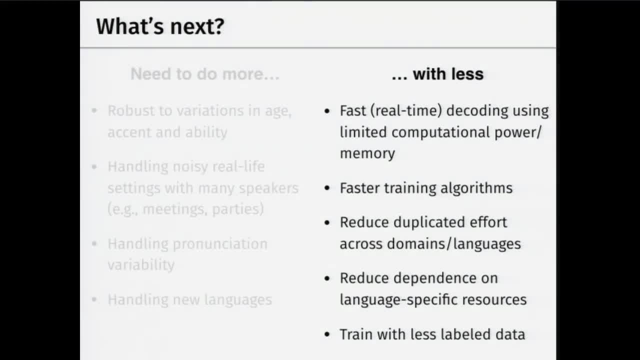 So can we kind of- this is something that I'm very interested in personally- So can we reduce duplicated effort across domains and languages, And also can we reduce dependence on language-specific resources, And this is, of course, the holy grail, I think. 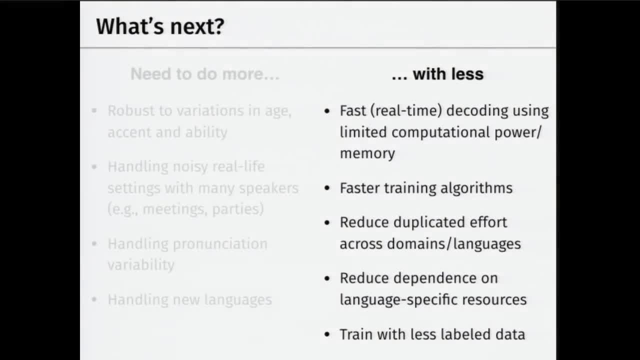 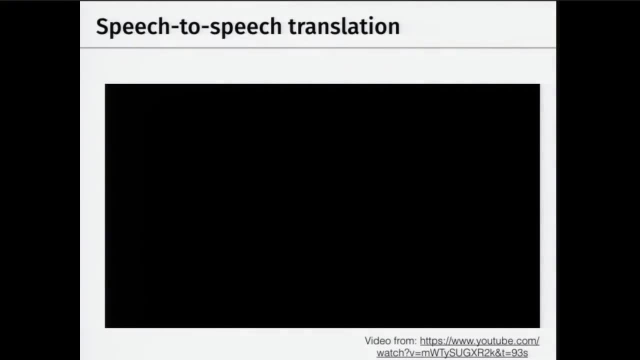 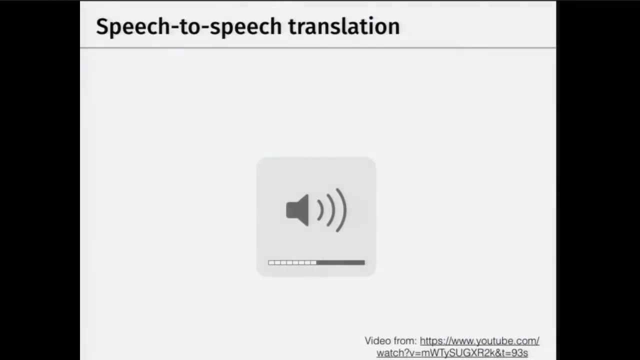 Training with less labeled data and actually making use of unlabeled data better. Okay, so I'll also show this one direction which Microsoft is working on and it's kind of very promising. So this is just an excerpt from an ad. So this is Skype. 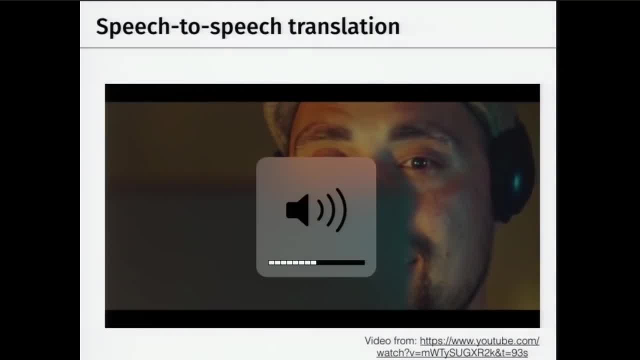 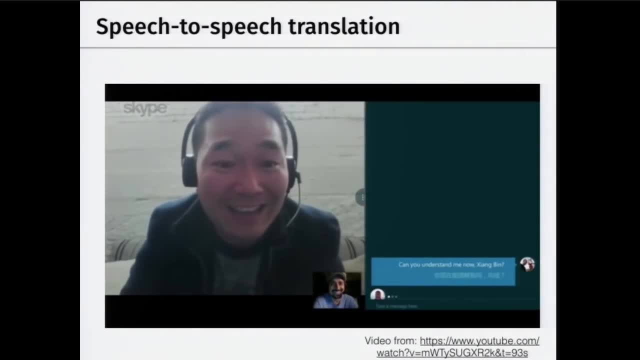 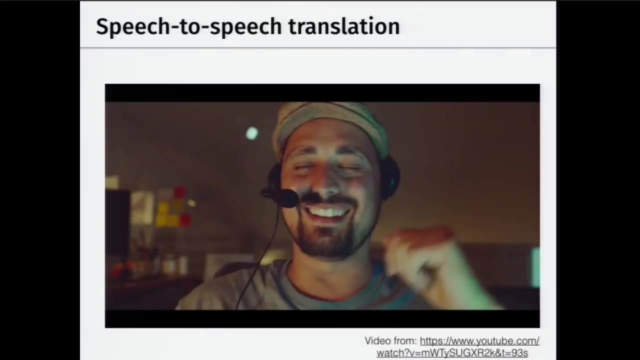 Can you understand me now, Sean, Bill? Can you understand me now, Tom? can you speak Chinese? Key, you speak Chinese. Yeah, if that worked as seamlessly as it worked here, that would be pretty cool. So I'm told this was just set up for the ad. 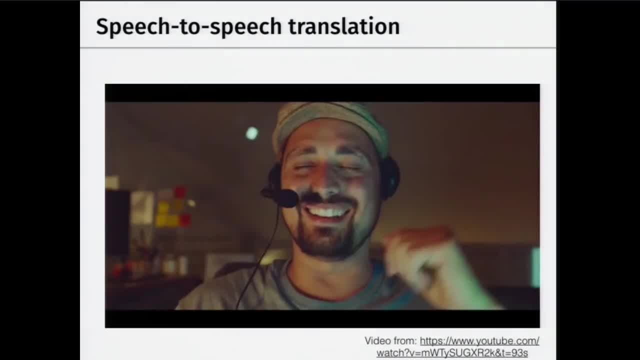 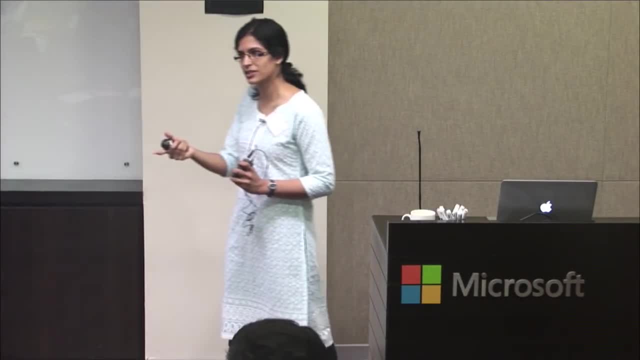 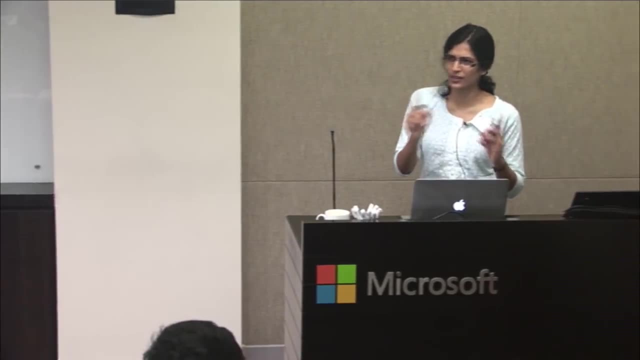 But so Microsoft has been working a lot on speech-to-speech translation and I think this is a very interesting problem Because speech also can have, there can also be cues in speech translation which help disambiguate utterances for the machine translation part, and so on. 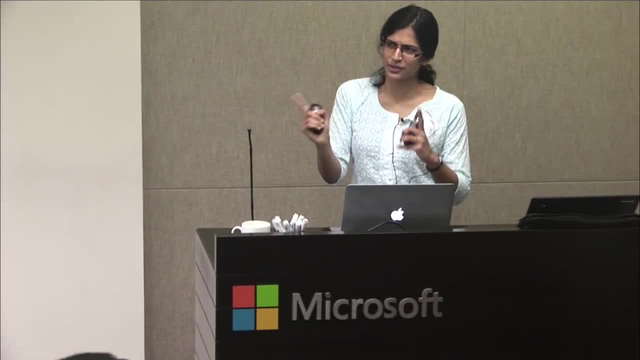 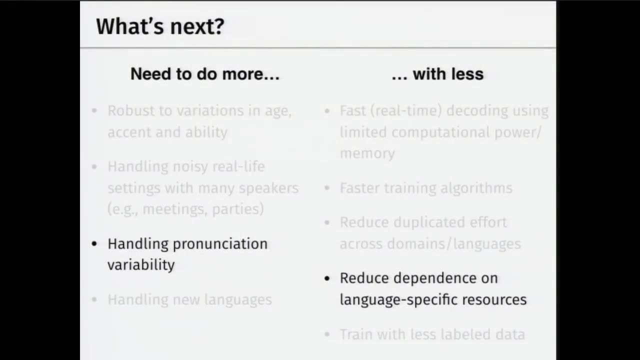 So I think there is something which can be leveraged from the speech component, from the ASR component. So this is something that we talked about a little bit, which was using speech production models and how we can build speech production inspired models to handle pronunciation. 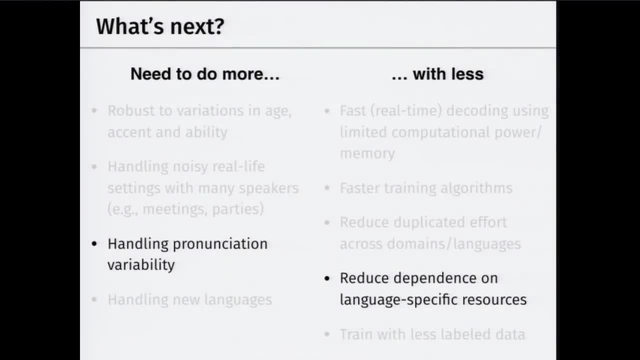 variability And actually in principle does reduce dependence on language-specific resources, Because all of us have the same vocal tract system, right. So there are only so many ways in which our different articulators can form different configurations and produce sounds. So in some sense, at least in principle, 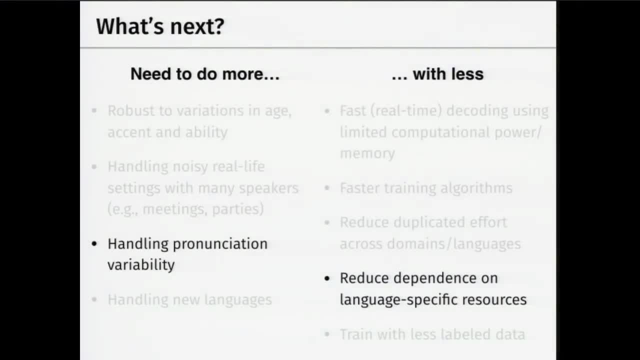 moving to that kind of a model does reduce dependence on language-specific resources, So we don't need to come up with phone sets corresponding to a particular language If you're going to represent all of these associations in terms of these articulatory features. But there are other problems with that method. 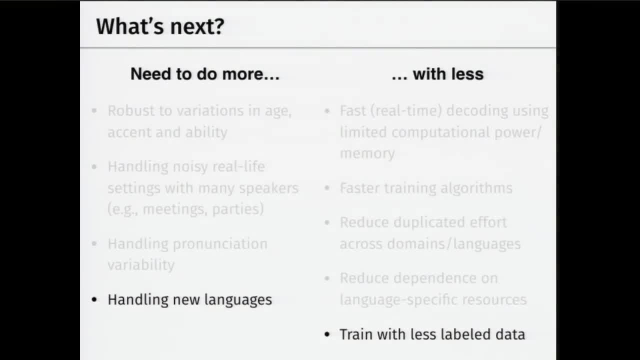 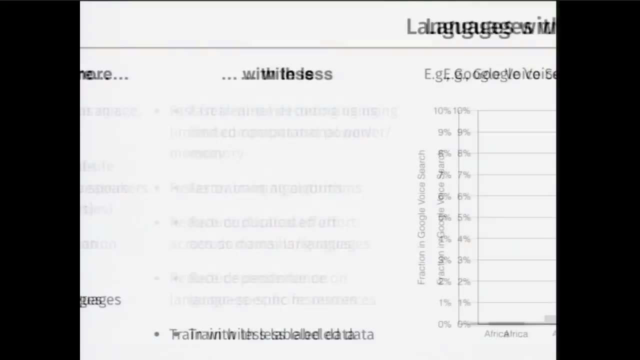 And this is another problem which I think is very interesting. So how do you handle new languages and not have to collect loads and loads of data? So just to tell you how many languages so far have ASR support, so this is actually a year or two old. 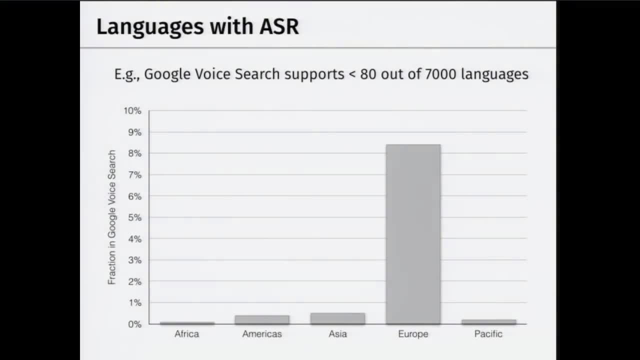 Maybe this number has gone up a little. So they support roughly around 80 languages, But these languages include Indian English, British English, which are not really languages, So that number is even lesser than 80.. And if you look at the distribution across continents, 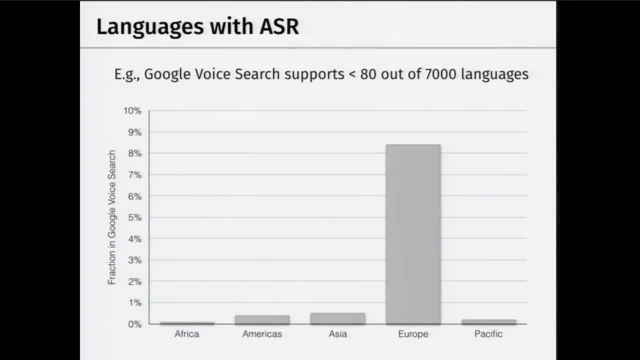 Europe has the highest representation in terms of languages which are supported by speech technologies. America, of course, is small, also because they are largely monolingual, But Asia is dismal, even though there are so many languages spoken in the Asian subcontinent. 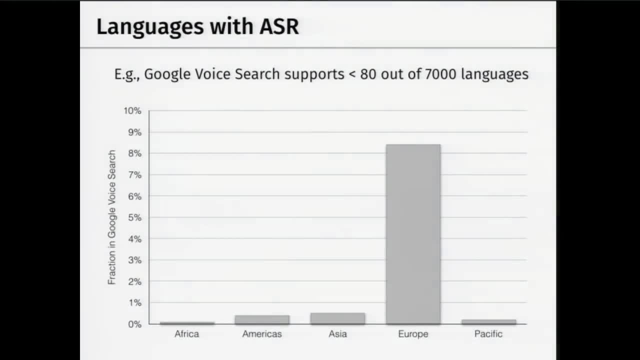 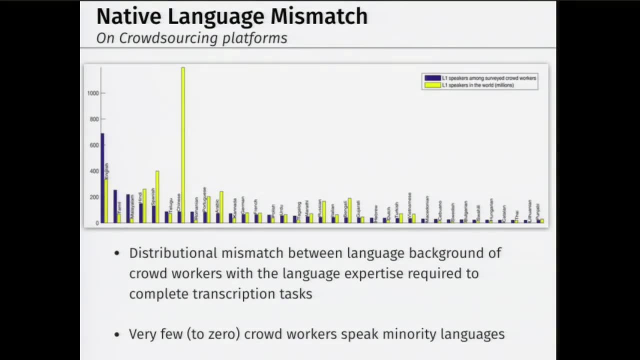 So, yeah, we should all do more to build speech recognition technologies or language technologies for various Indian languages and languages in Asia, And so one thing that we have looked at is: can we try and crowdsource the labels for speech? So can we just place speech utterances to crowds who? 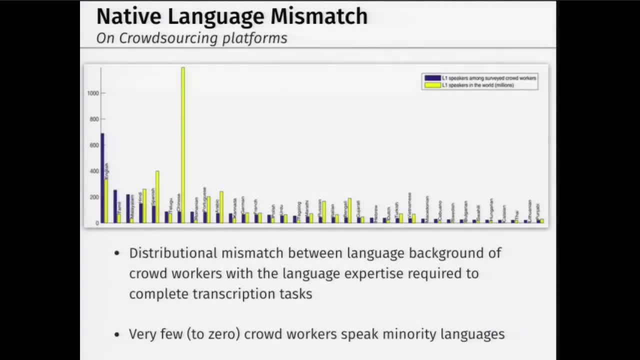 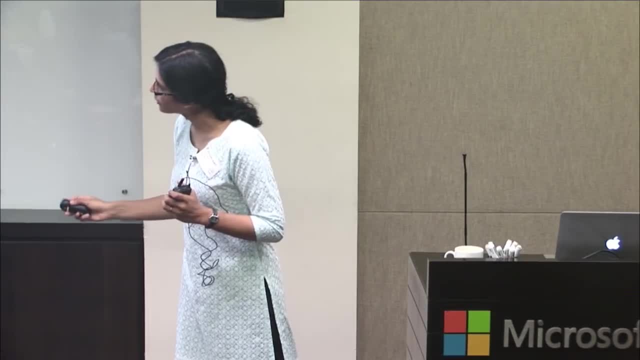 speak the particular language and then try to get transcription from them. So it will be a little noisy. but then there are techniques to handle the noise in those transcriptions. But that also has an issue because it's somewhat unfair to a large number of languages. 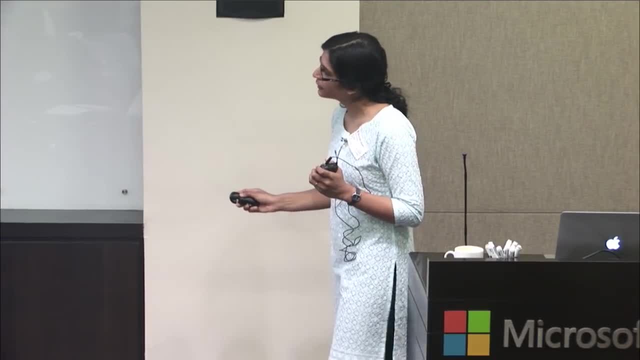 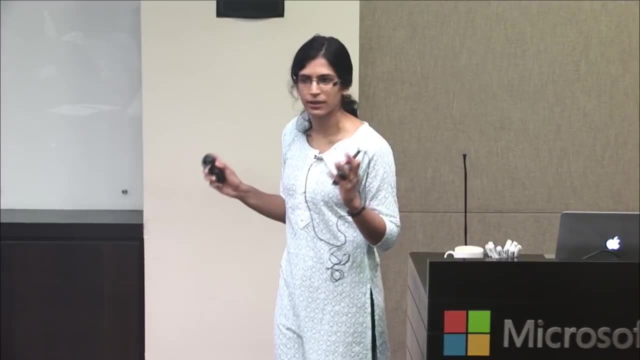 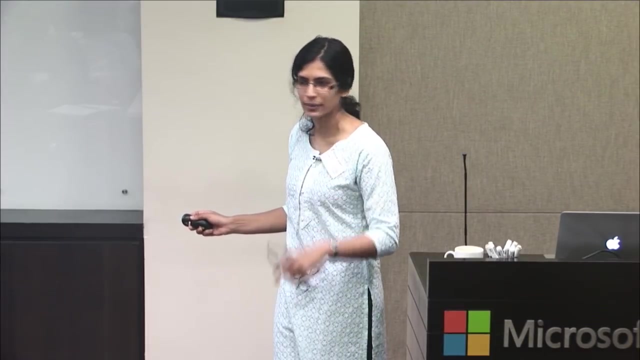 So this is just a histogram showing this was all the speakers who are sampled from a large crowdsourcing platform which is MTurk, Amazon's Mechanical Turk, And this looked at the language demographic of crowd workers on Mechanical Turk And the yellow bars are actually the speakers of those languages. 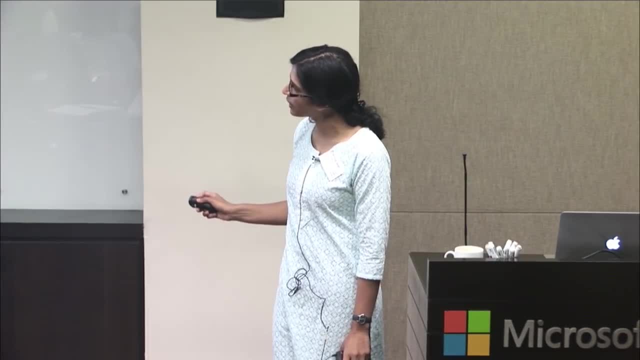 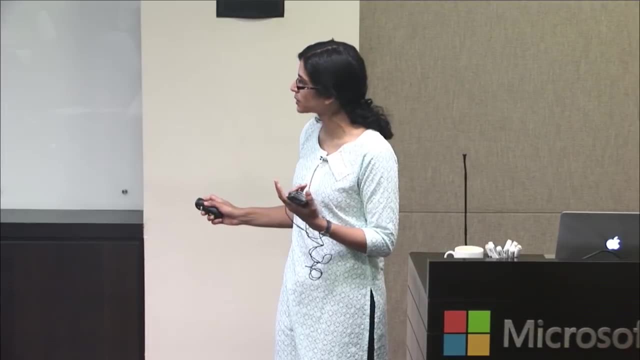 In the world. So you can see there's a large distributional mismatch between the language background of the crowd workers and the language expertise which is needed to complete transcription tasks. And if you look at, I mean, this tale is really really long. 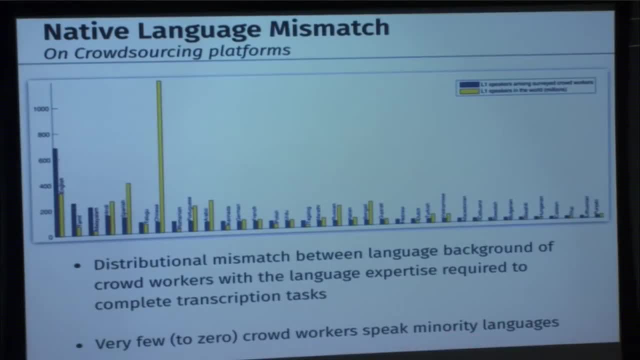 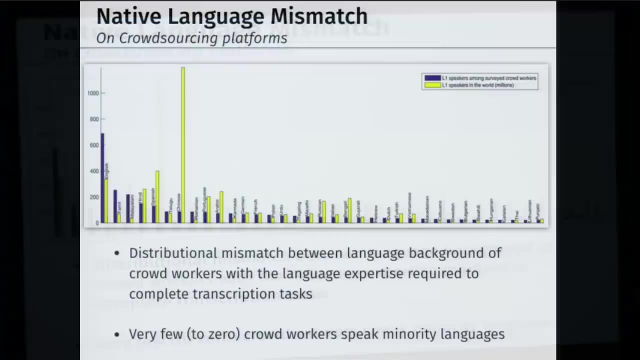 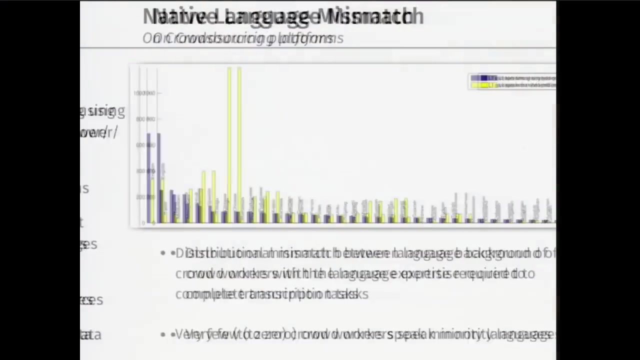 So forget about minority languages or languages which it's very, very hard to get native speakers on crowdsourcing platforms. So this also may not really be a viable solution always. So I think there are lots of interesting solutions, lots of interesting problems to think of in that space. 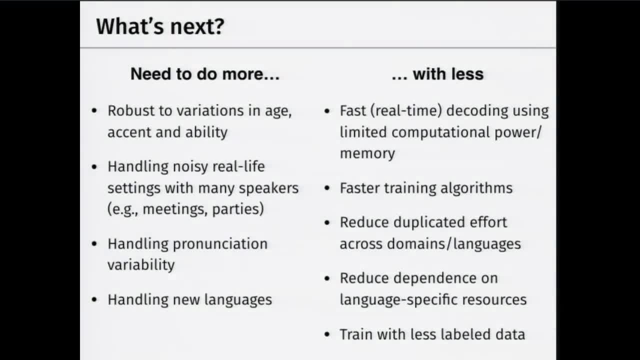 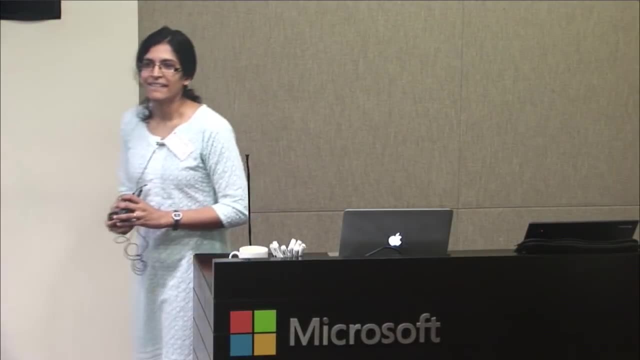 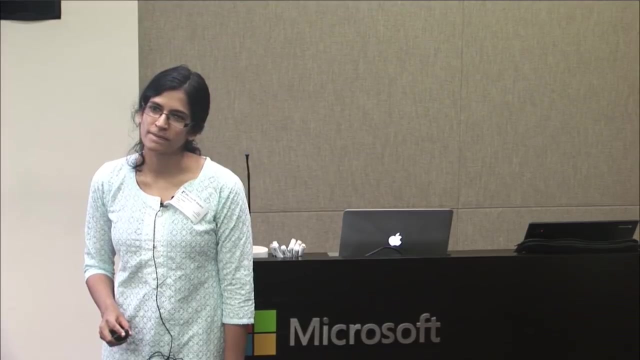 So with that I'm going to stop. I'll kind of leave you with this slide. Yeah, I think I'm doing good on time. So thanks a lot. I'm happy to take more questions. Yes, Yeah, Yeah, so in language models. 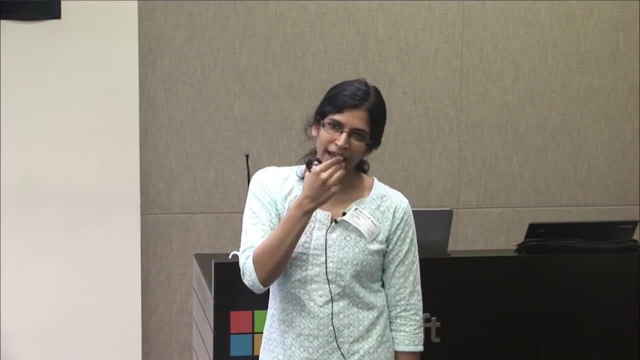 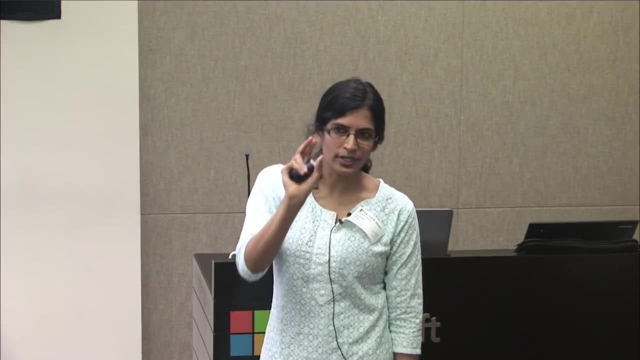 you can back off all the way to a unigram model. So as long as each of the individual words you've seen somewhere in the language model And if your acoustic model is good, so it's going to give you a somewhat reasonable phone. 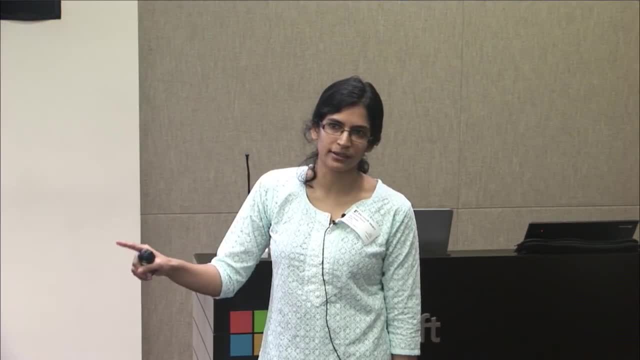 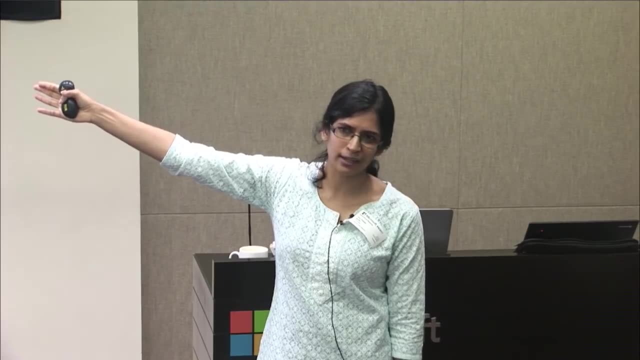 sequence corresponding to the underlying speech. You might still recover the word sequence, even though the language model doesn't give you too many constraints. So, for example, I think, with Sarah Palin's speech, the language model- I don't think anything more than maybe a bi-gram model. 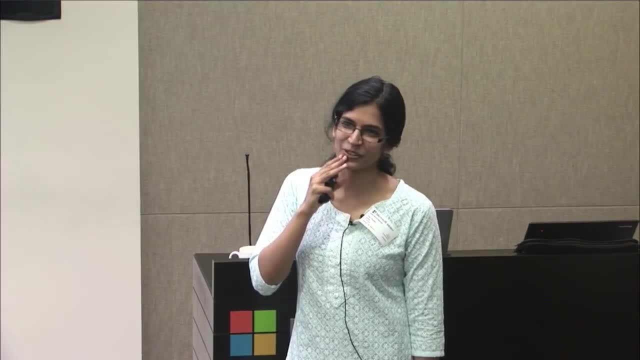 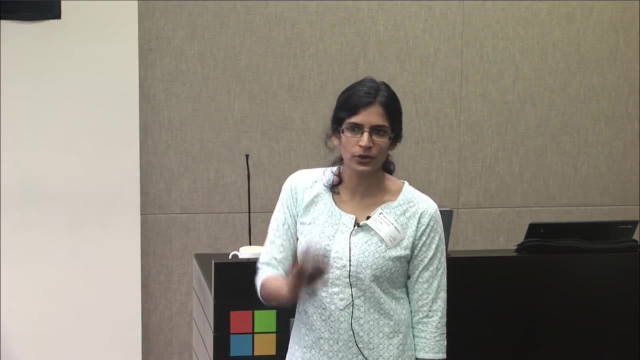 or maybe a tri-gram model at the most. So as long as the individual words have been seen in text, in large volumes of text, and if your acoustic model is good, you can still recover it, even if there is no continuity between the words. 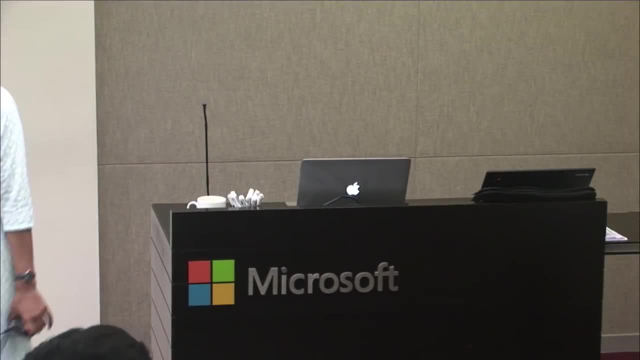 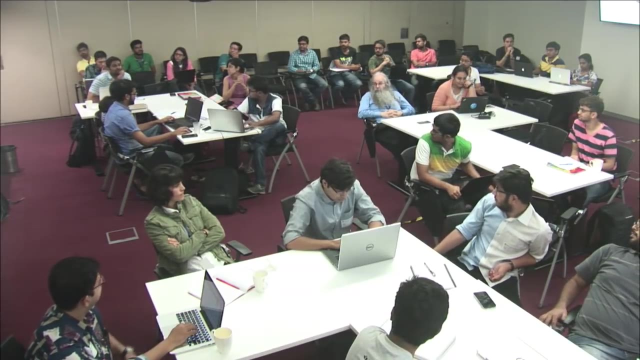 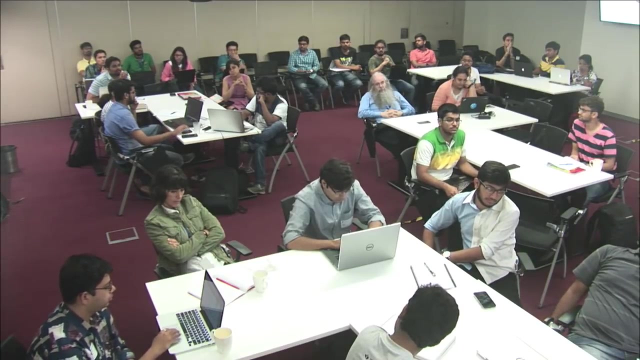 Does that answer your question? Yeah, Any other? Okay, yes, Do you ever feel a need to have more than 40 phones, for example in English? Because I thought that's probably the case. Did you ever find some peak somewhere which you felt that? 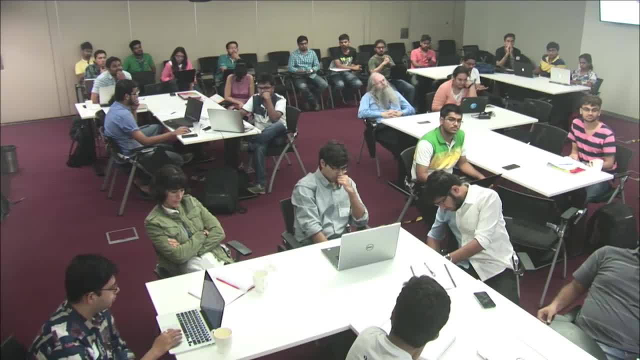 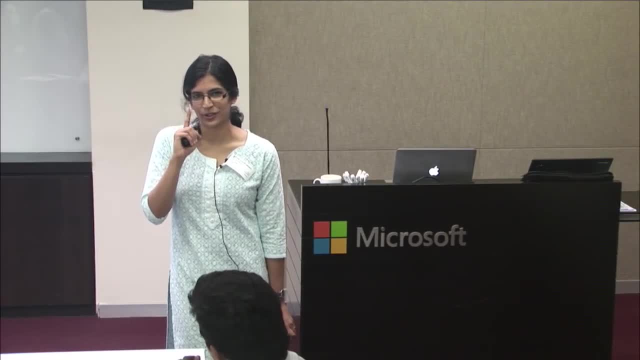 having more than 40 phones would probably help the system. Would it help to have more than 40 phones? Actually, the so 40 is the number of phonemes. Yeah, but so the number of phones in English is more than 40.. 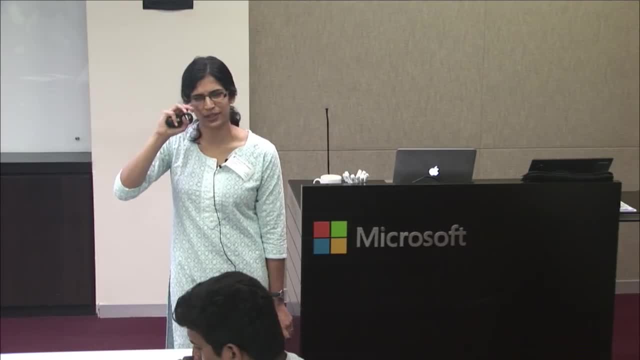 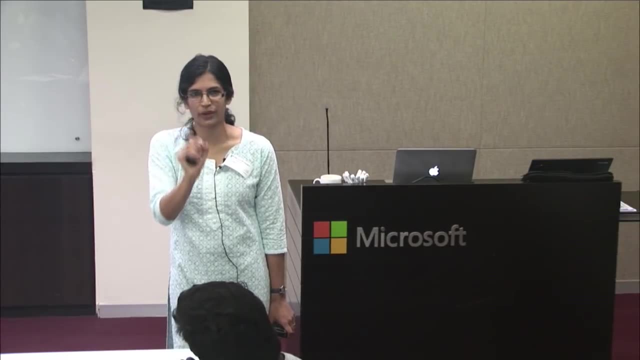 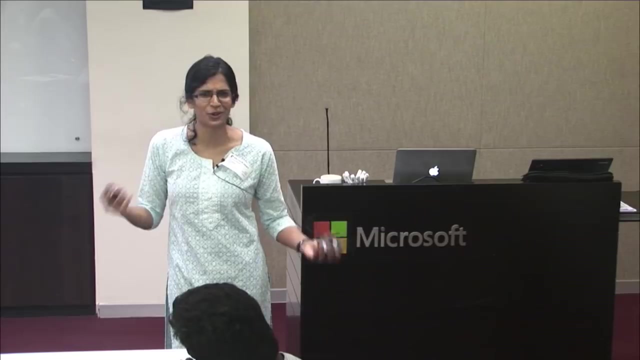 So even in those phonetic transcriptions the number of phones were almost close to 80.. Because it's actually annotating all the fine-grained variations And that of course helps if you have that kind of but where are you ever going to get that level of phonetic annotation? 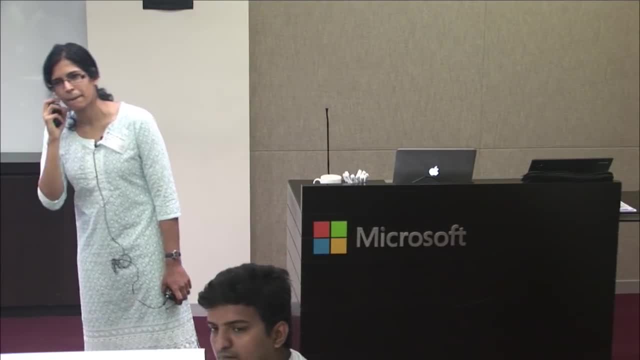 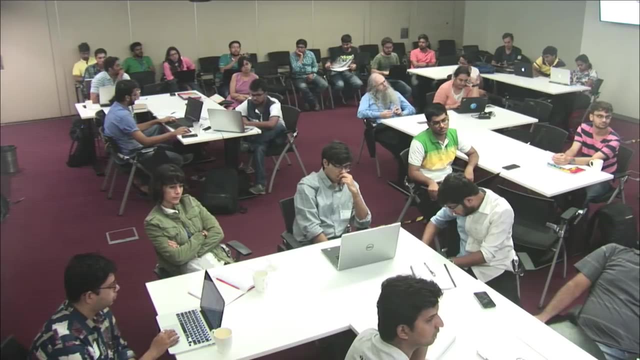 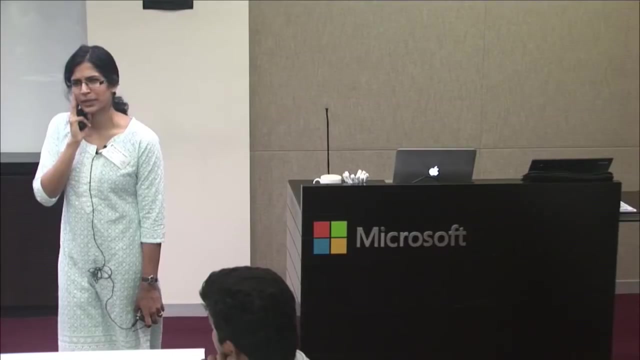 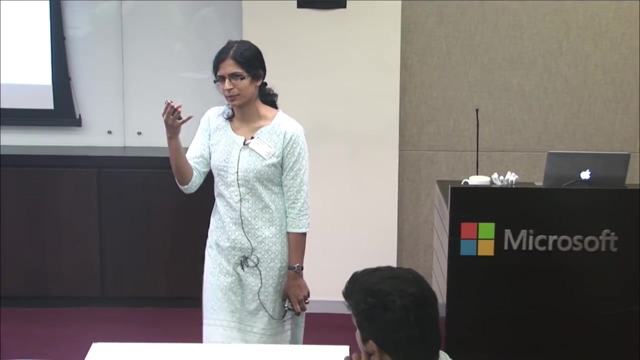 Yeah, You need lots other than lots of data Other than Indian. you also need lots of computational resources. So, but other than that, like I said, it doesn't really work as well as the entire pipeline yet. So there's still a delta in terms of the performance of the state. 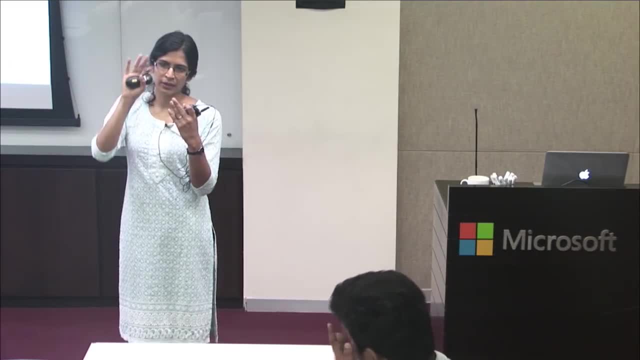 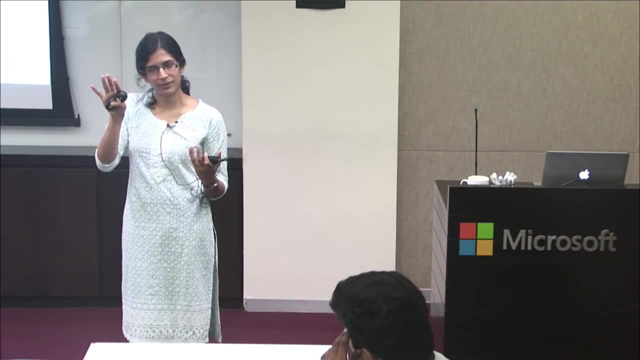 of the art systems. There are systems and these end-to-end systems, And also so currently so all these end-to-end systems are recurrent neural networks. So there is this issue of how much context to retain and whether you're retaining that context effectively. 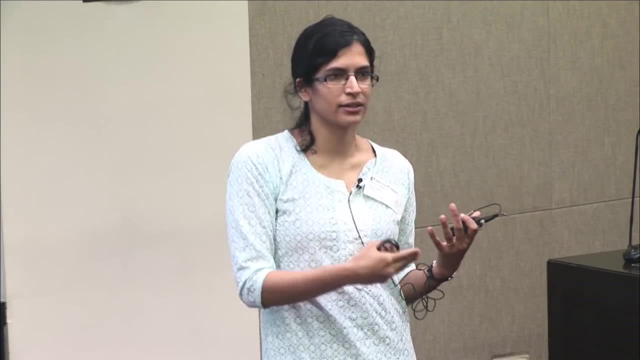 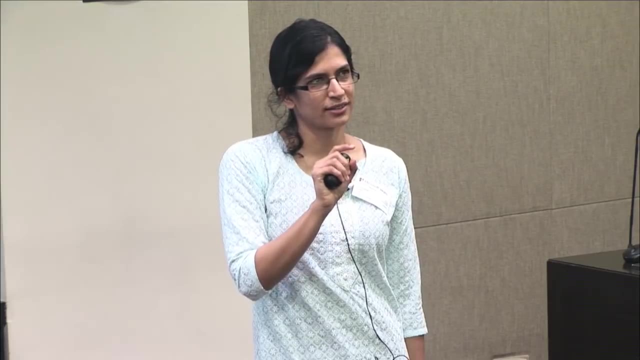 which is where these attention mechanisms come in. But attention mechanisms also really fall short. So, if you're interested, there is an ICLR paper this year which is- I think the title is something like frustratingly short context Or something like that. 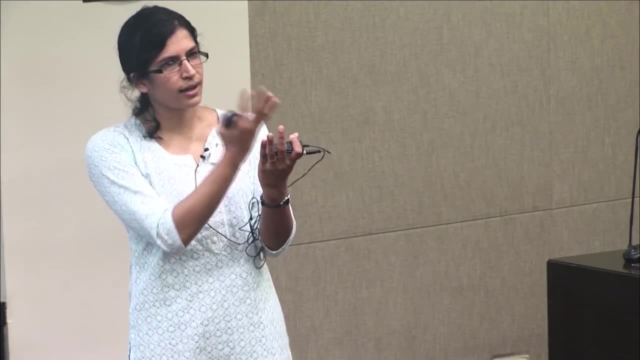 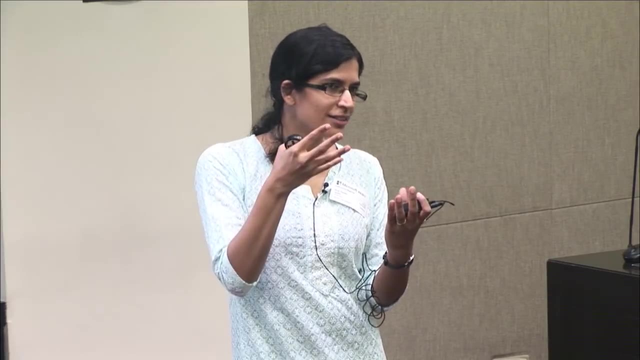 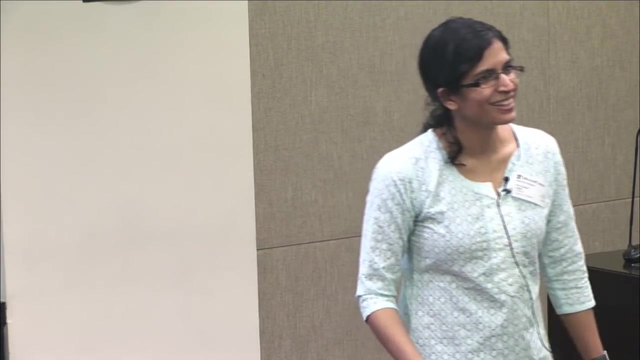 You can search for frustrating. So the idea is that even if you just look at the last five output representations, you can do as well as a really sophisticated attention mechanism. So attention mechanisms also need to be kind of improved further. Yeah, How does these end-to-end systems work for? 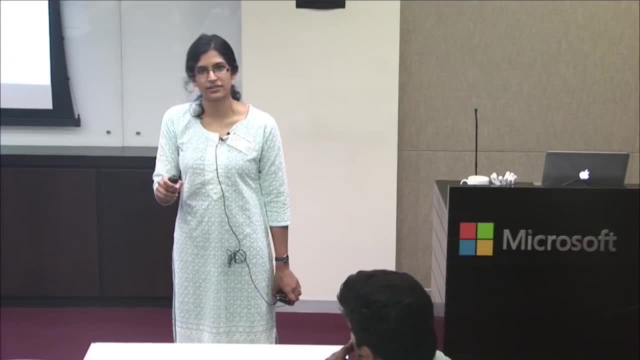 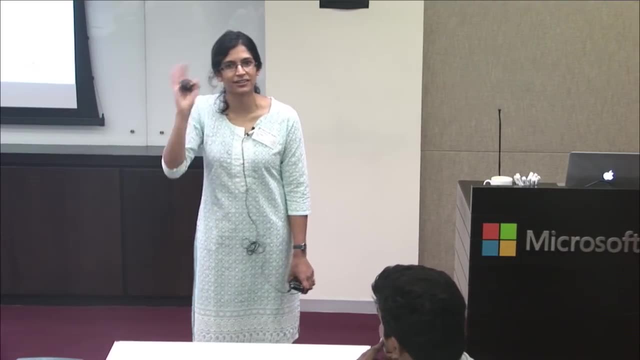 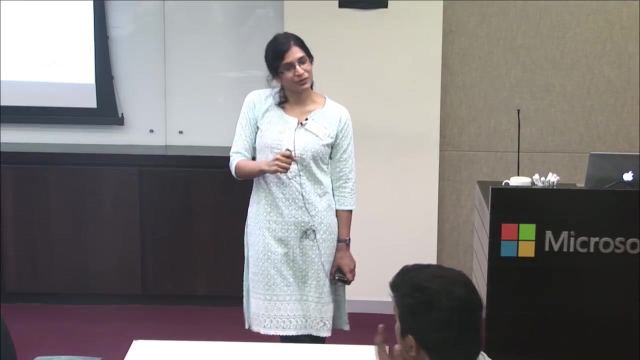 Yeah, so the end-to-end system is actually predicting characters, So it predicts a single letter of the alphabet. So out of vocabulary is not an issue at all because it's predicting one character at a time. So it might then work even better for Indian languages. 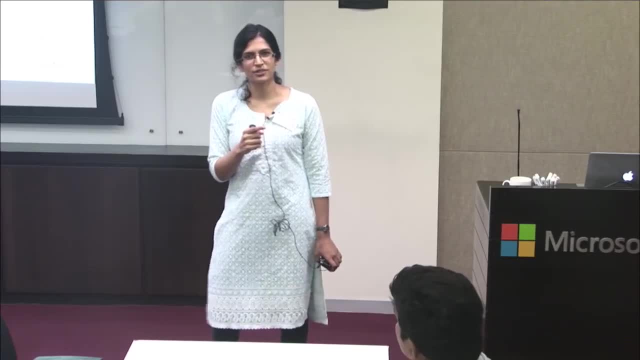 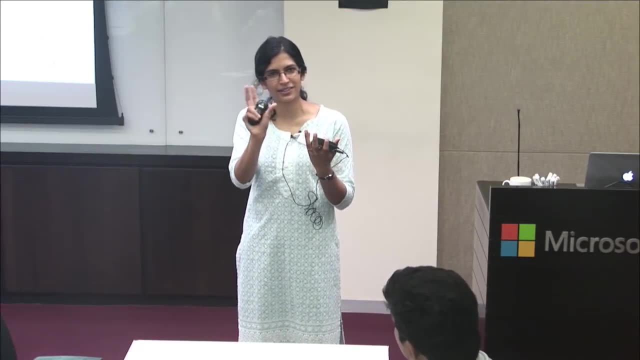 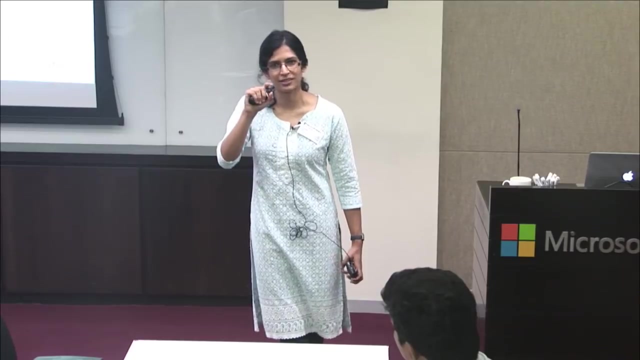 Yeah, so that's actually something very interesting. So for Indian languages, which are morphologically rich and where you probably cannot expect to see various forms of a word in the vocabulary, end-to-end models might actually work really well, But we haven't seen this yet, because this amount of data is 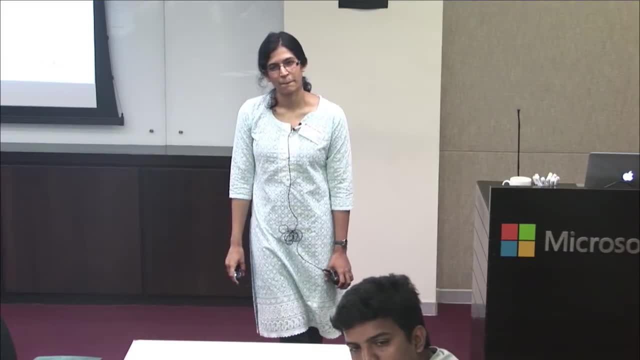 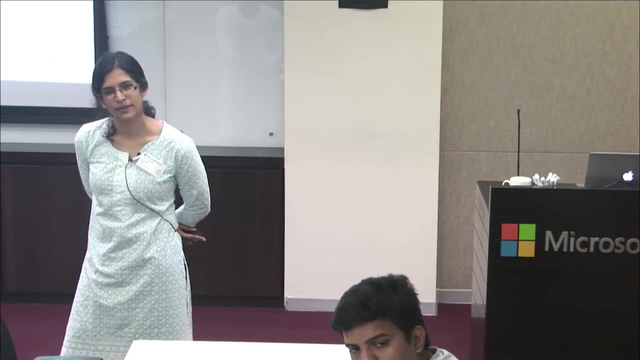 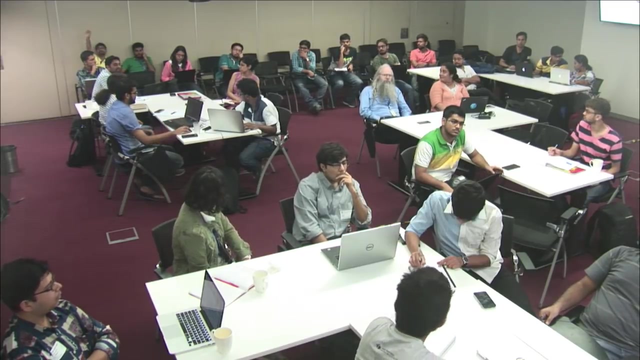 not available. yeah, Yeah, Yeah, For end-to-end speech, for example, in English, you have a 26 characters to map. Yeah, but that's a good mark. In English, right, characters don't really map to sounds. 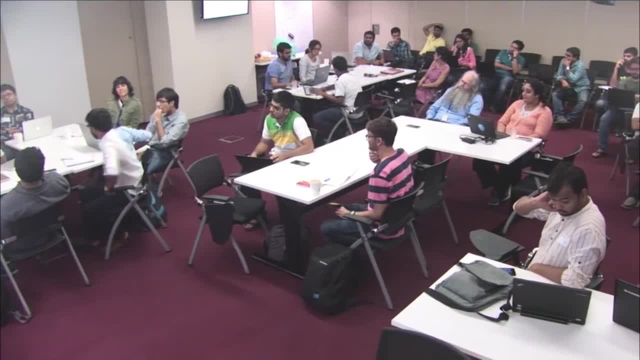 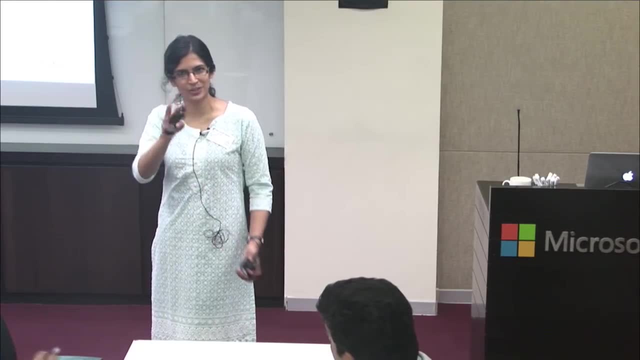 No, not at all. So the end-to-end system actually needs to all these problems. it needs to learn. It needs to learn the sound mapping, It needs to learn the spelling. So yeah, so there's no, because it's so irregular, right. 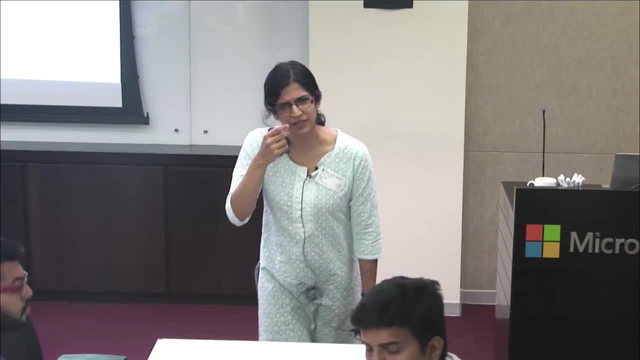 the mapping between the characters. So what was the point you were saying, Sunil? So I mean like, for example, in English it's like 26 classes. Yeah, I mean, that's what you're dealing with. 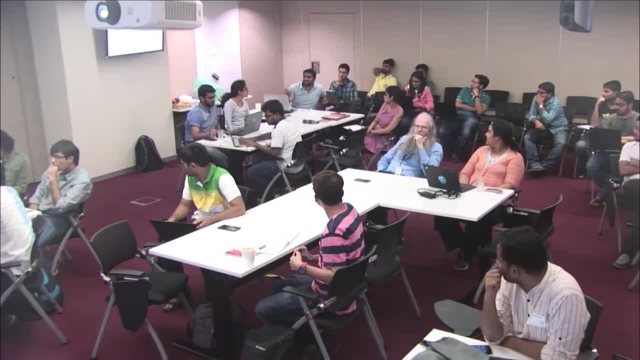 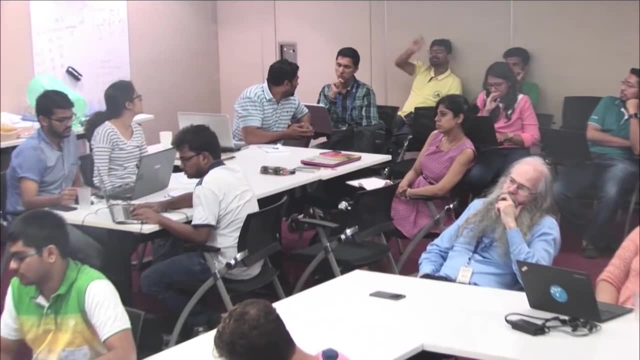 But if I take Hindi, for example, I need to have a class for and C, right, So you have so many combinations of-. No, you don't need a class for and C, You have E. Yeah, exactly Yeah. 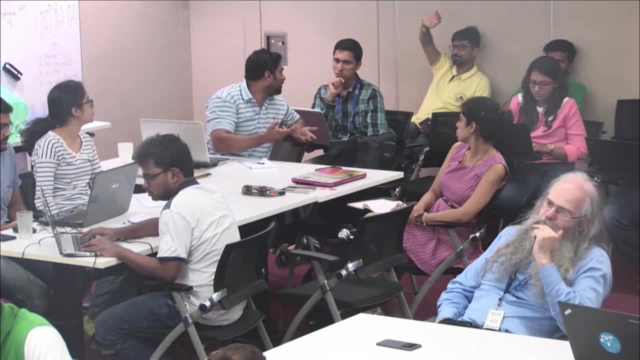 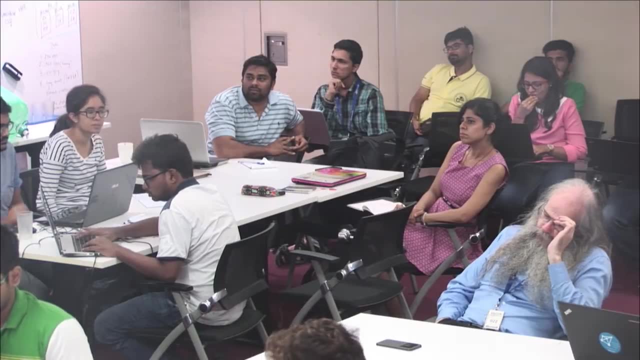 So you just- 50.. So you have multi-levels for every- No, you might have double of 26, because you, so you have one. so you just split it as split it according to its Unicode representation: Right. 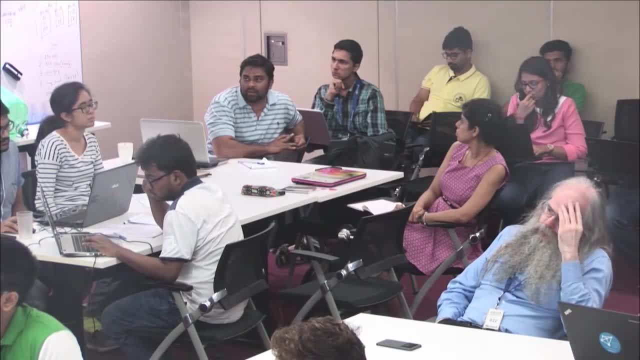 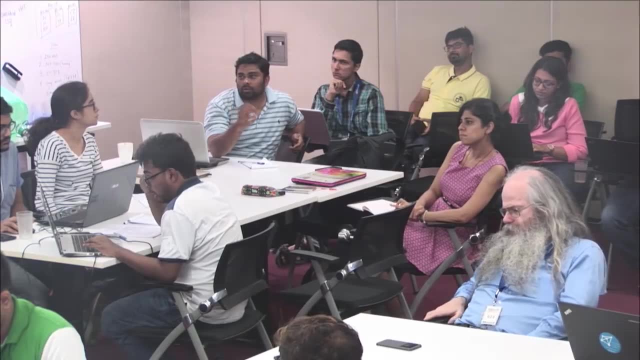 So you would have: C would just be sub plus E, the E matra. Okay, So you would predict sub and then you would predict the matra and you would predict and so on. So it would be multi-level or not a single level. 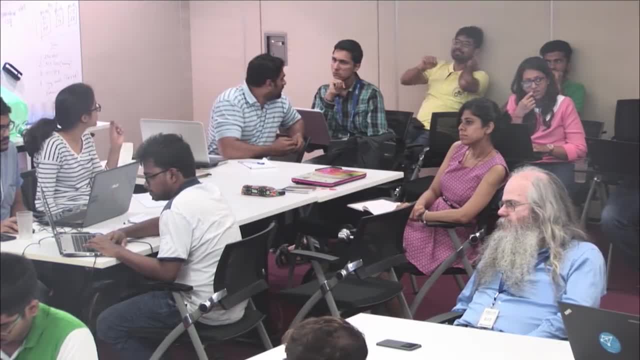 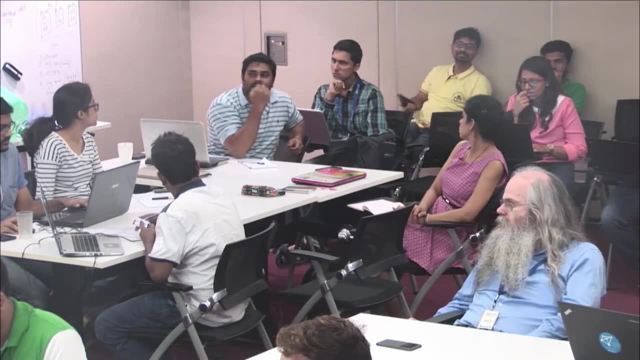 No, it's not multi-level, So you just predict each of these. So you see, on English, S, E, let's say So, you predict S, then E, then- Yeah. So here also you predict the- Yeah, yeah. But the label size? of course the label space becomes larger, but probably just by double. I don't think it'll be more than that, Which, if you have enough data, should be okay. And I think yeah, because the like Monojit said: 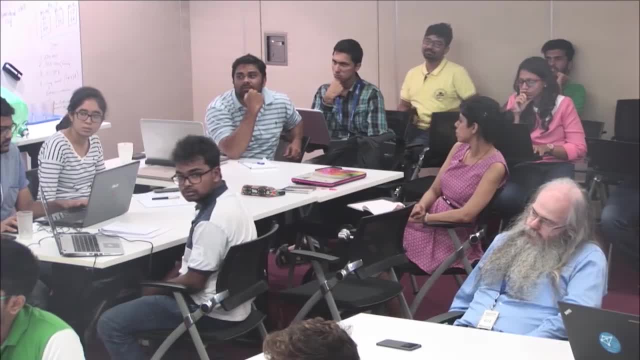 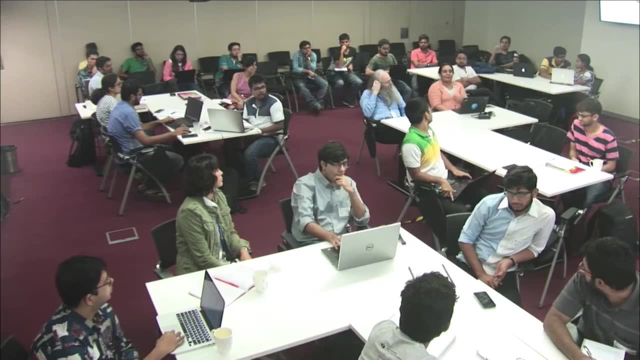 the mapping is much more stable. It actually might do even better than in English. Yeah, What do you think the minimum amount of data is that we need if we want to? Yeah, so I asked this to friends at Google and so on. 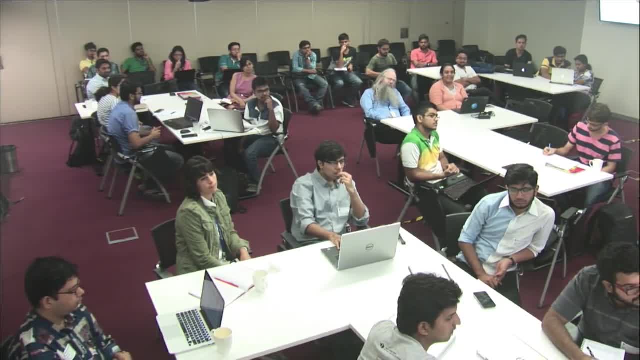 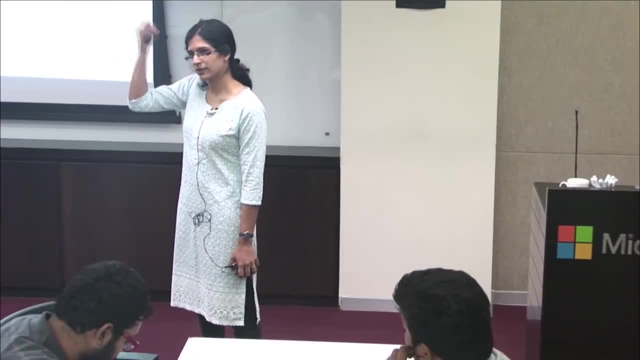 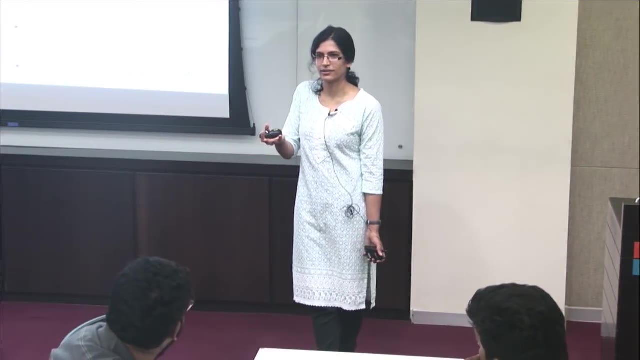 So they use like $10,000 of speech. All of you must be using speech of that order, So I know the standard pipeline. so for switchboard for instance. So switchboard is around 200 hours of speech And the error rates now are like 5%. 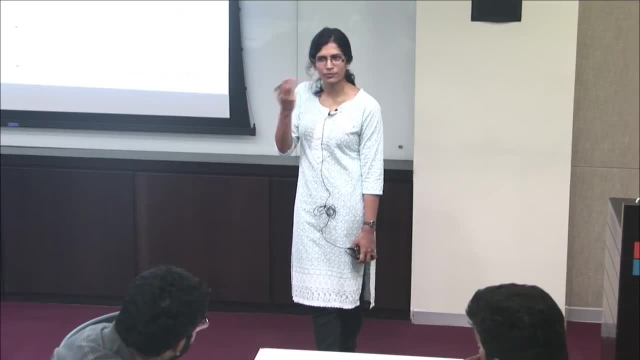 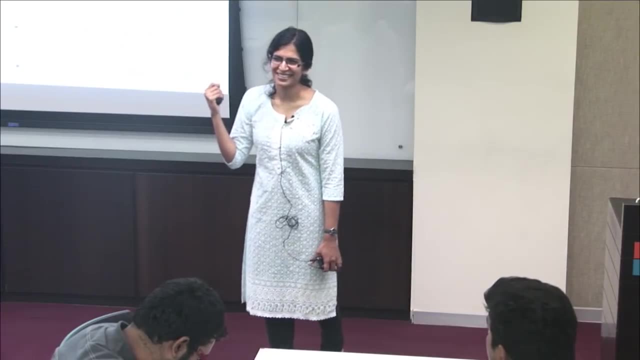 The latest was 5%. Okay, So, of course, with a lot of machinery. so Yeah, end to end. What do you think the minimum, bare minimum, would be if we really wanted to do this, To try it out? 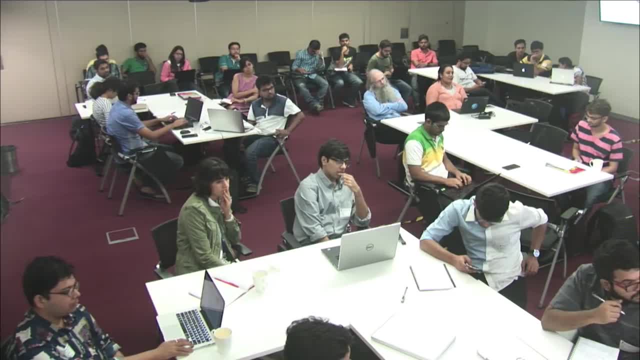 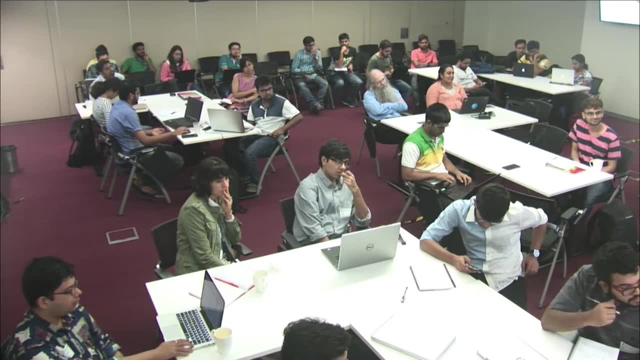 So the other papers that I showed you, they actually work with switchboard, which is 200 hours of speech. So even if you're in the 100 hours and more, I think you can start trying out end-to-end systems. But if you're looking at 10 hours, 20 hours I think. 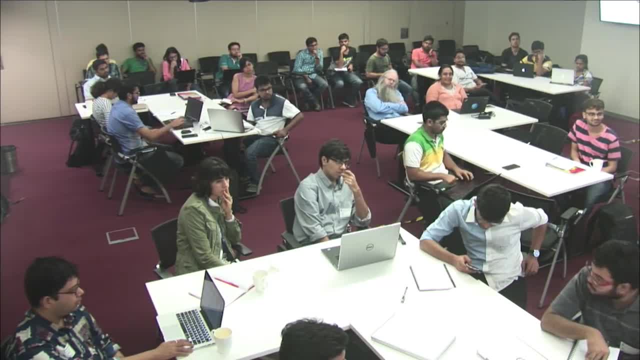 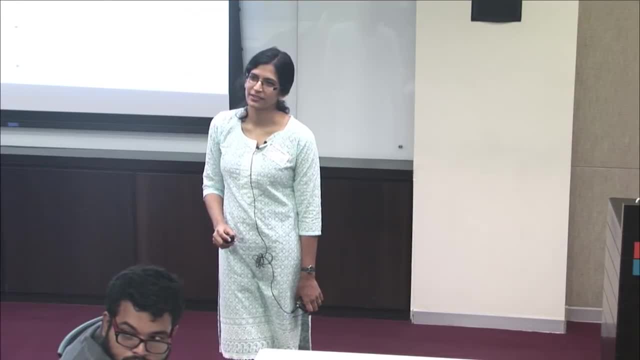 but I would still be interested to see if there are experiments on Indian languages with even smaller amounts of data. Right, right, 120 hours, Correct, Yeah, yeah, So it's sort of beginning to work, isn't it? Yeah? 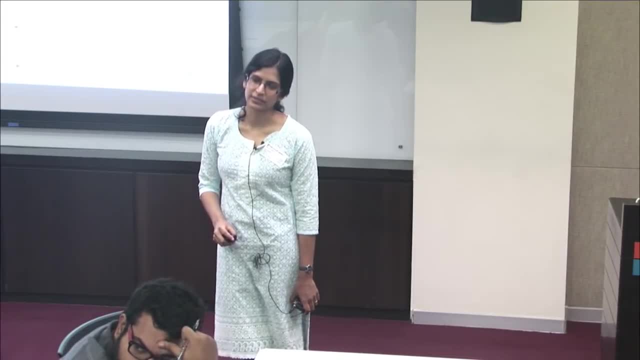 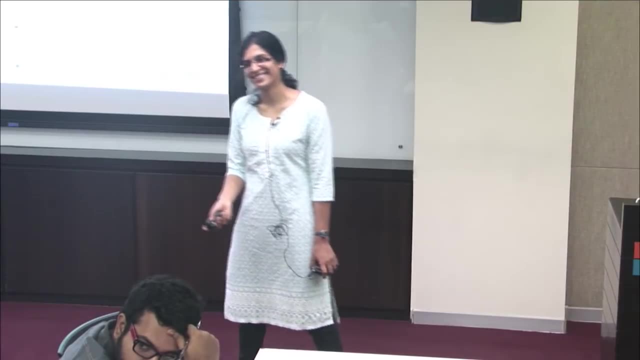 It really has to be appropriately similar data. Yes, So if it was all lectures from one person, then maybe- Yes, yes, yes, That's true, that's true, Of course. yeah, But you probably need good transcriptions. 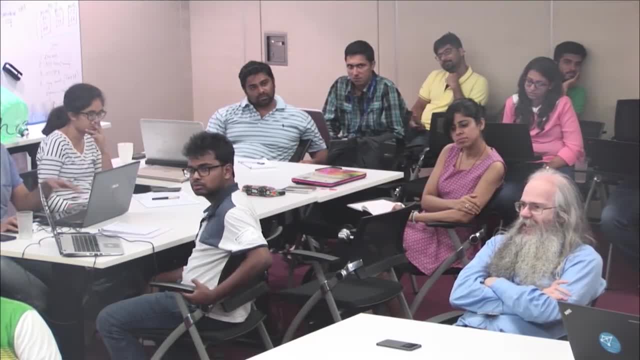 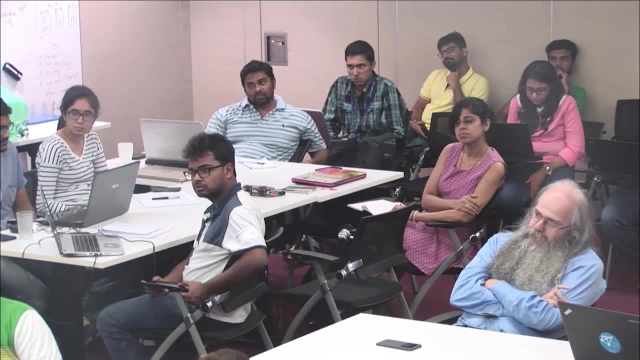 but don't underestimate that If you were doing it for Hindi, you know like is- Yeah, I think- Yeah, That's a very- I think that would be a really good experiment to run, even with just 10 or 20 hours of Hindi speech. 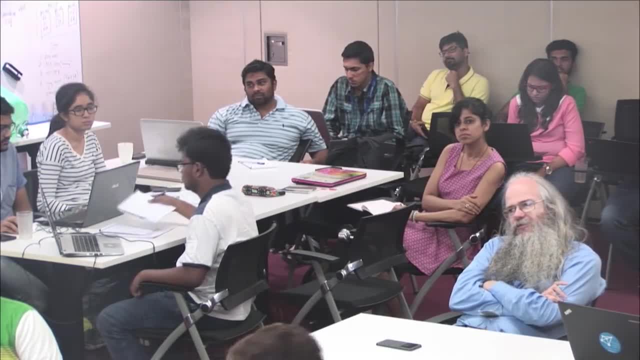 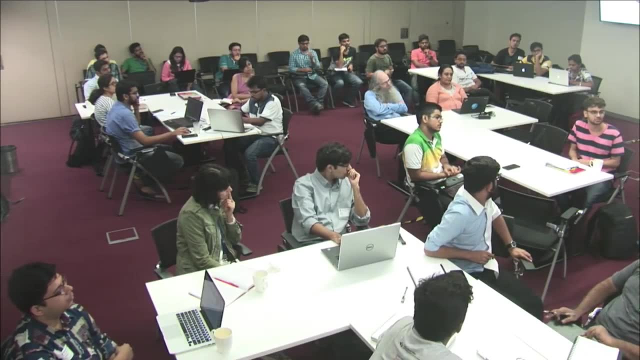 Yes, How an end-to-end system would perform. Yeah, You had a question. Yeah, Is there evidence of these end-to-end systems performing better for a language with less complicated or- No one has done that yet. Not just Indian languages, any languages? 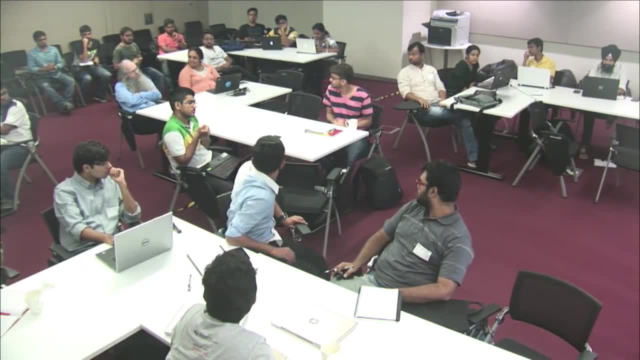 Oh no, So I'm not familiar. No, no, no, No, no, no, no, I'm trying to think about that. Alan, you had some- I'm trying to think about that. I'm trying to think about that.